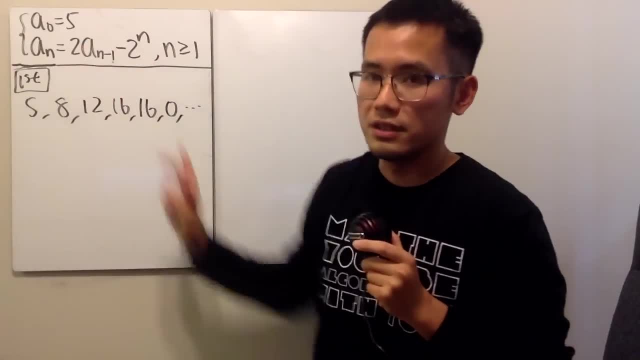 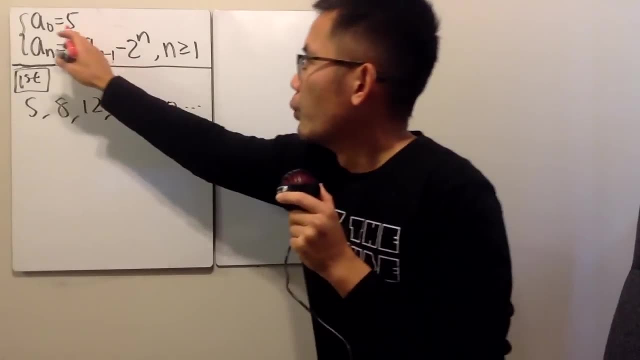 And notice this right here- does not base on the previous term, And usually when you have 2 to the nth power, it's a good hint that we should be looking at the powers of 2.. Well, n starts with 0, so I will write down this right here. 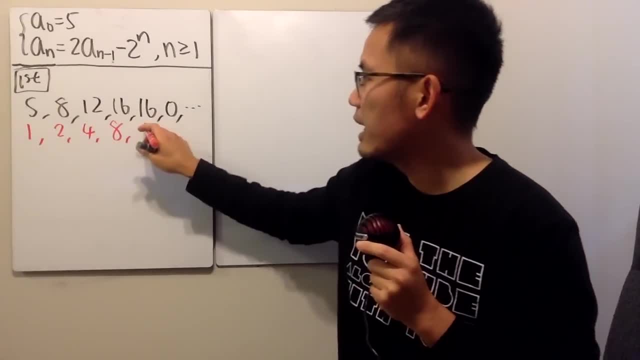 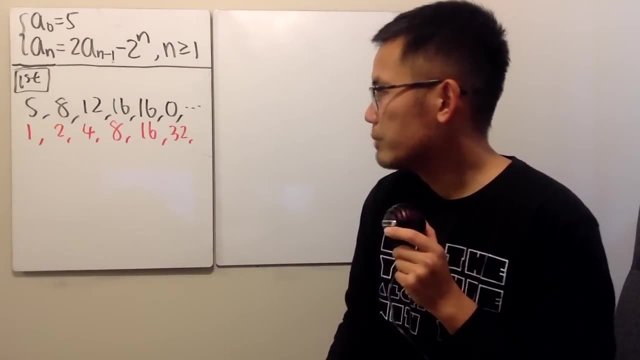 1, and then 2,, and then 4,, and then 8,, and then 16, and then 32,, and then so on, so on, so on, right, Very nice. Now I want to make a connection between these numbers and these. 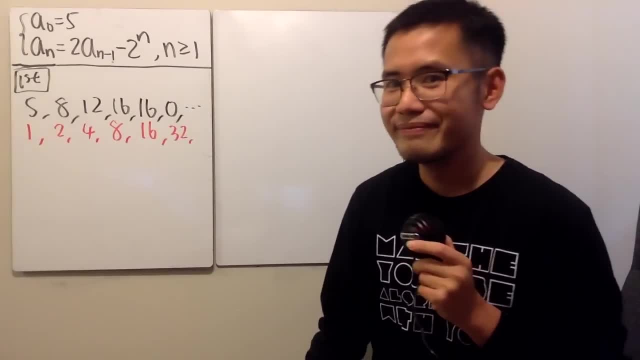 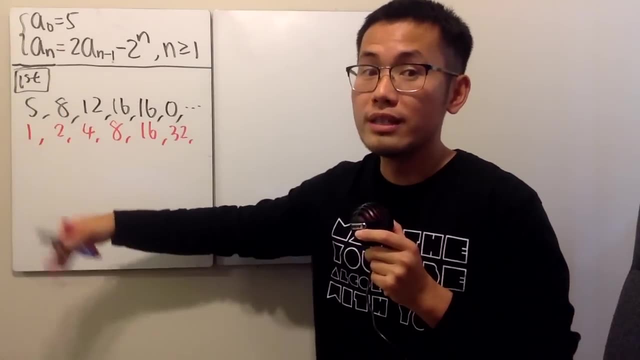 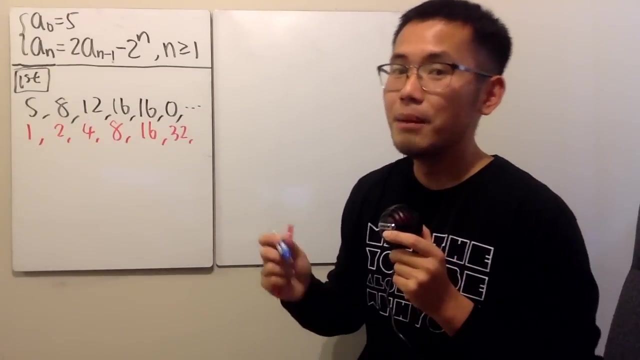 How can we do it? Well, have a look. How can we go from 1 to 5? You can say add 4, or you can say multiply by 5.. How can we go from 2 to 8? You can say add 6,, but, better yet, you can say multiply by 4.. 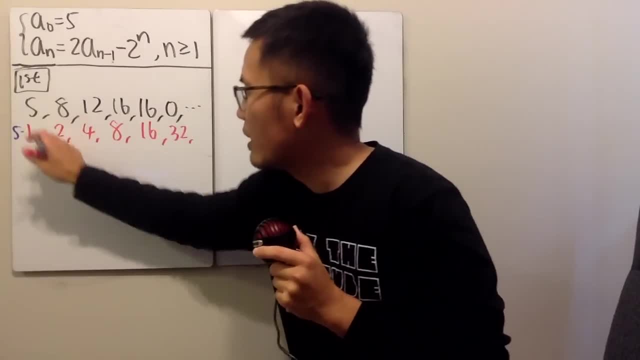 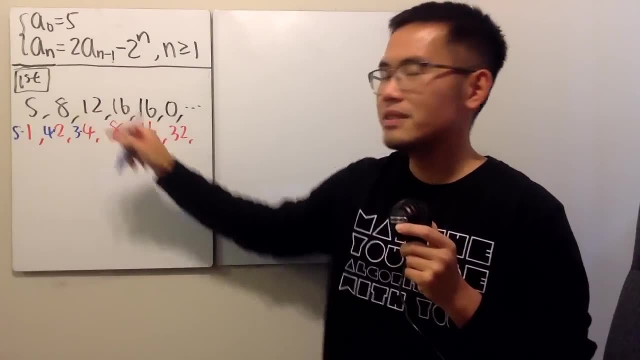 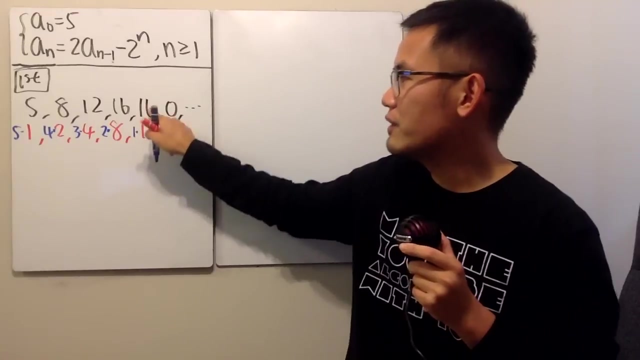 Because if you said: multiply by 5 here and then multiply by 4 here, what's next? Multiply by 3.. Multiply by 3, isn't it? 3 times 4 gives us 12, and then 2 times 8 will give us 16, and then 1 times 16 will give us 16, and lastly, 0 times 16 will give us. 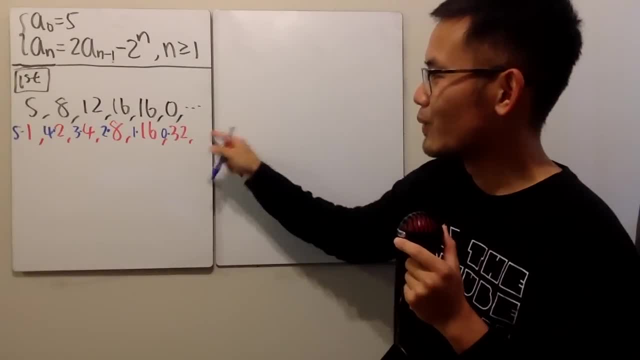 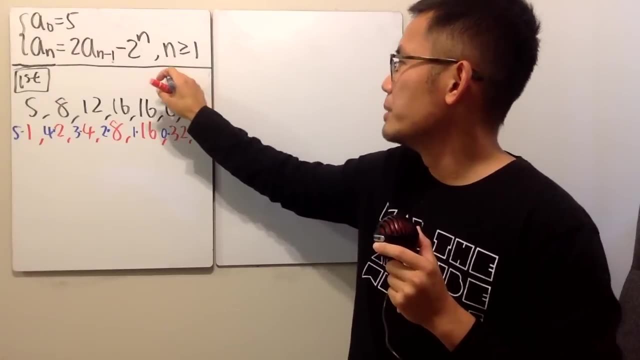 I mean 0 times 32 will give us 0. What's next? It will just be negative 1 times 64,, isn't it? So here again, it will be negative 1 times 64. So that will be negative 64 for the next number. 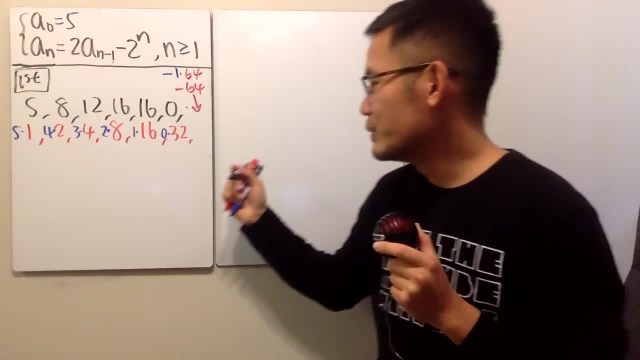 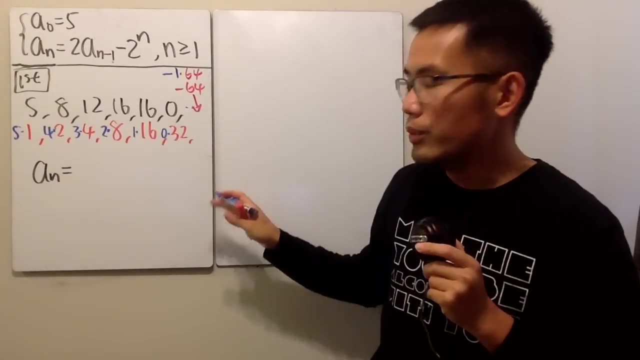 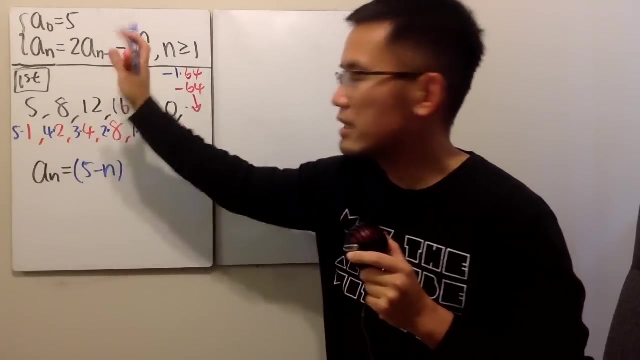 Very nice, huh. So based on this we can just write down a formula already: a, n is equal to the following: The numbers in blue they're just going down, It's arithmetic, That's very nice. And the formula for that is just 5 minus n, because n starts with 0.. 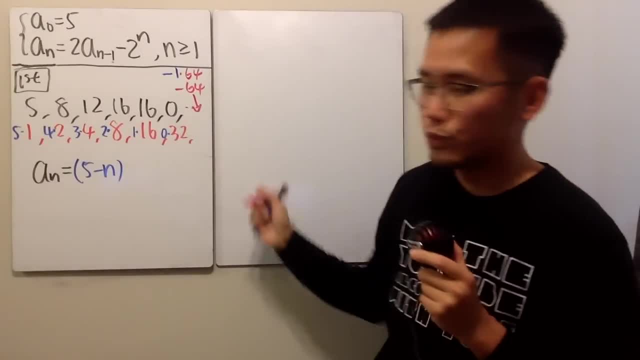 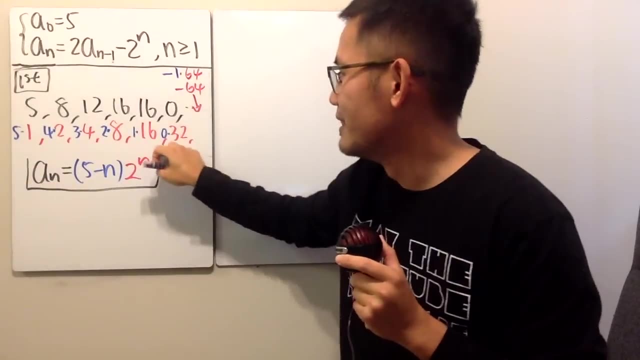 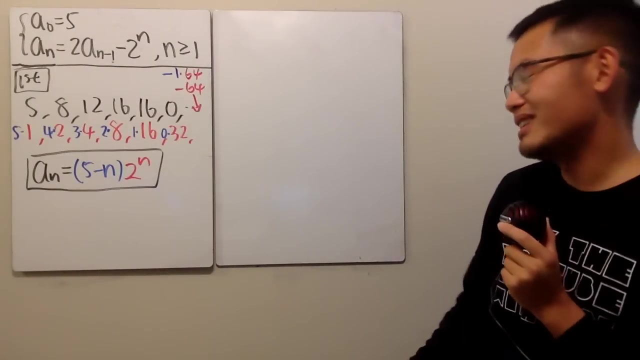 Then we see that the numbers in red, they are just the powers of 2.. So I just have to do 2 to the nth power And we are done Again. as I said this right here, It could be the one that you love the most, or it can be the one that you hate the most. 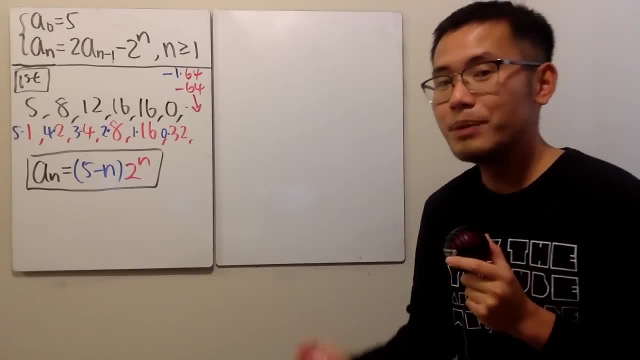 Sometimes it's not so easy because, for example, if you look at the Fibonacci sequence, write it down. Write down the numbers 1, 1,, 2,, 3,, 5, 8, so on, so on, so on. 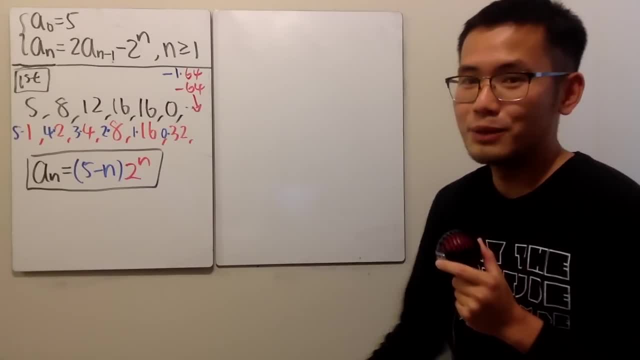 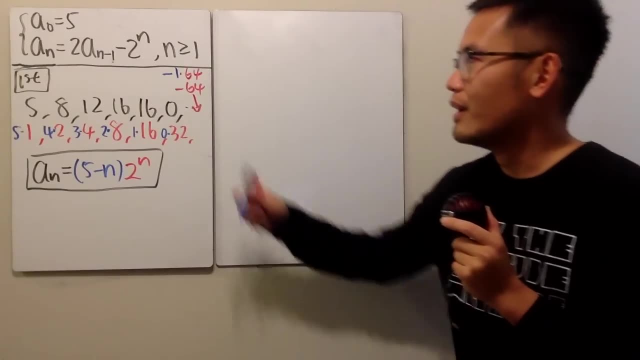 And try your really best and see if you can find a nice pattern for that. Can you come up with an explicit formula for that? I don't think so. Right, You do have to have a systematic way in order to solve this kind of recursions. 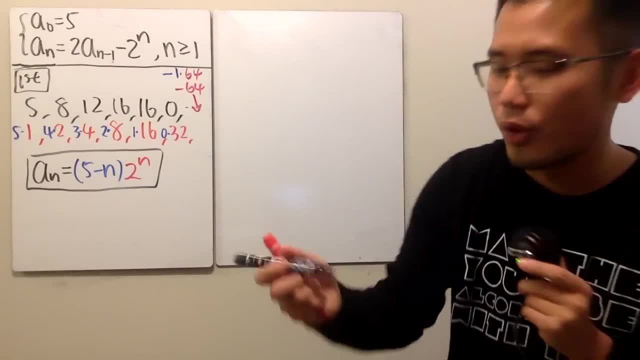 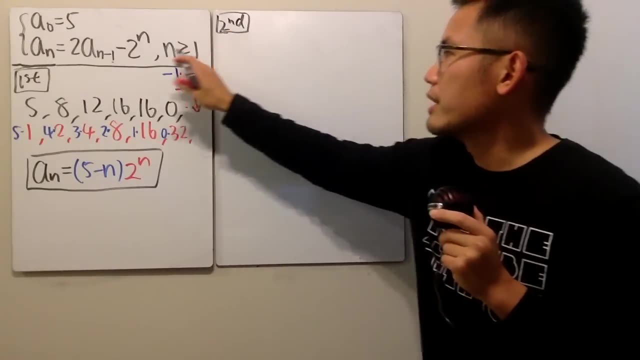 And that's the second way, And also the third way are four, So have a look. Here is the second way. Well, as I mentioned, this right here is called the recurrence relation, And some people also call this to be the recursion. 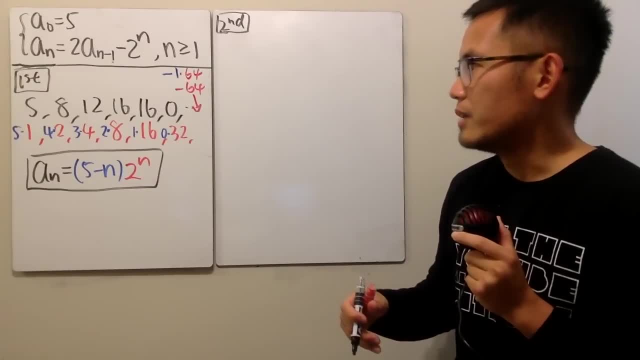 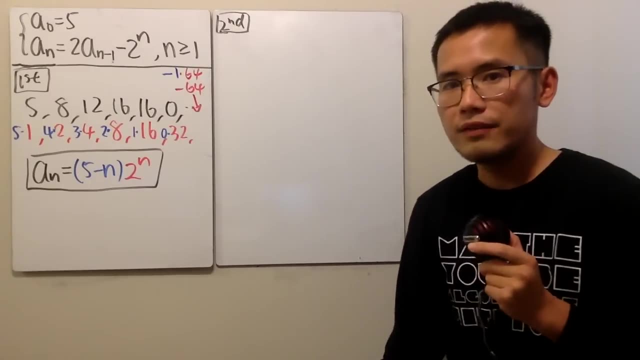 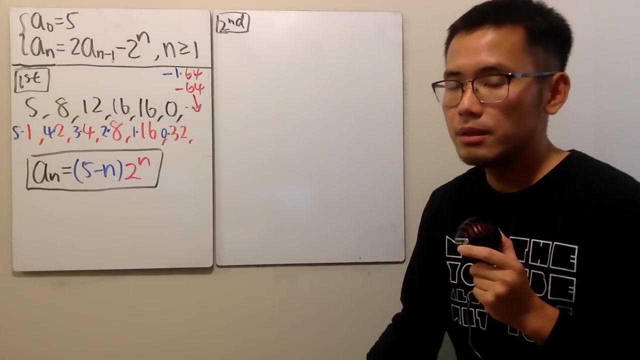 And some people also call this to be the recursive formula And difference equation, etc. etc. It depends on the kind and all that stuff. Anyway, though, hopefully you guys have taken differential equation, because I'm going to make a connection between this with the linear differential equation- 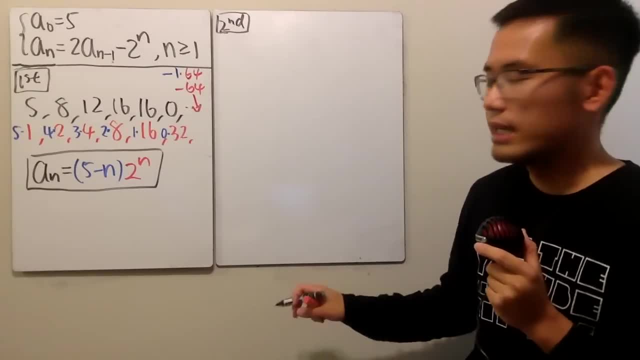 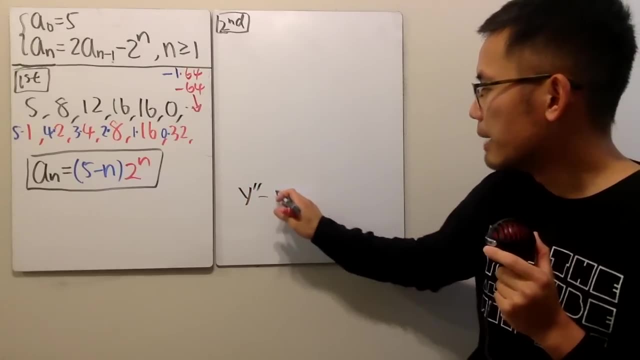 In particular maybe the higher order. So let me show you guys this right here. Suppose you have a higher order, let's say second order, differential equation. Let's say y'' minus 3y' and then plus 2y. 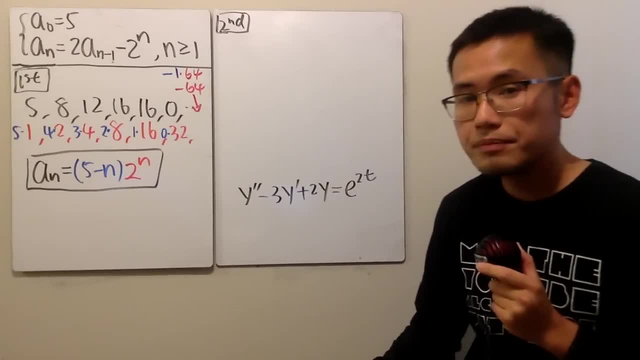 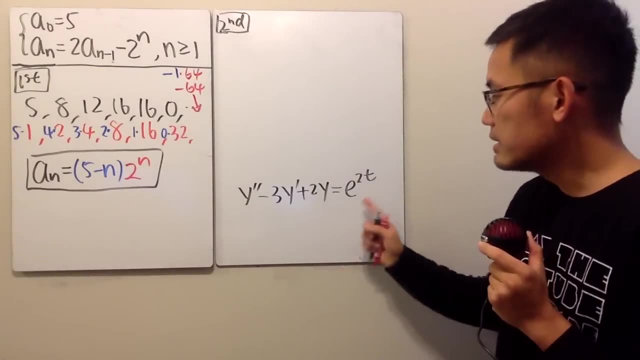 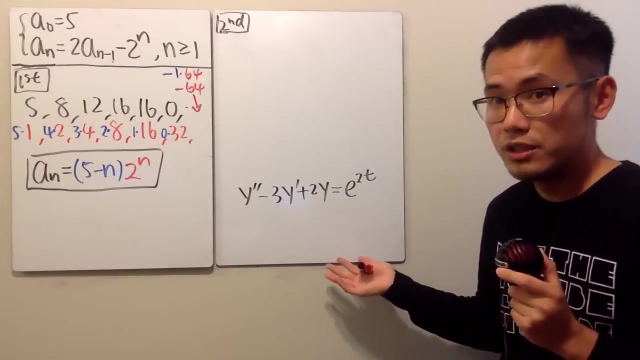 Equal to e to the 2t. like this, This right here it's a second order linear differential equation with constant coefficients. But this right here is not homogeneous, because the right hand side, we have the function Right. If this was equal to 0, then it's a homogeneous situation. 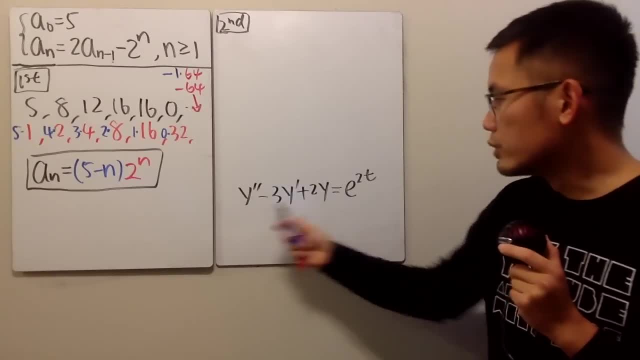 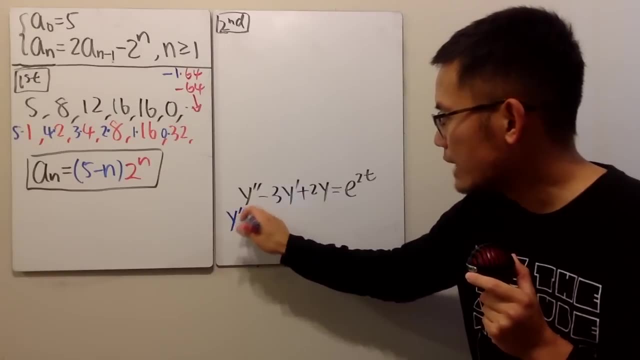 Now this is how we are going to do it, To solve this differential equation. what we do first is you consider the homogeneous situation, Namely, you want to solve: y'' minus 3y' plus 2y is equal to 0.. 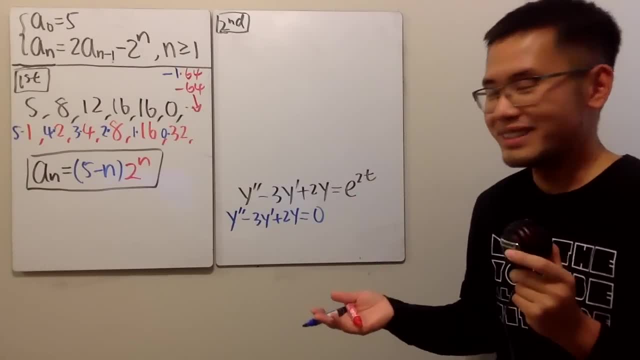 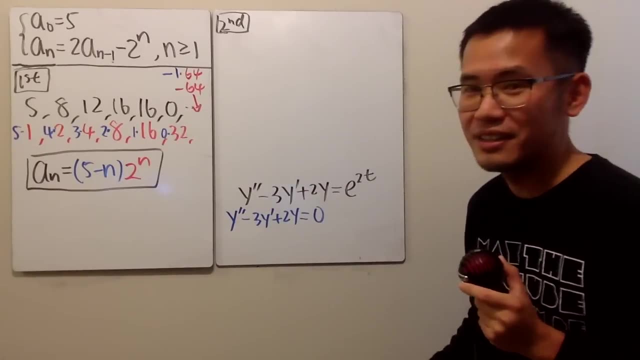 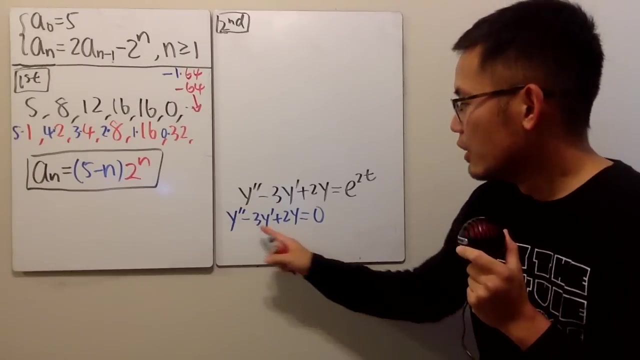 And the way to solve that is: you start with a guess. If you would like to say that Some people hate that because nobody likes to guess, Just like guess and check, That's not an idea. However, if you really think about it, you can see that there's only actually one good choice. 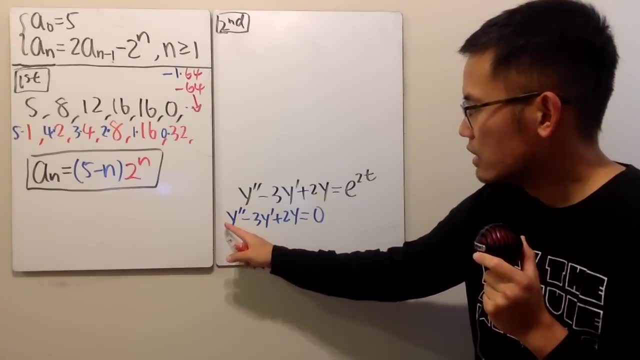 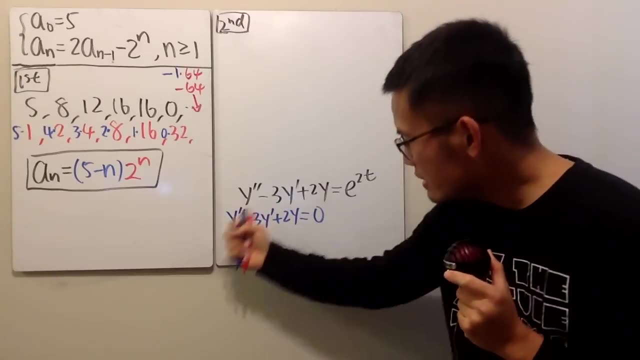 Right here you see the y', y''. they are just like a constant multiple, All of each other in order to have everything add up to be 0. And the only function that will make that happen is when y is equal to the exponential function. 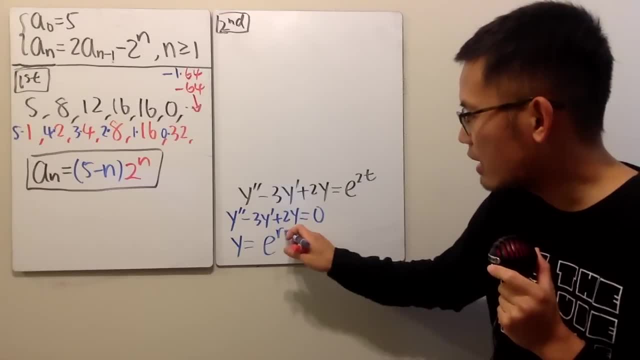 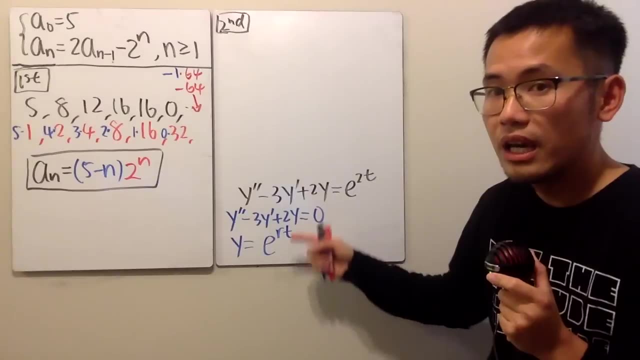 And we can write it as e to the some constant r times t like this: Because, again, if you differentiate this, you will get r? e to the r? t power, And if you differentiate that, again you get r squared times e to the r? t power. 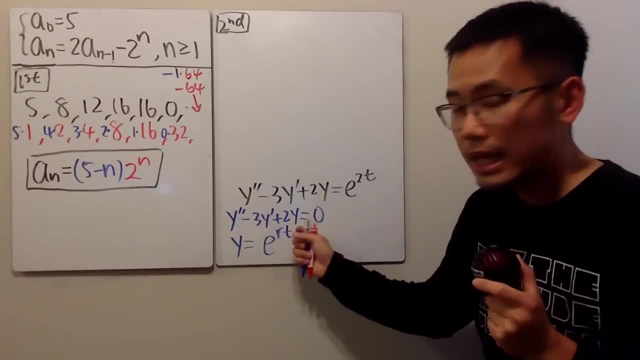 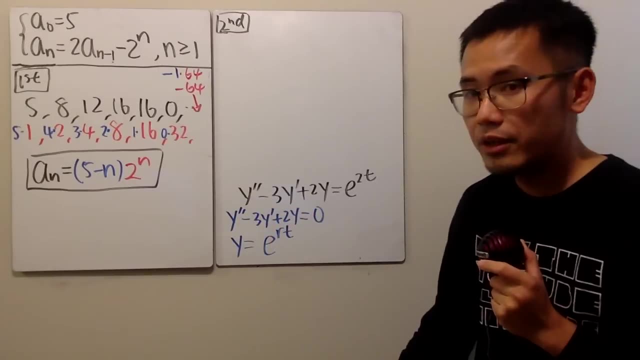 And you see they are just a constant multiple And if you plug that in, then you will be able to solve for what r should be, And then that's how you can get the solution to the differential equation right here, And this is again called the homogeneous differential equation. 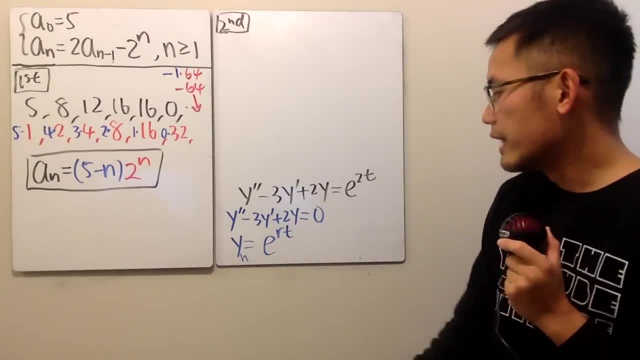 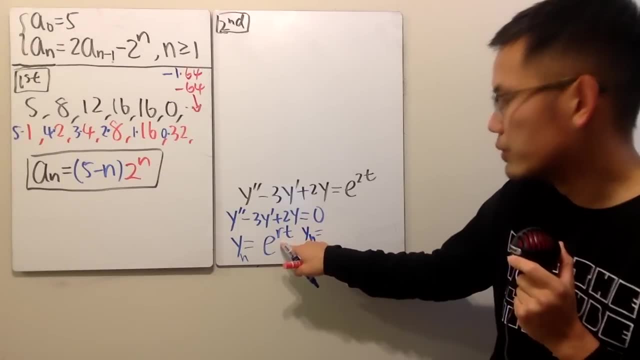 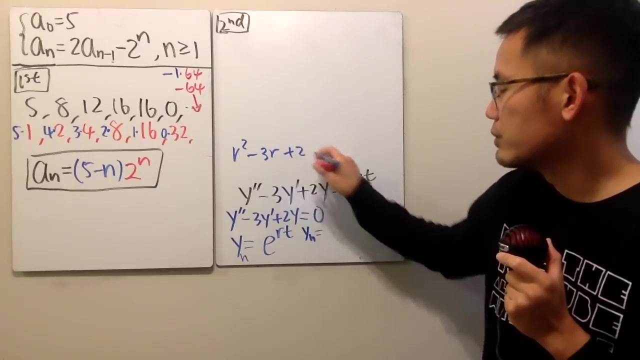 And usually we can put down the yh for this. So that's the idea And in case, if you are interested, I will tell you yh. this right here you will get. r is equal to well. you pretty much will have to solve r squared minus 3r and then plus 2.. 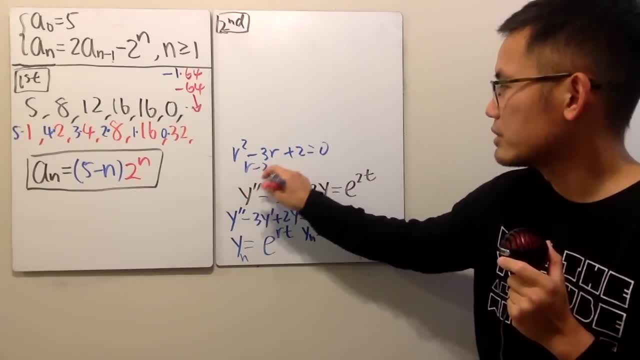 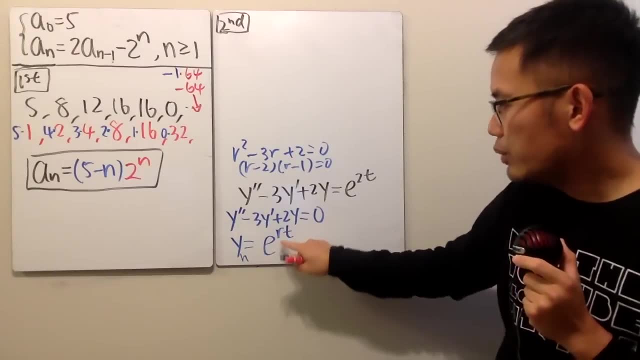 So you can just have to make that equal to 0. And then it's r minus 2.. And then r minus 1 equal to 0. So in another word, your e to the r, t, your building blocks to your solution. I will tell you. 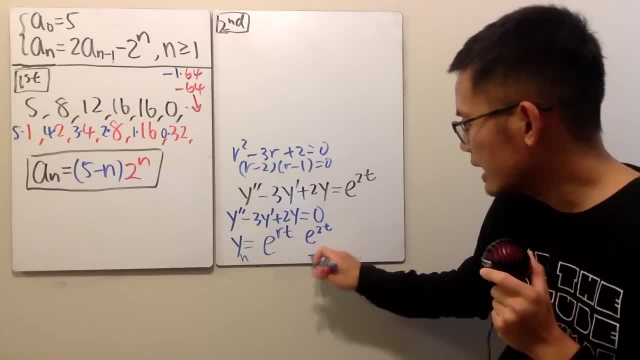 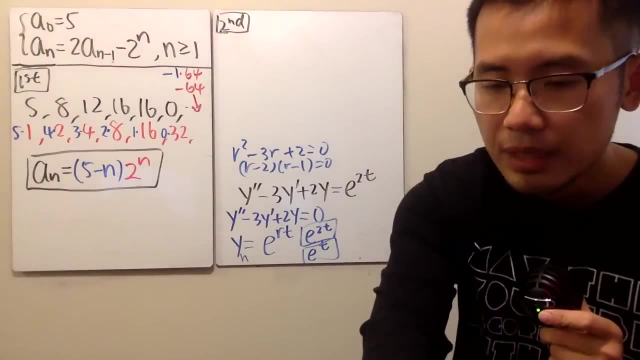 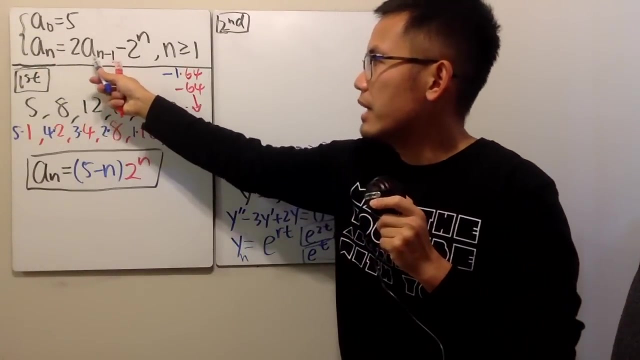 is going to be e to the 2t and the other one is e to the 1t. So these two are your building blocks. for your final solution, I will say, And we are going to do the similar thing right here. What we are going to do is you see that we have the a sub n here, and then 2 times a sub n minus 1.. 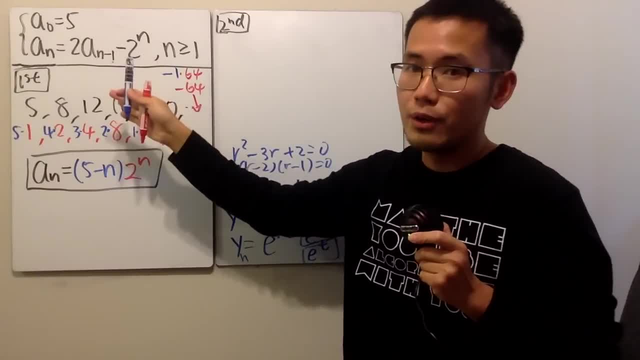 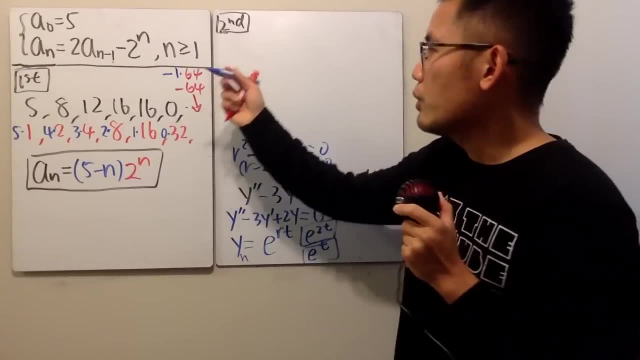 This is the one that does not have the a or whatever right. Just like this, This one does not have the y or the y prime, whatever. Just ignore that for now. So let me just again write this down right here for you guys. 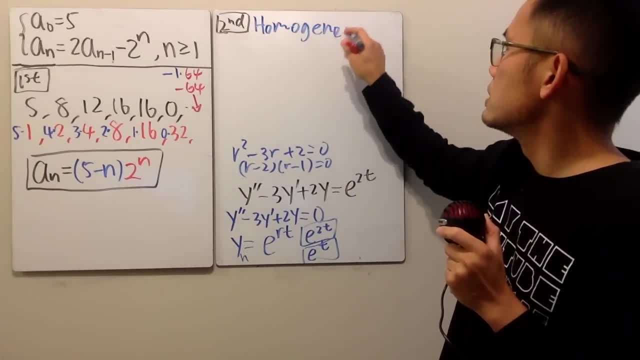 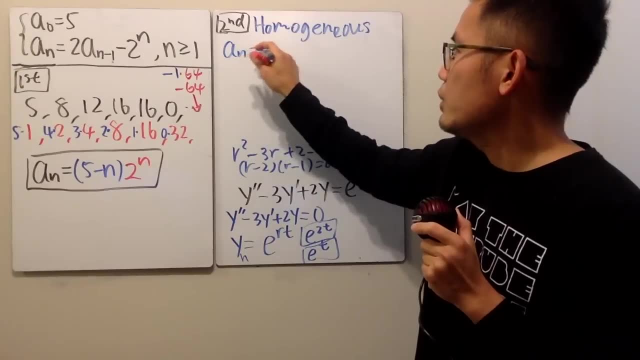 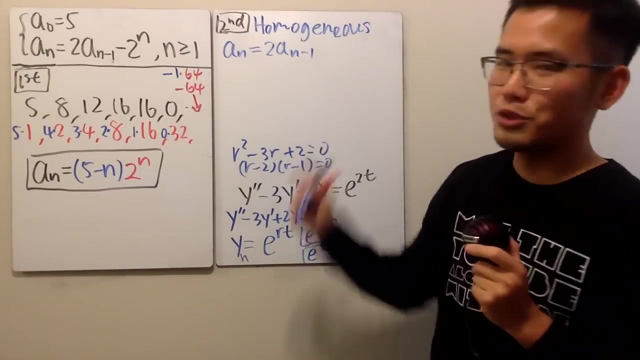 This right here is the homogeneous situation, And what we are going to do is I am going to be looking at an equals 2 times a sub n minus 1.. I am going to try my best to solve for this, But this is not so bad at all. 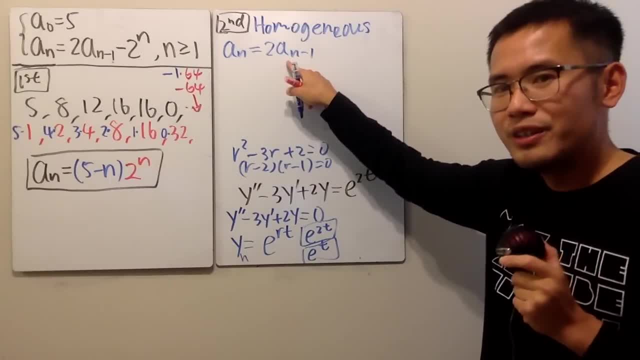 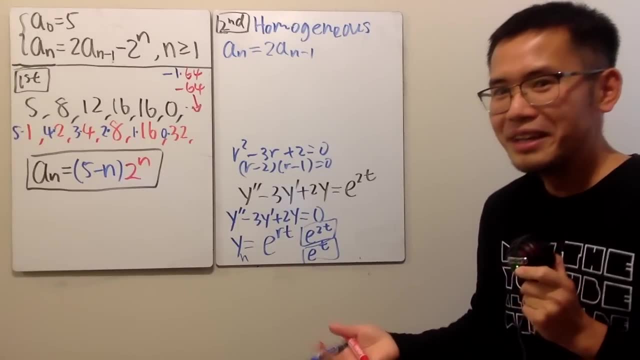 How come? Well, if we look at this carefully, this is just telling us: multiply by 2 with the previous one, multiply by 2 with the previous one, multiply by 2 with the previous one, namely 2 to some power. 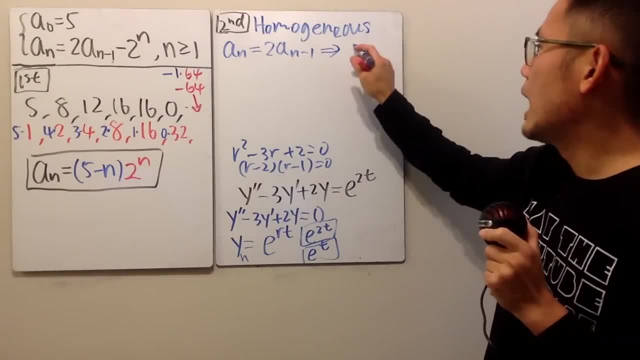 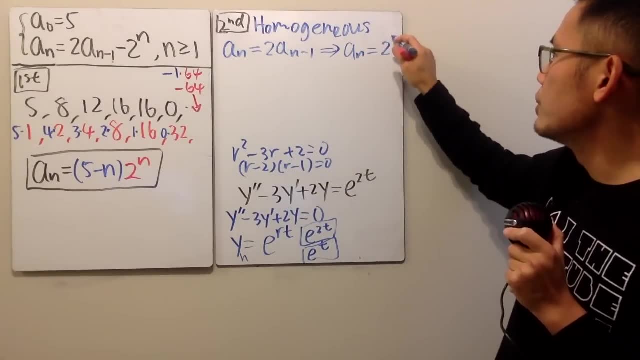 Exponential situation. This, right here, is telling us. our homogeneous solution, right here, should just be. let me write down a n. 2 to the nth power, right. Well, Now you might be wondering what if sometimes we have like something else? 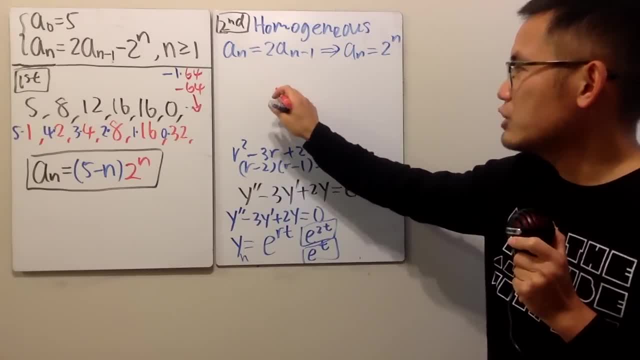 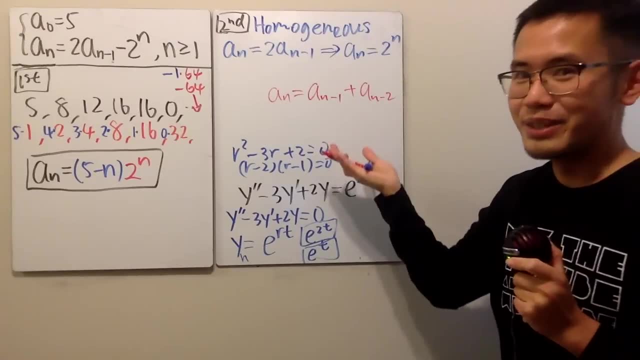 For example, for the Fibonacci sequence. For the Fibonacci sequence you have a n, that's equal to a n minus 1 plus a n minus 2.. This is not so easy to just look at this and then figure out what the base should be right. 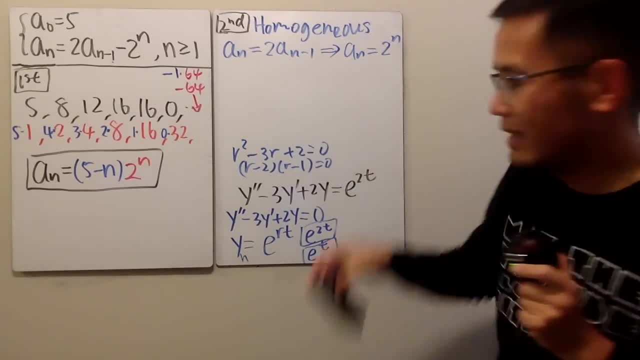 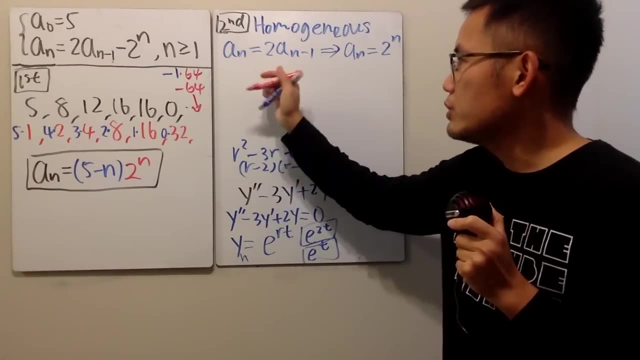 So this is how you are going to do it. It's very similar to what we just did right here. When we have this, Well, our initial guess is that a? n is equal to 2.. Our initial guess is that a? n is equal to r, again for some base, and then raised to the nth power. 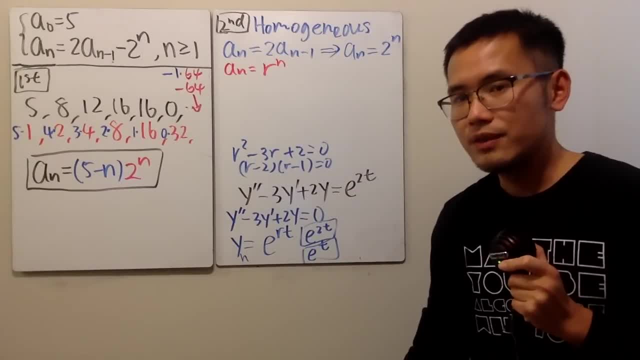 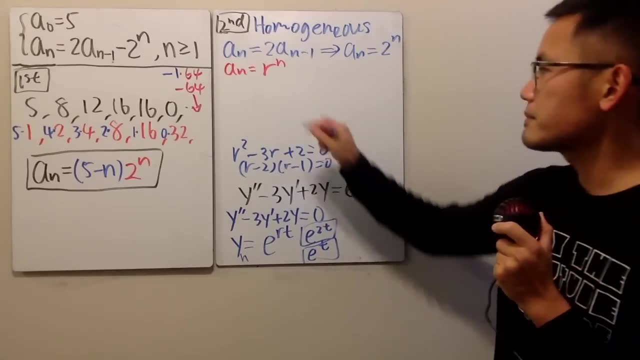 In fact, this is how I solved the explicit formula for the Fibonacci sequence, which I have a video for you guys already from three years ago, So go check it out if you would like. Well, now I will do the work for you guys. 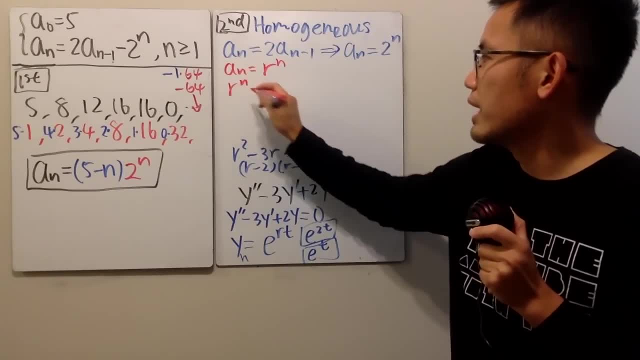 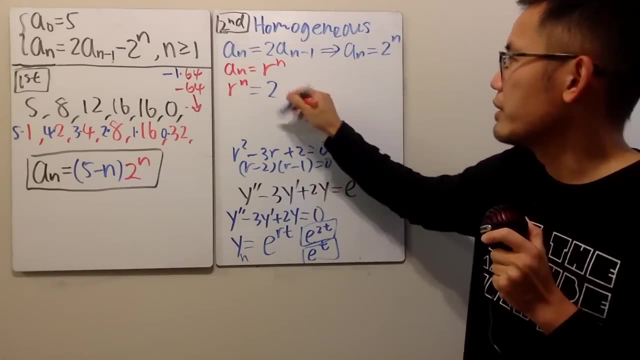 a n is equal to this. so I will just put down r to the n, which is equal to. here we have the 2, and a sub n minus 1 is just. you put n minus 1 right here, so it's r to the n minus 1.. 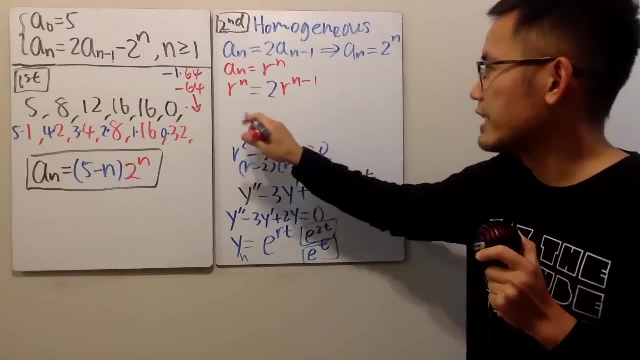 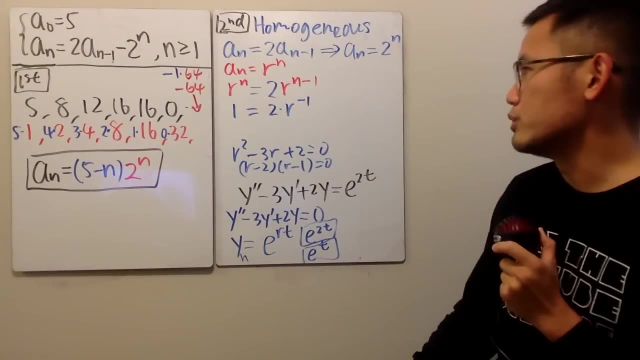 And you see, both of them have r to the nth power. we can just divide that out. you get: 1 is equal to 2 times r to the negative 1.. And of course we could divide. it's because r should not be equal to 0.. 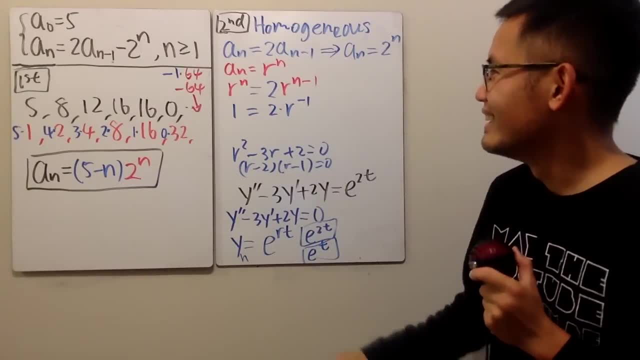 If r is equal to 0, we are not doing any math right here at all, right? Anyway, right here you can see that r to the negative 1 times 2 is 1, so that tells us r is equal to 2.. 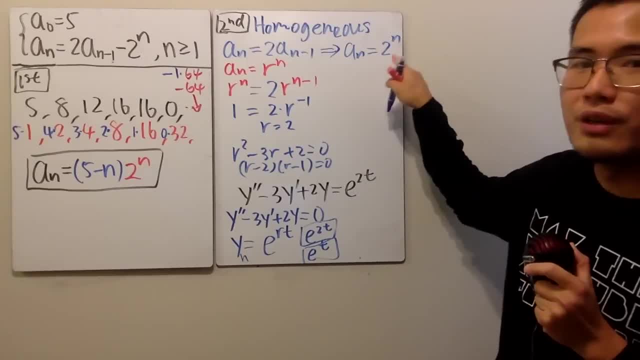 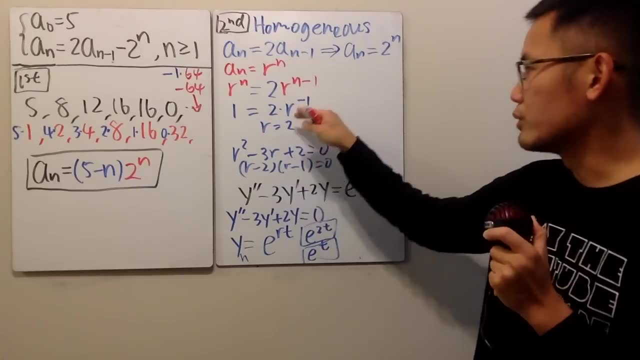 Then you can just put the 2 back right here, and that's how we figure this out, And we only have 1r, because this is just, you know, r to the negative 1 power. that's all right, And this right here. we have two solutions, because this is the second order. 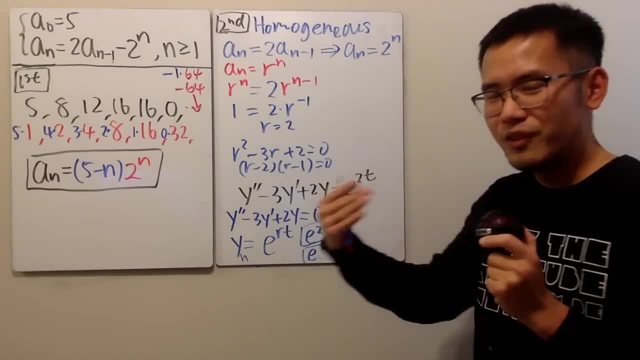 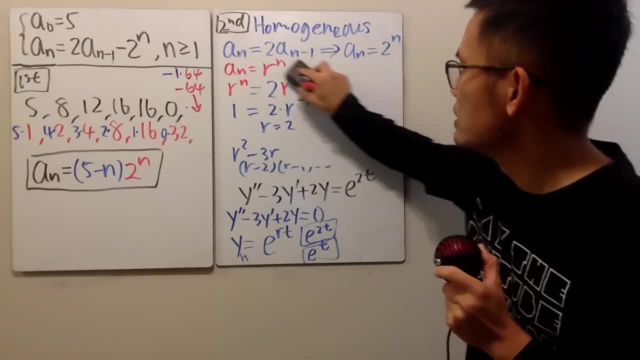 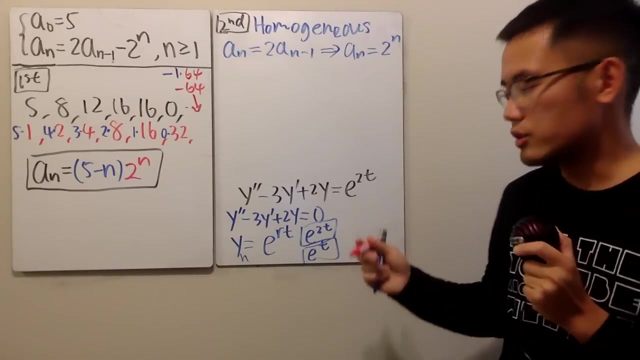 And you see this right here- is n minus 1, so it's like the first level difference. that's the idea. Alright, so that's good. That takes care of the homogeneous situation. However, though for the particular situation it's trickier, so pay close attention to this. 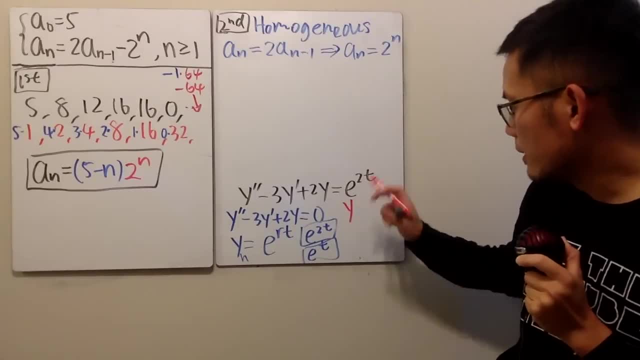 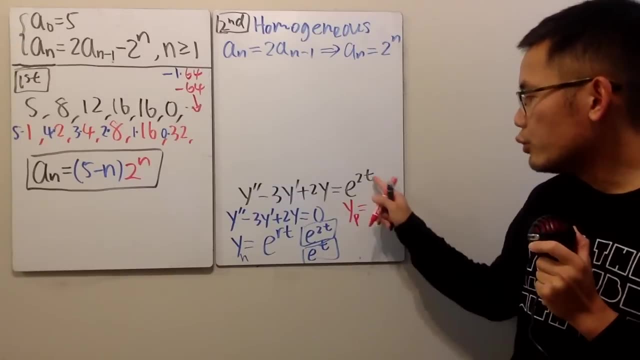 Again, I will use this as the example For the particular solution. if you look at the differential equation situation, well, you have to pay attention to the form of this function, which is exponential, named the e to the 2t. 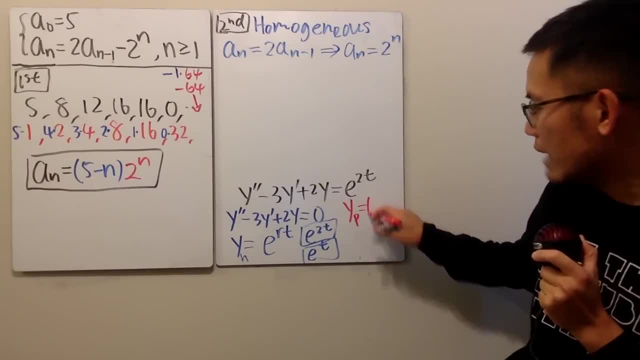 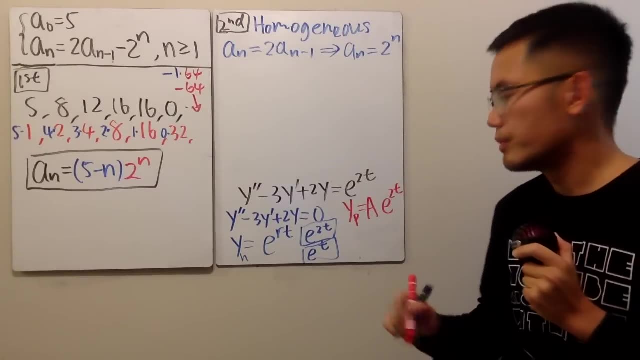 Well, the particular solution: you should have some constant, multiple, let's say capital A times this, which is e to the 2t. But here's the problem, If you put down e to the 2t, in fact, 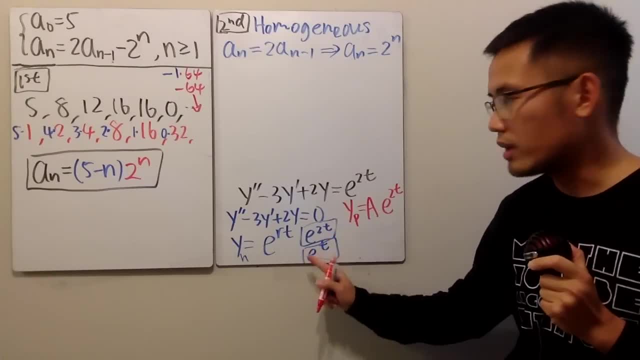 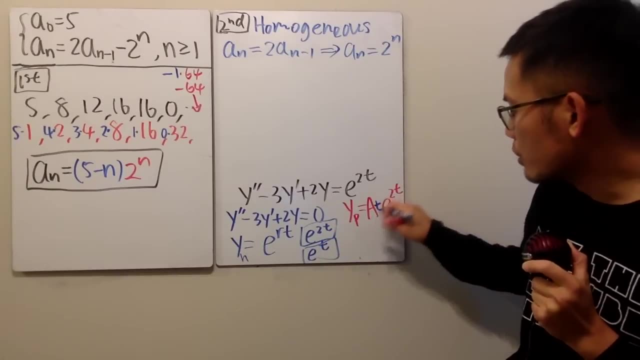 we have a duplication right here already from the homogeneous situation, right? So the way that you're going to fix this is that you are just going to multiply this by t, Why? You can check out my differential equation video on that. You can check out Dr Plan's video on that. 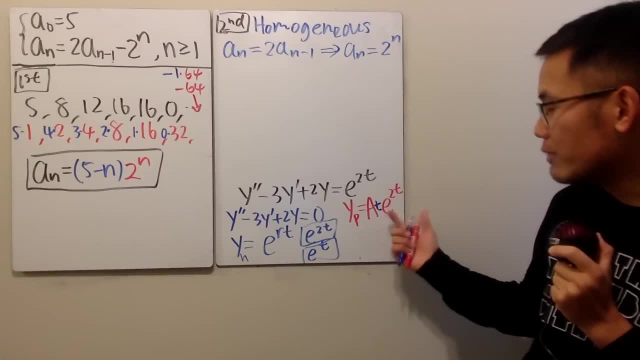 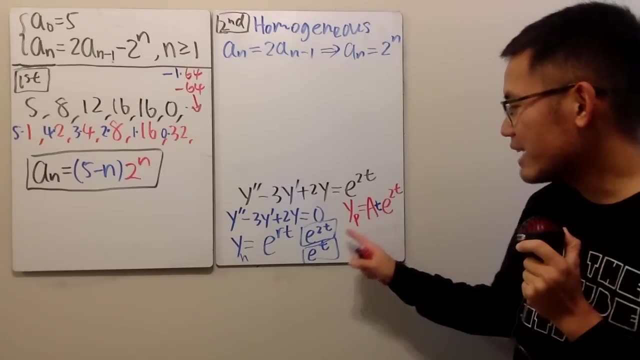 But for now, the purpose is just that I want to show you, guys, you have to make sure this, and that they have to be linearly independent in order to come up with new solution, Because, again, they are just the building blocks. 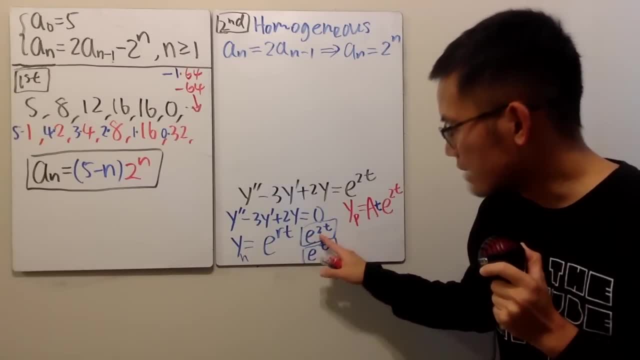 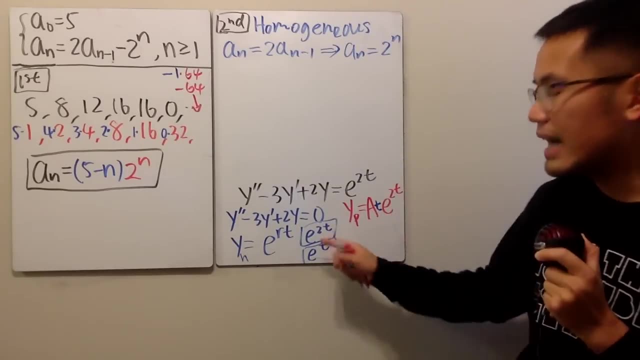 Later on you will have to multiply this by a constant, likewise that to get the general solution. If you just have a times e to the 2t, this and that match No good. So you just multiply by t, it will work out very well. 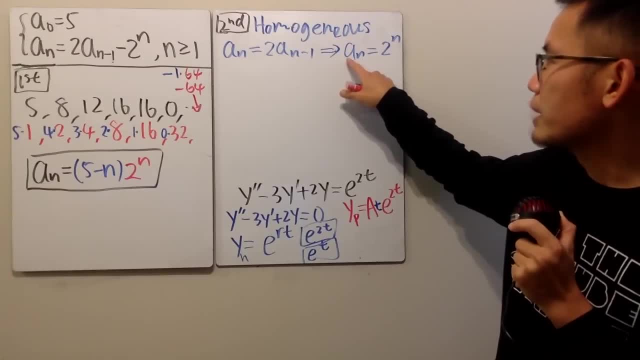 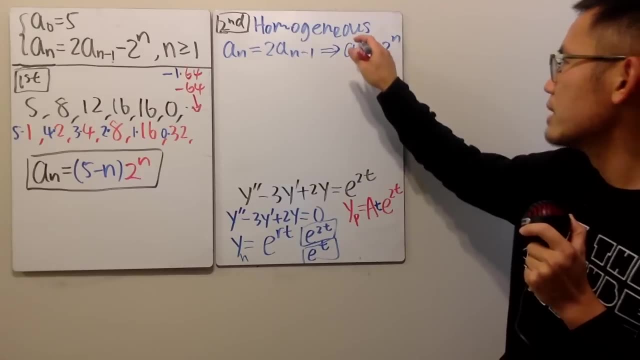 Now have a look. This right here. we have the homogeneous solution right here already. And some people will say this is a n, and then with the little h, little h on the top, with a parenthesis, but this does not mean you take the derivative right. 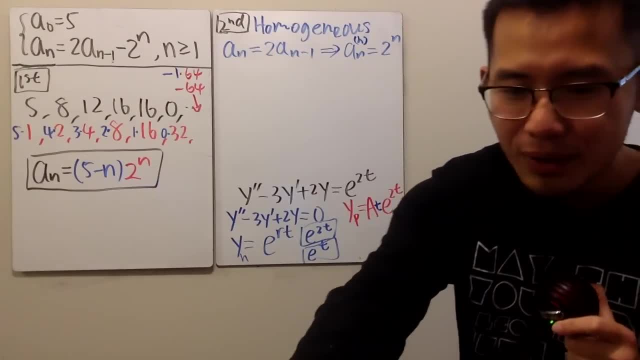 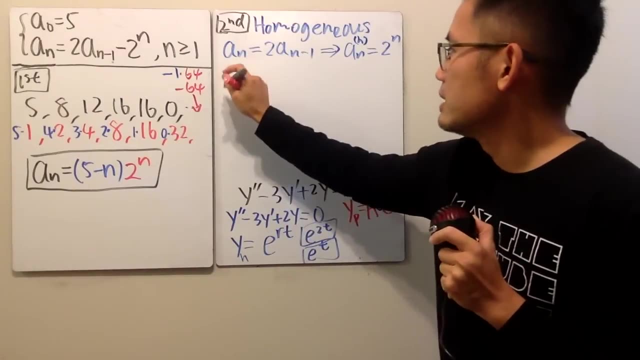 So it has nothing to do with the derivative in this notation. Now here we go. We are going to focus on the particular solution. I will do this one in black. So here is the particular situation: Partic, No, not particle. 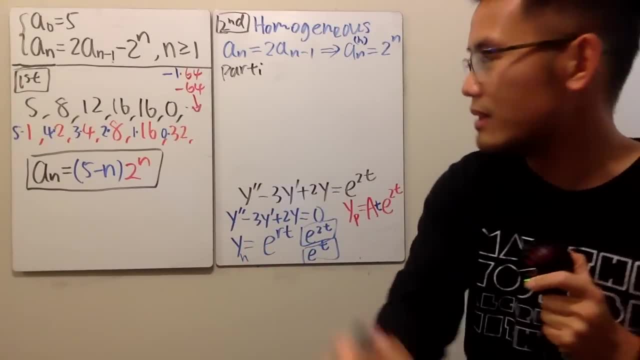 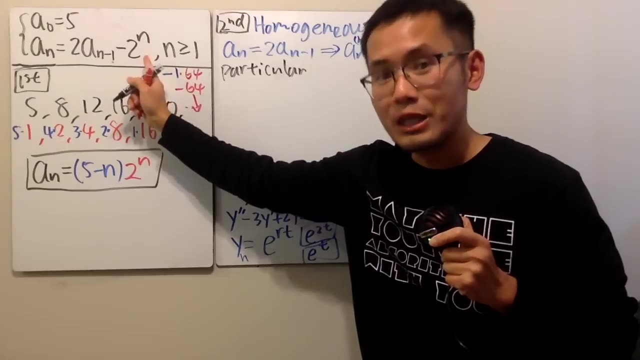 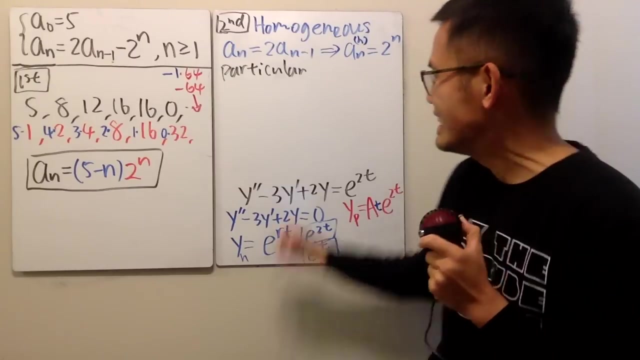 Partic, Particular Partic. There we go. Particular situation. Well, you have to just look at what kind of function, what kind of sequence this is. We have 2 to the n. Ah man, I am going to write down a n. 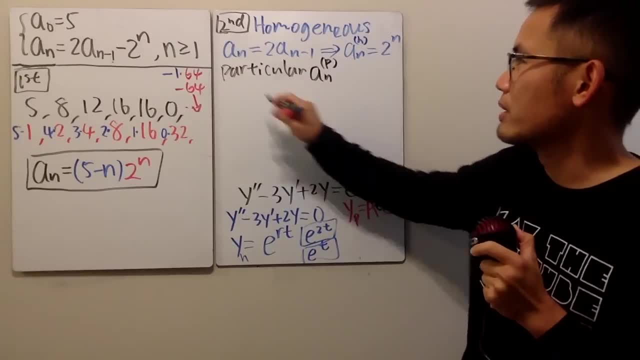 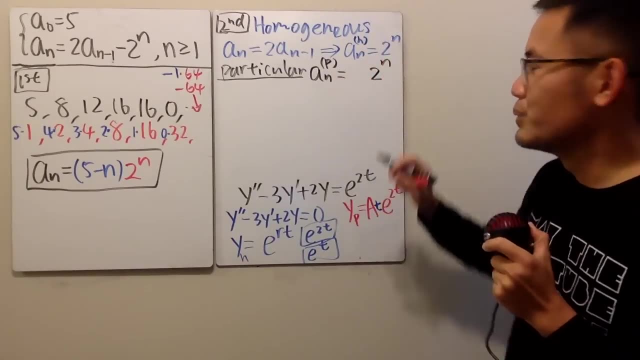 and with a little p right here. parenthesis, because for the particular situation We have 2 to the n right here, so this is also going to be 2 to the n, with the constant in the front. Again, let's put down capital A for that. 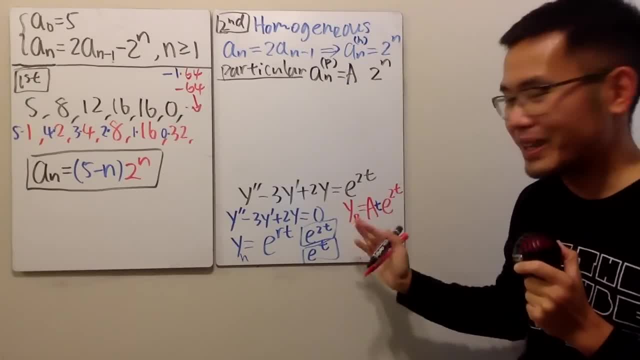 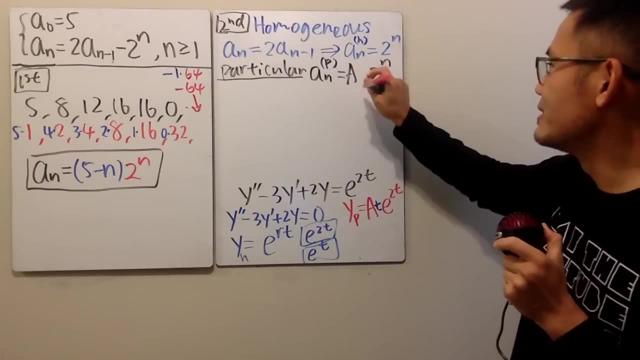 But just like this, right here, this and that match. What do you see what we can do? Yes, all we have to do is just multiply this by n. That's it. No kidding. Right Again, I can do more videos on that. 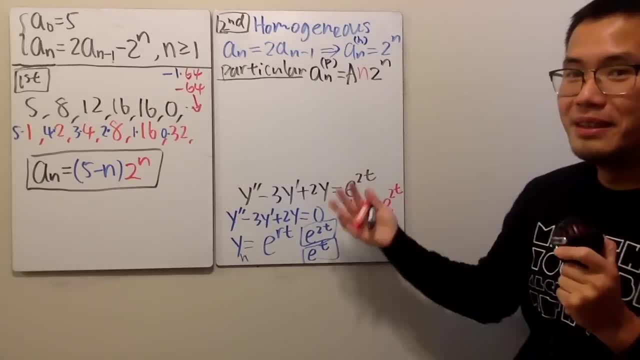 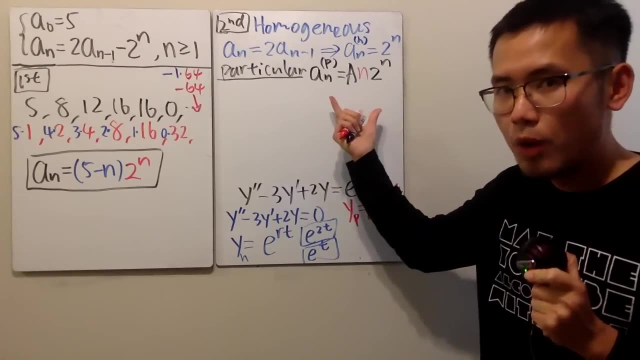 if you guys would like. But from that, hopefully this right here is satisfying. You know you guys are satisfied with this already. Okay, Once we have the particular form, then just go ahead. put them back to the original. 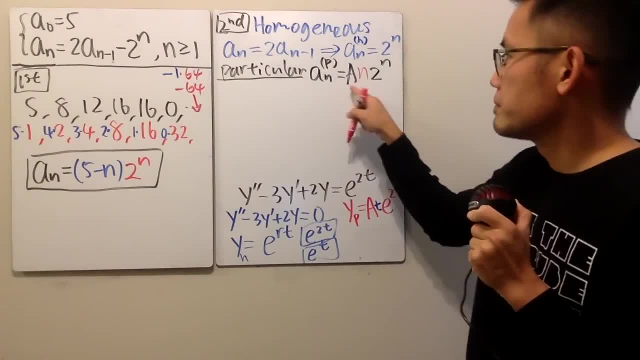 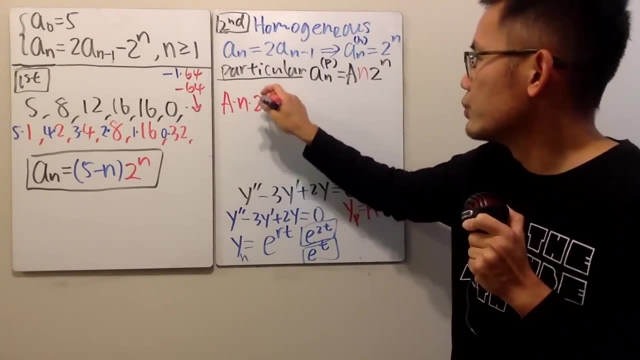 Because we have to figure out what A should be. So this right here, I will just put it down right here: on the left hand side, We have capital A times n and then times 2 to the n and that should be equal to. 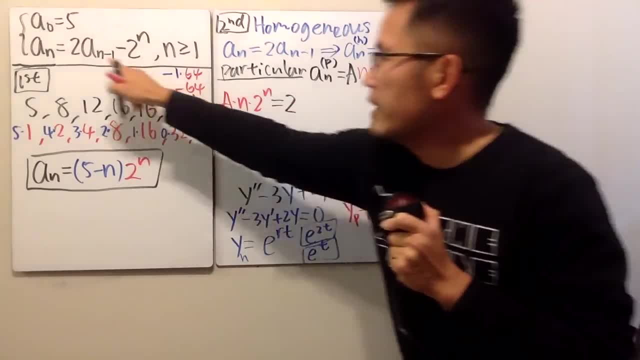 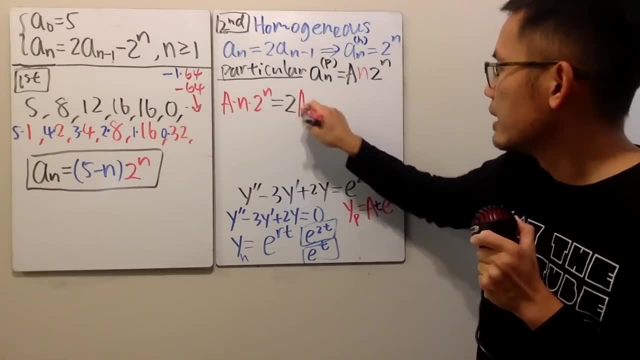 we have a 2 right here and then A sub n minus 1.. Well, this will become n minus 1,, likewise for that. So we have A and then n minus 1, and then 2 to the n minus 1.. 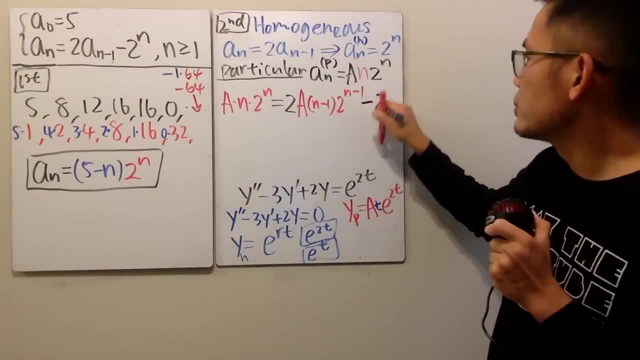 And lastly, we have the minus 2 to the n, minus 1.. Minus 2 to the n's power, And now we just have to focus on how to solve for capital A right here And bye-bye. differential equation. 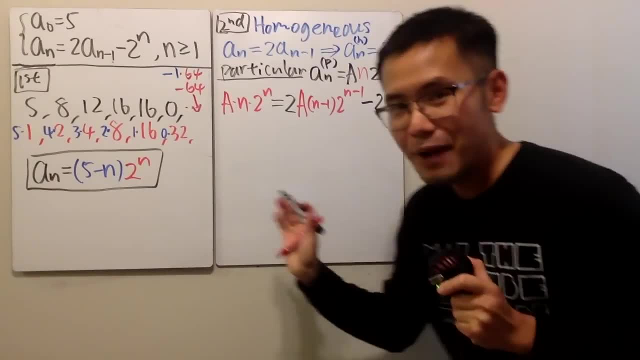 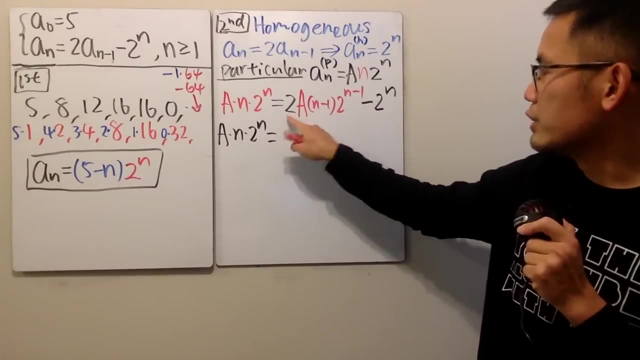 I'll see you guys soon. All right, Now here's the deal. The left hand side is still A times n. times 2 to the n Multiply, So you see 2 times. this is just 2 to the n. 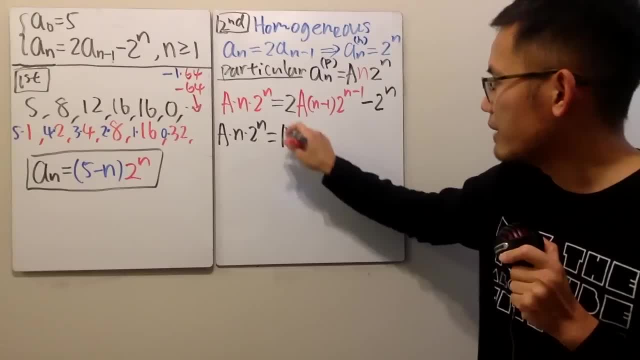 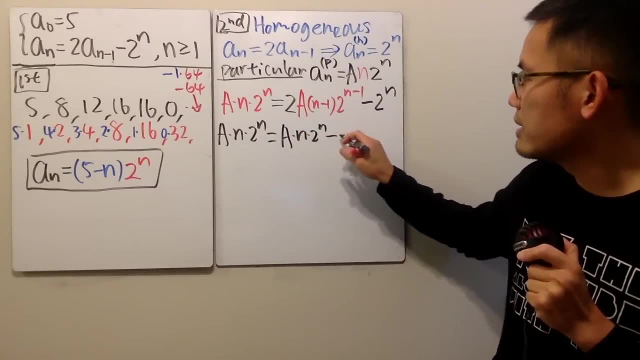 which is nice- A times n times 2 to the n. So we have A times n times 2 to the n. And then again we have 2 to the n times A times negative 1. So it's minus. 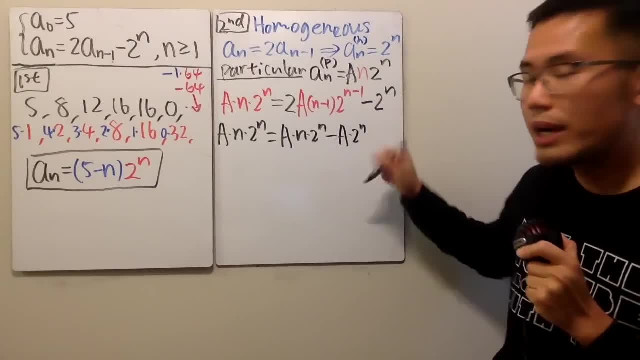 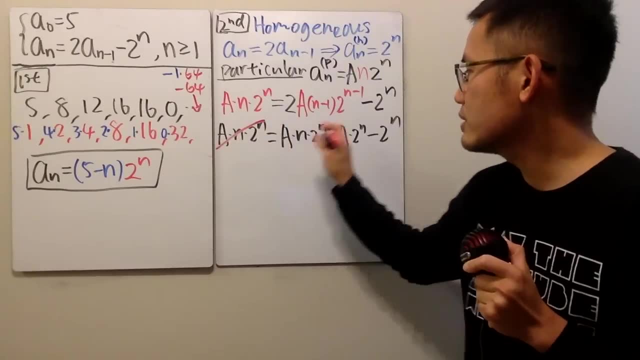 A times 2 to the n. Then right here we have minus 2 to the n. Now have a look This. and that they are the same thing. So of course they can just cancel each other out. Very nice. 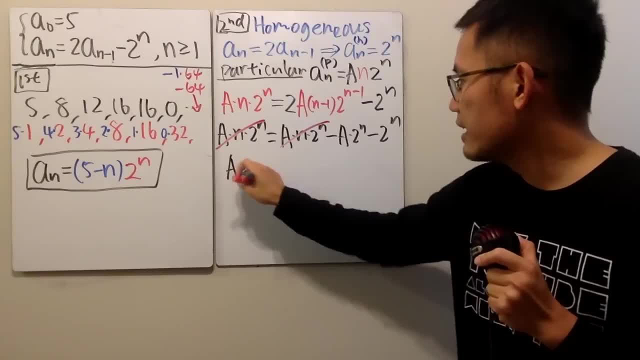 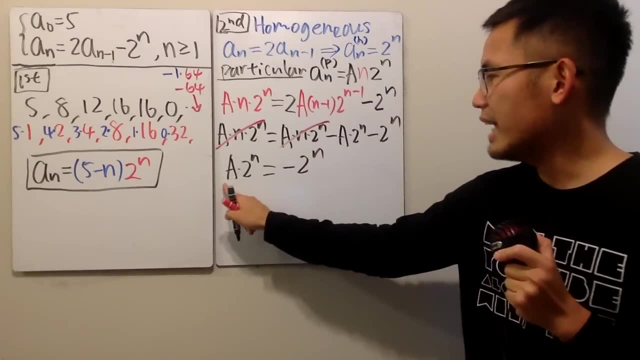 And I will just move this to the other side, and I get positive A times 2 to the n. that's equal to negative 2 to the n. So what does that mean? A has to be negative 1.. 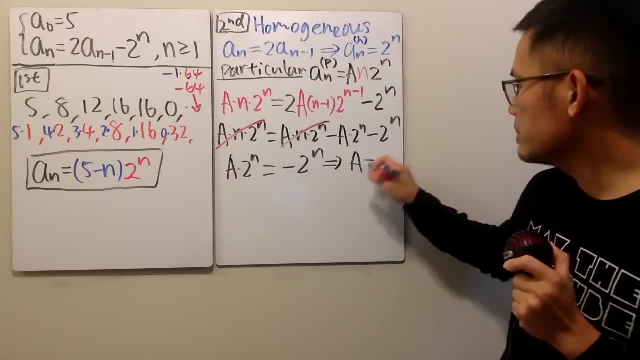 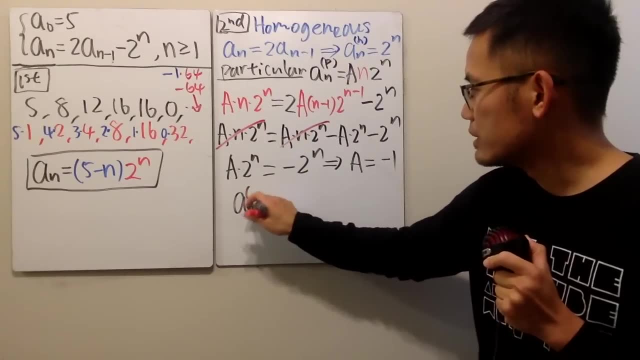 So that's very nice. Right A has to be negative 1.. Now we can see that our particular solution here, A, n with a little p like this, A, is negative 1.. So I just have to put on negative 1, right here. 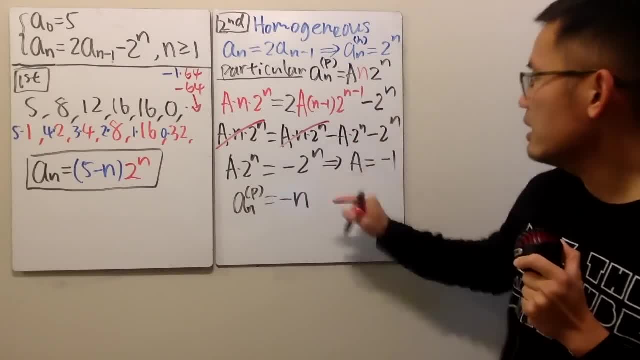 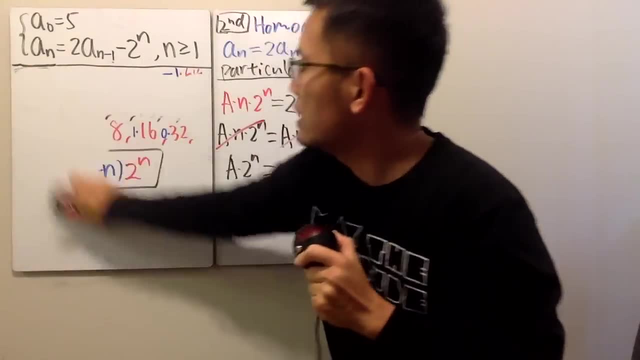 and then times n, which is going to be negative n, and then 2 to the n, like this: Very nice, All right. Now I will have to come back here because we still don't have the 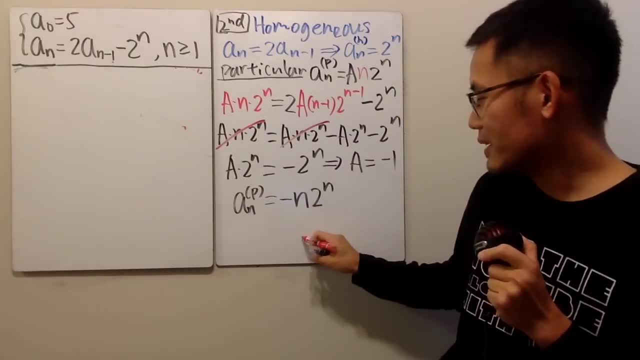 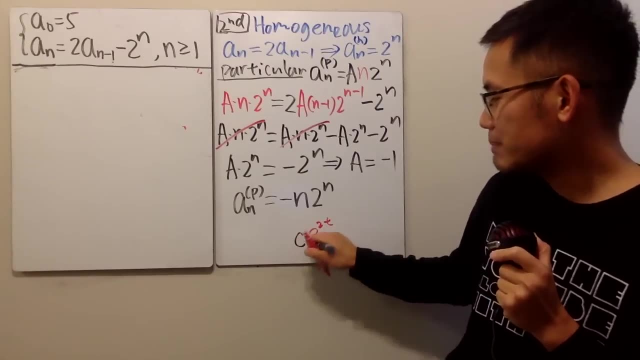 constant. yet Remember- earlier I had to bring out the differential equation again- When we have the e to the 2t and then e to the t, what we have to do is you multiply this by a constant. 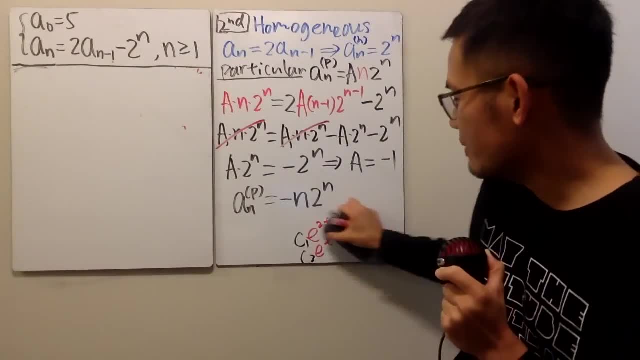 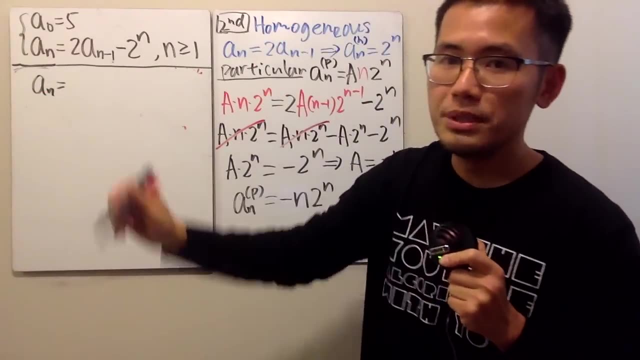 multiply by that constant. you have to find out the general solution. first, Right. Well, I will tell you the following: Right here, our A? n. this right here has to be the form of right. here we have the homogeneous solution. 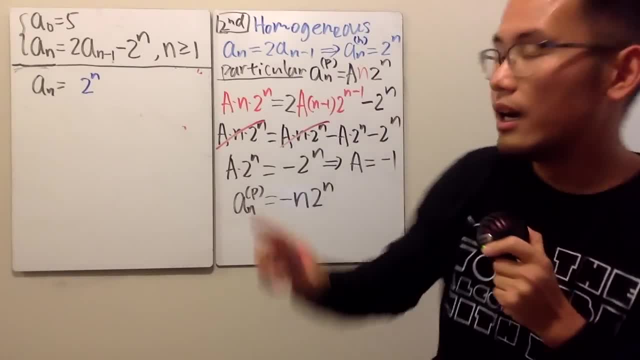 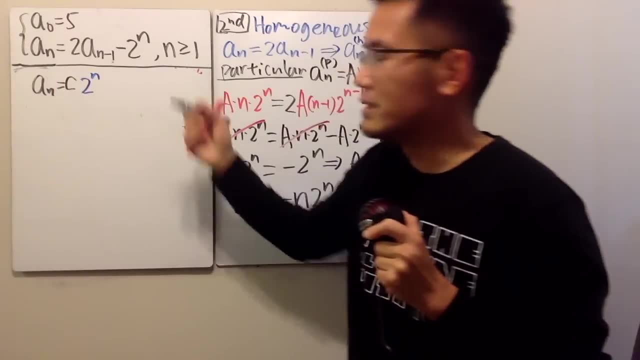 which is 2 to the n. This right here is the one that you are going to multiply by a constant. So let me just put down our favorite constant, which is c, And this right here is a particular solution already. 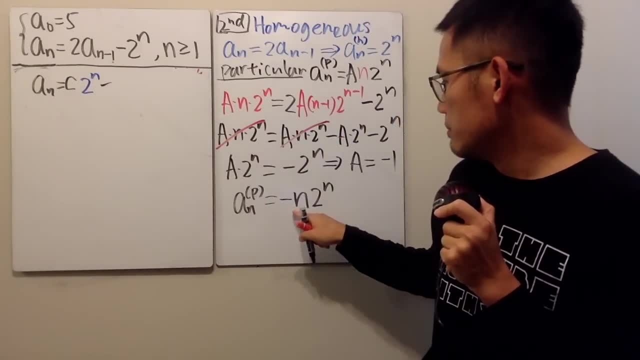 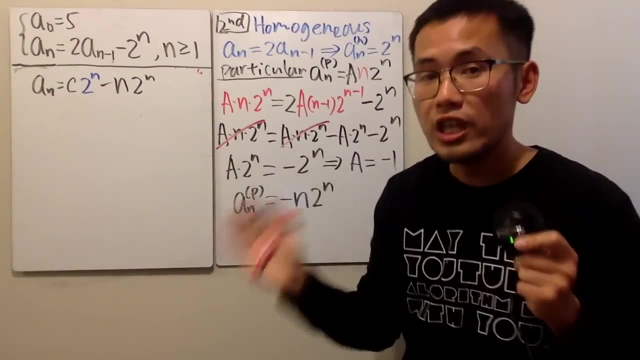 So I'm just going to minus n and then 2 to the n, like that. So this right here is our general solution for this recurrence relation. But how can we find out what c is? Of course, 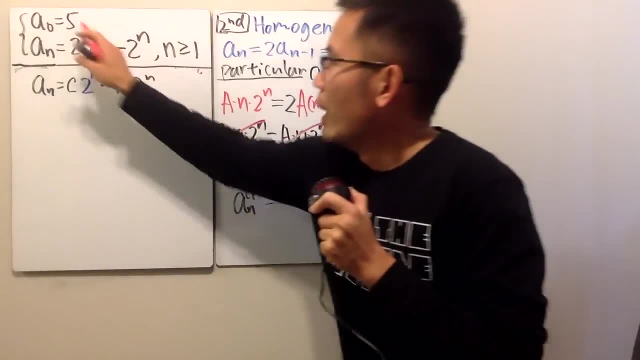 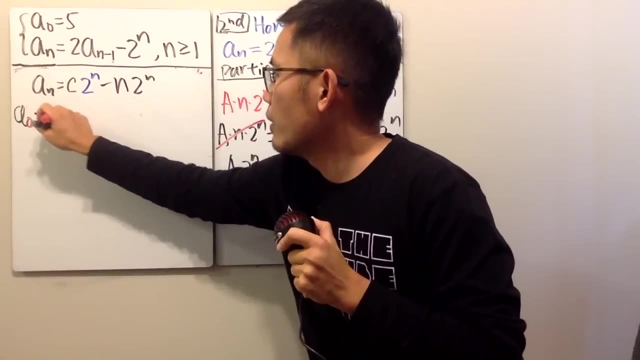 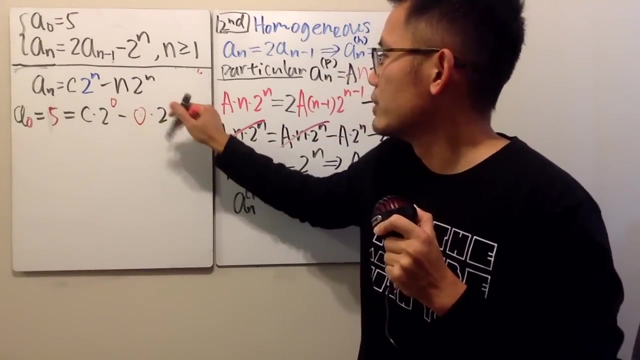 as always, use the initial condition: a0 is equal to 5.. a0 equals 5, that will tell us well: c times 2 to the 0th power minus 0, times 2 to the 0th power. 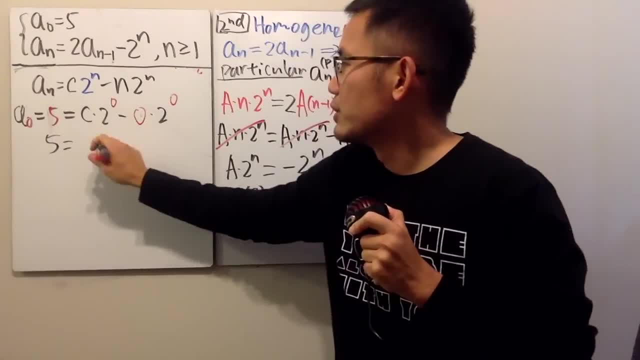 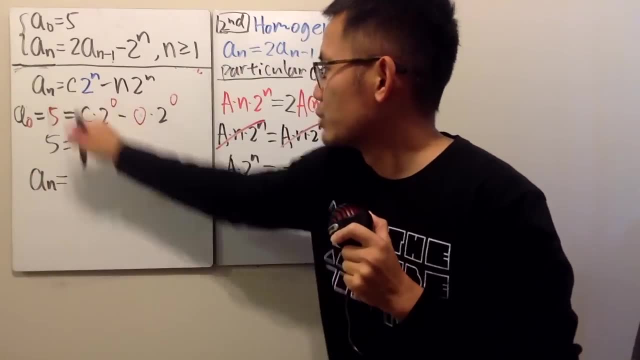 On the left hand side we just have 5.. This is just c minus 0, so c is equal to 5.. So final answer: a, n is equal to this. right here is just 5,. 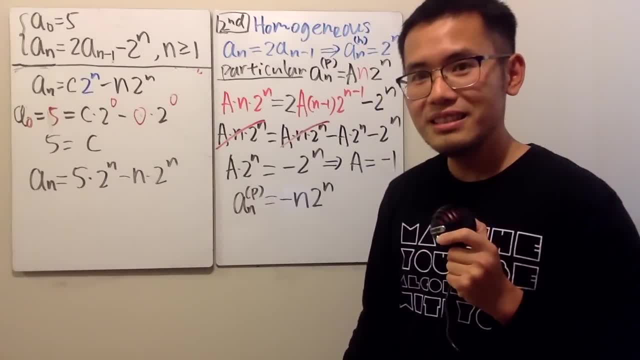 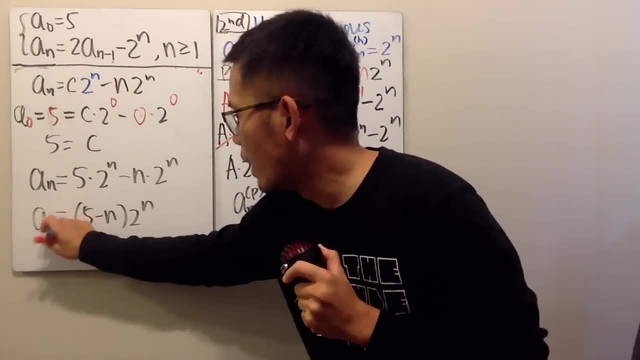 times 2 to the n minus n times 2 to the n. Yes, same as what we got earlier, because we can write this as 5 minus n times 2 to the nth power for our final answer. 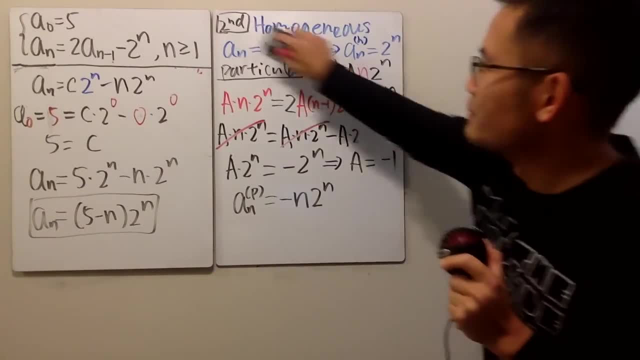 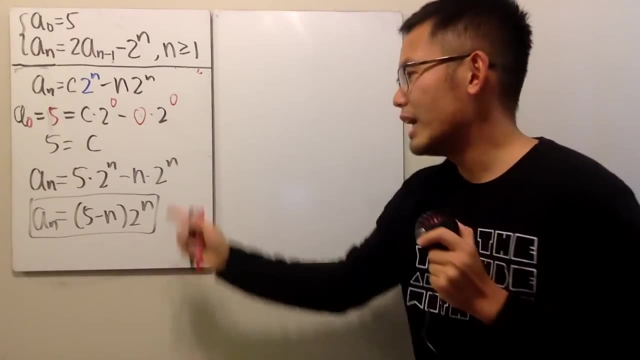 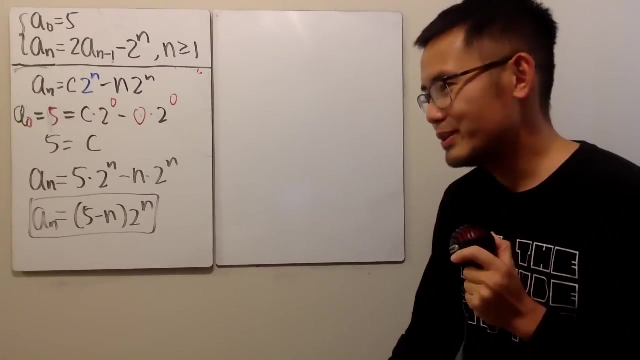 like that Right. Very cool, huh. Now the third way is perhaps another way to explain why we have to multiply by the n right here, without knowing that. I will just tell you guys the following right: Do you guys remember your calculus 2,? 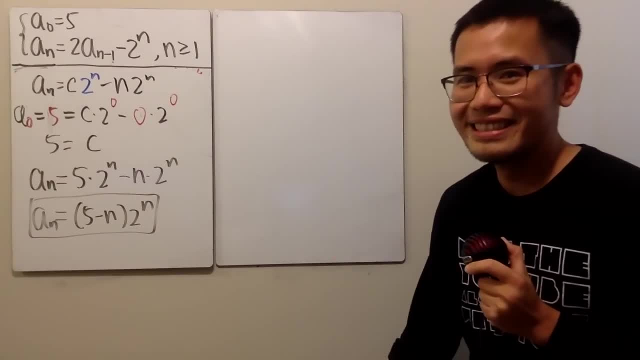 your differential equation. The part that you hate the most is that you have to use power series to solve differential equations. Yeah, I don't like that either. That's the third way. right there. Third way might be the longest. 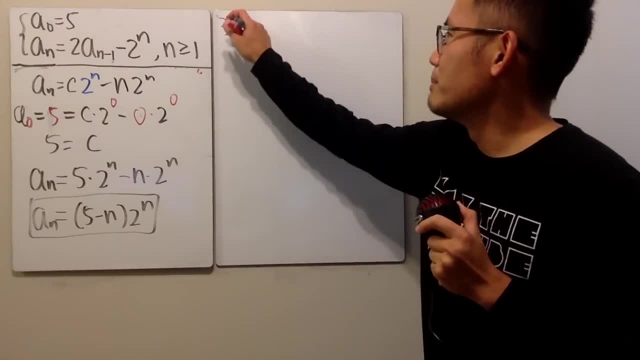 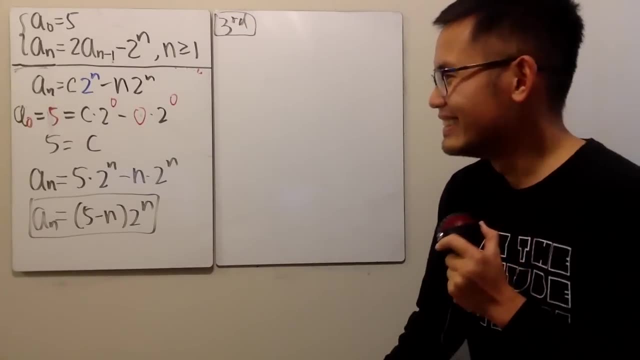 but hopefully it comes more natural. I will say: Just let me know how you guys feel after all this right, This right, here we'll be using infinite series, and the particular name for this is: 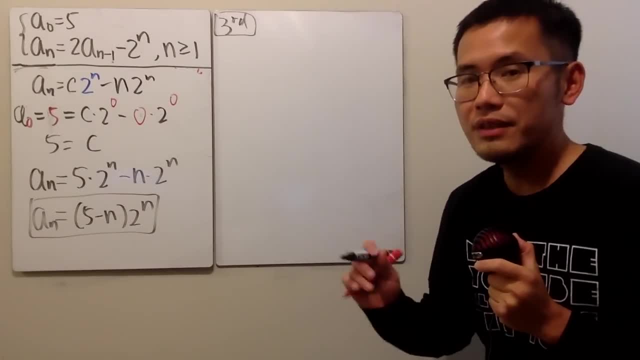 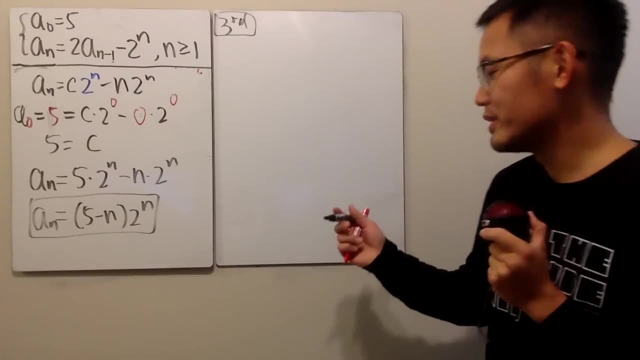 constant series, right? So this right here we'll be using infinite series, and name for this is called the generating function, right? So here we go. I will have to tell you guys what a generating function. 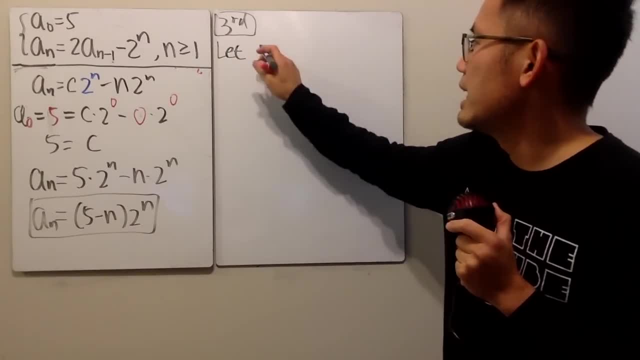 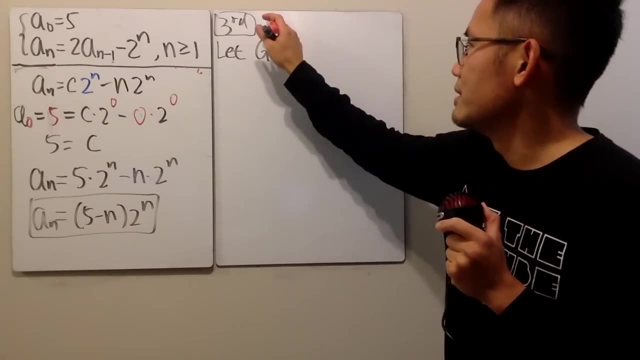 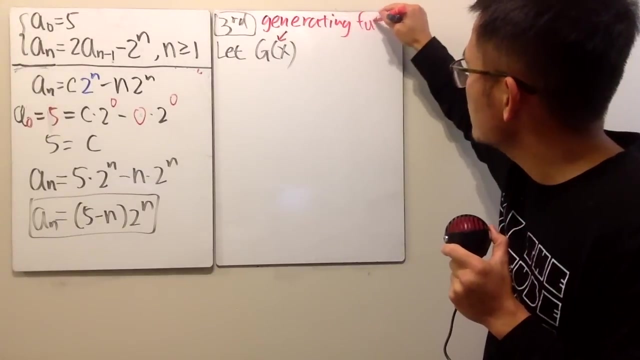 I will just write this down for you guys. I will start with let g of x and again this: right here is what we call the gf, namely the generating function. generating function, and again this right here: 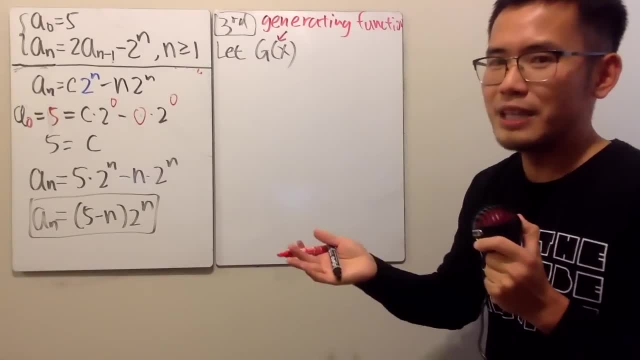 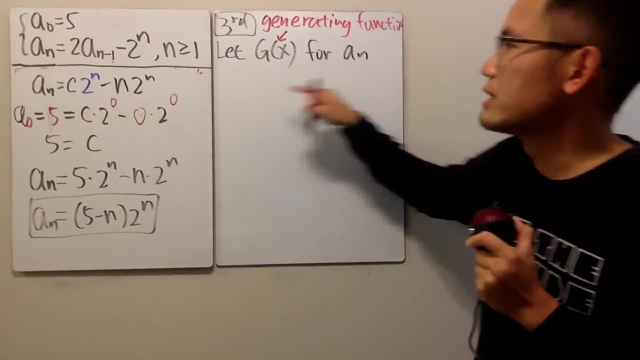 it's not so crazy, it's just like a fancy name, right, I will say, because the generating function will write it as g of x for an, which is the one that we have. let this right here. 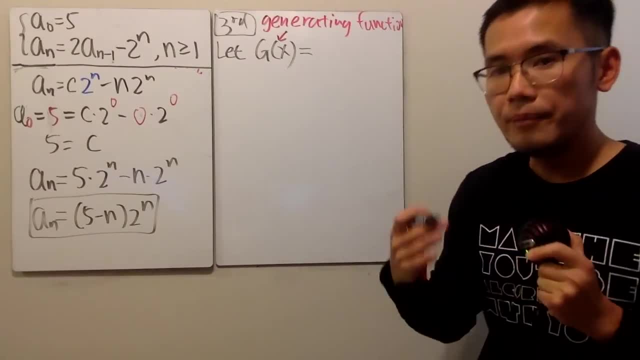 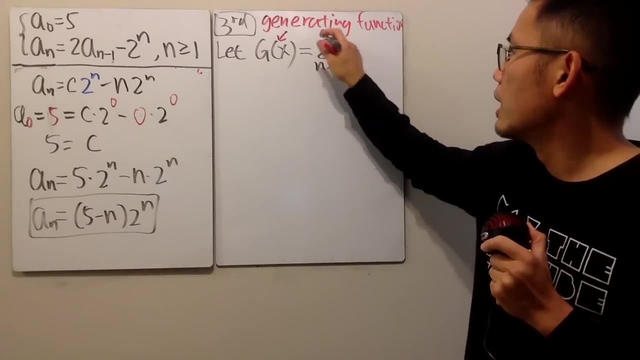 actually I will write it down like this, this right here again: it's just a infinite series, so you just go ahead and do the series, but you have to go from zero to infinity and then you just focus on. 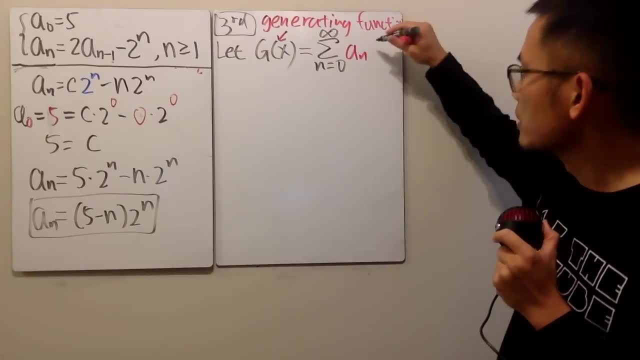 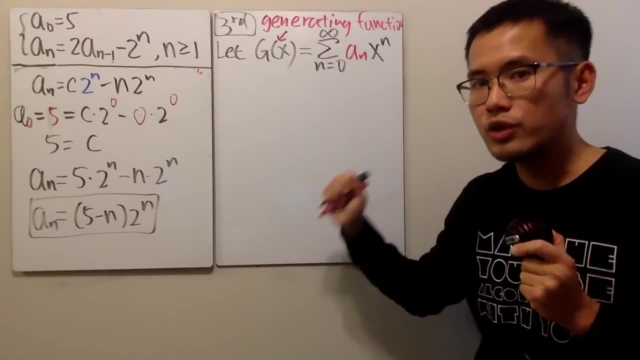 whatever the an is, and then you multiply by x to the nth power again. whenever you have a sequence, an, you can have a generating function by simply putting the an down right here. that's all. 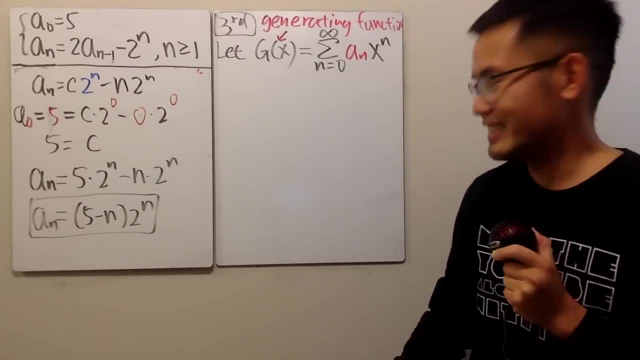 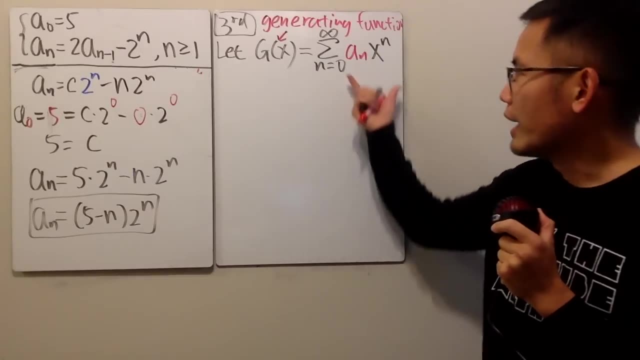 and then you can call this to be g of x. that's all, seriously, that's it. and the difference between a generating function and your usual infinite series is that, right here, we don't really care about. 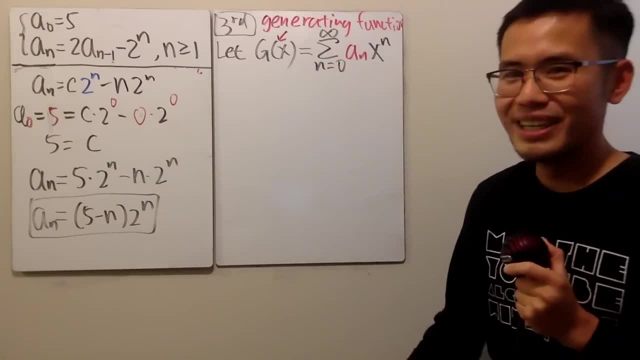 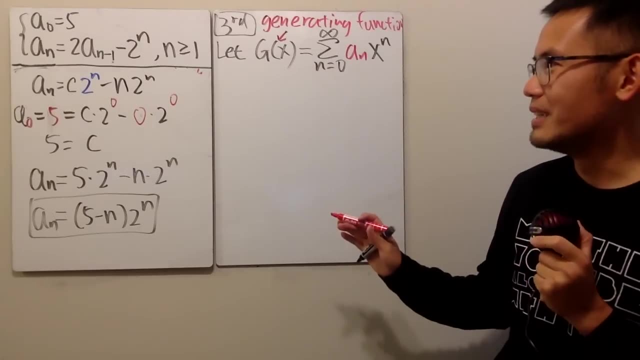 its convergence. all we care about is the coefficient, because we're trying to find a formula for the an. so this is nicer in that sense. you don't have to worry about the, if it converges or not. 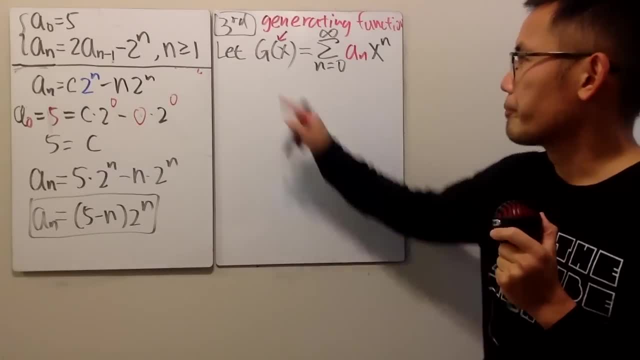 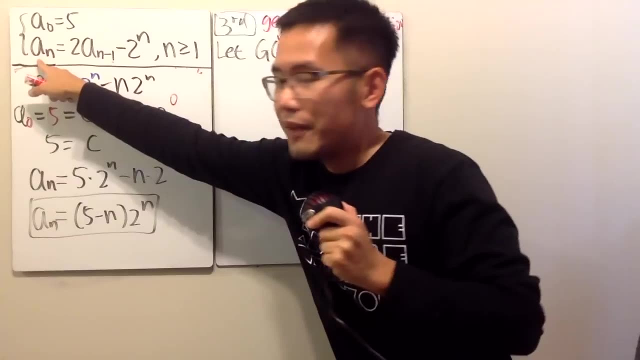 yeah, just do the math. that's pretty much it. so let g of x be equal to this, and of course we're talking about that and this is how we are going to do it. have a look. 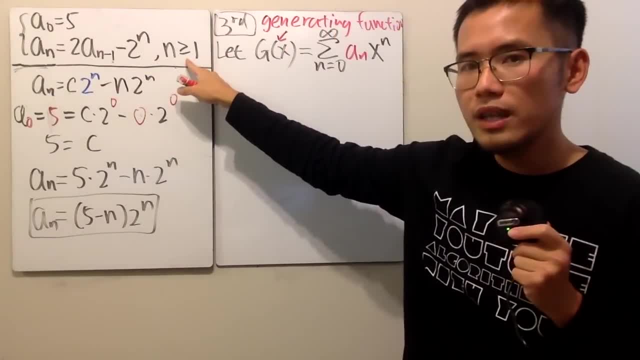 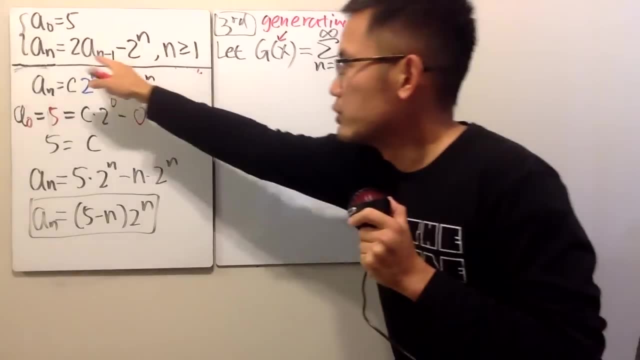 we have the an right here, but this is only good if n is greater than or equal to one. the generating function always starts with zero to infinity. keep that in mind, however, in order for us to use this. 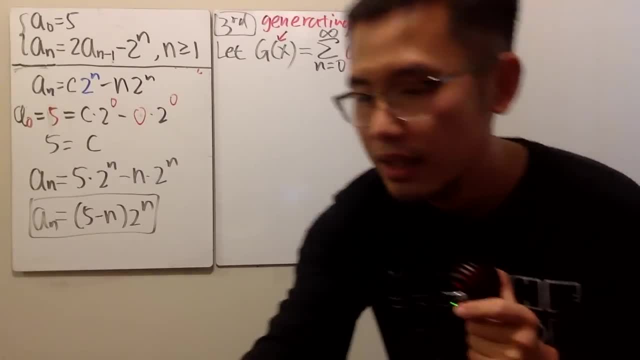 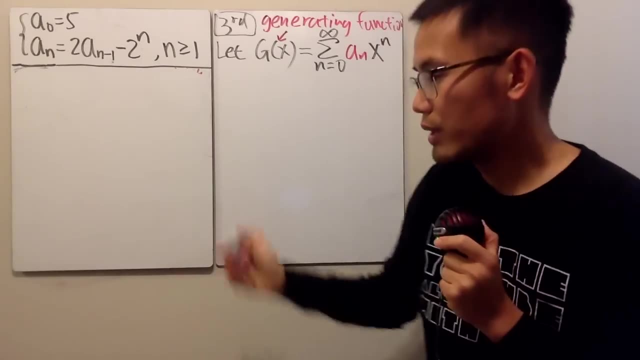 we can only from one to infinity right, and I'm going to erase all this and I'm just going to work out this right here for you guys. so here's the deal. I'm going to look at this. 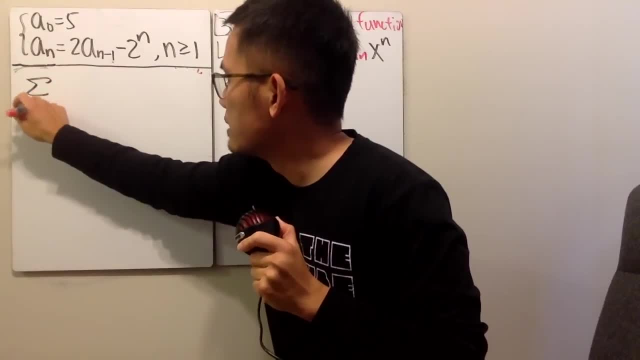 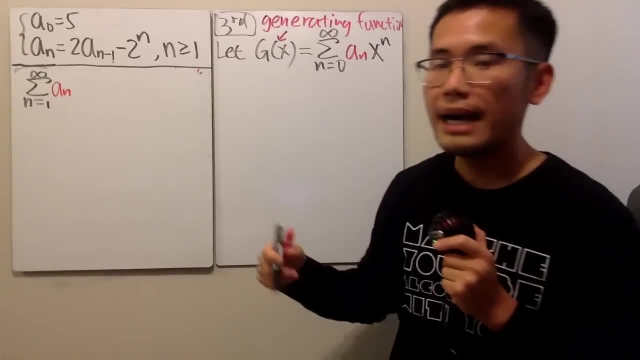 and I'm going to sum it up- from one to infinity. so have a look. here is the sum as n goes from one to infinity and I'm just going to have the an here, and again I will have to multiply by. 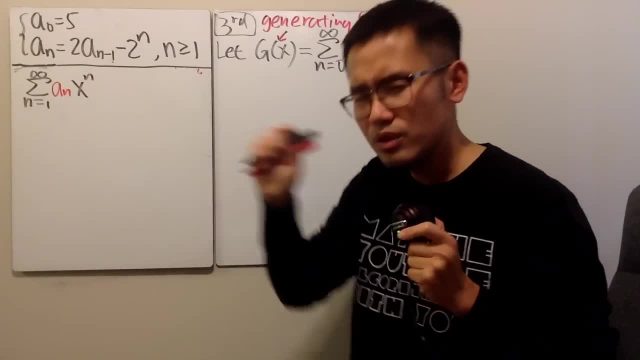 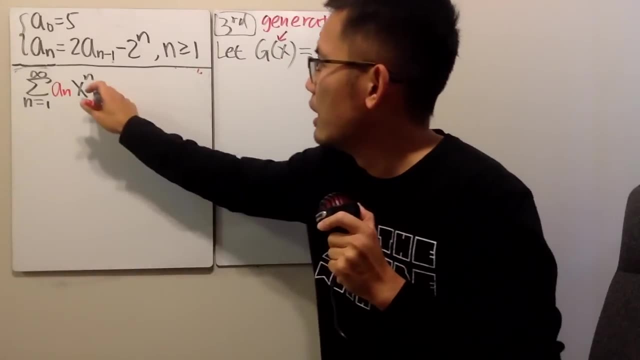 x to the nth power. that's the generating function. almost because this is at one, this right here is zero. we have to fix the index. you'll see anyway, because we're going from one to infinity, we can use this. 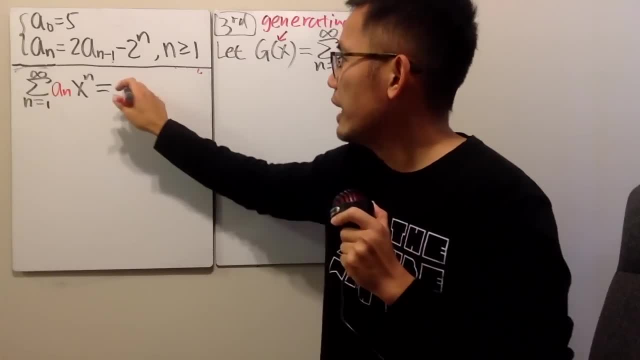 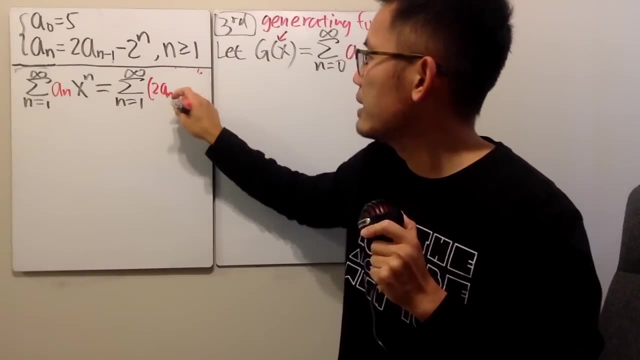 so I can just put this down right here. for the an, namely we get the series as n goes from one to infinity parentheses, this guy, which is two an minus one, and then we have the. 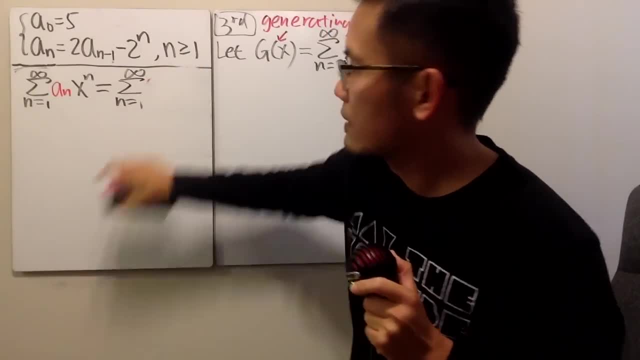 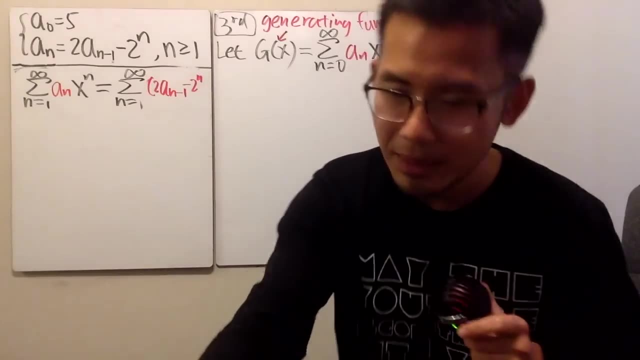 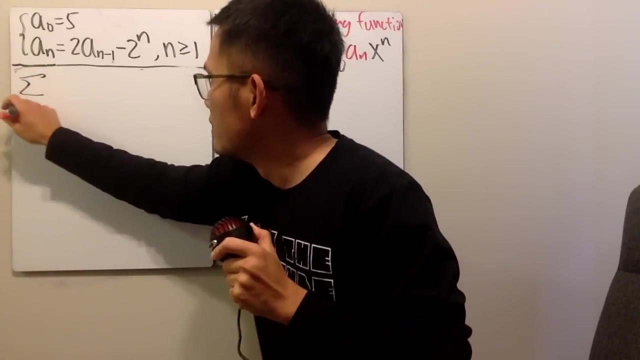 sorry. two an minus one minus two to the n. I'm. I'm so sorry. this it's just not. I don't have enough space. I'm so sorry. alright, let me write this down again. sum it up. 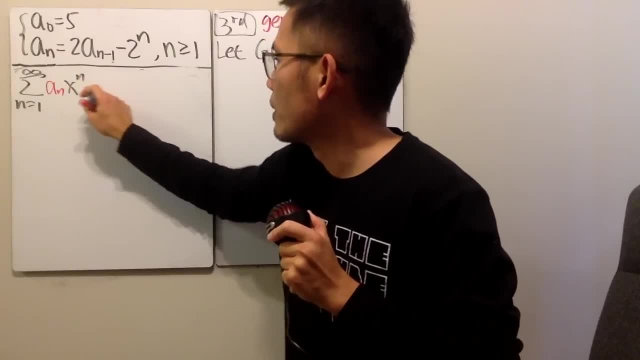 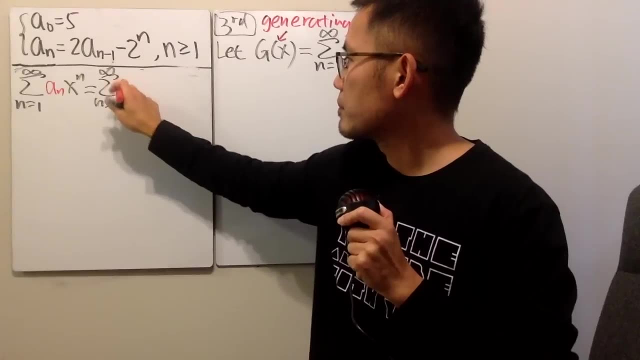 from one to infinity, an, and then multiply by x to the nth power. this is the sum as n goes from one to infinity. this, right here, I will just replace that two, an minus one minus two to the n. 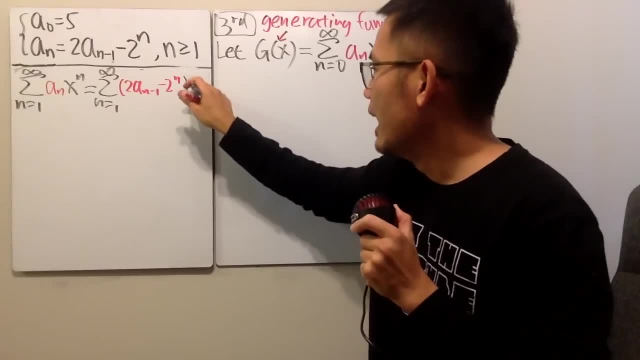 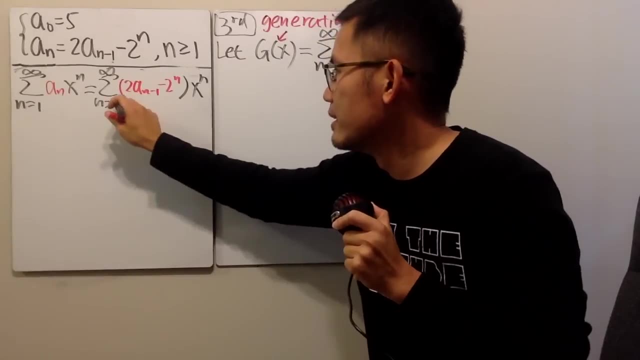 then. this is not eta, this is n alright. n times x to the nth power. this is not h, this is n alright. alright, anyway, just go ahead. just change that now. what we can do next. 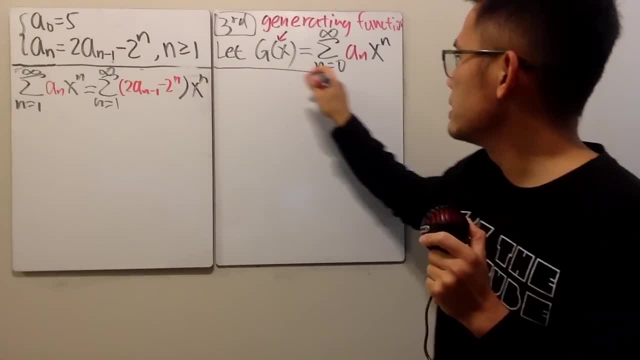 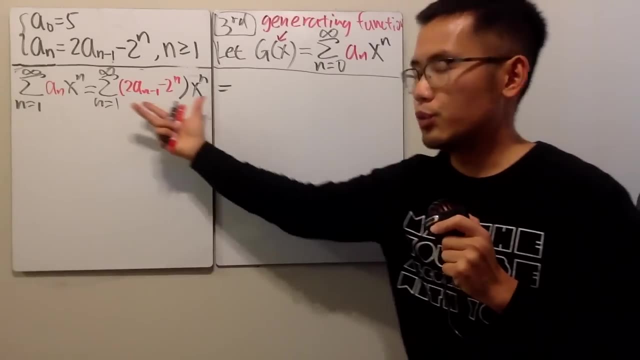 is that we are going to fix this and this is how. so keep this in mind. this is the third way. just keep that in mind. well, I will have to come here because I have to work this out. 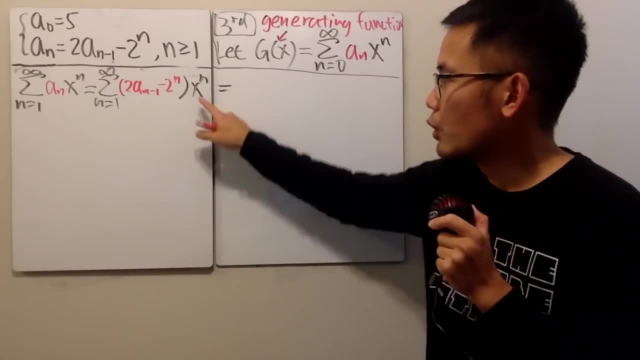 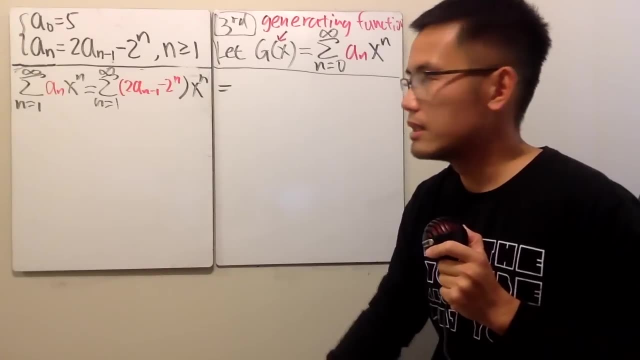 the way that we are going to do this is that we are going to fix the power right here. I want to have x to the n minus one. I will just take out one of the x because eventually, 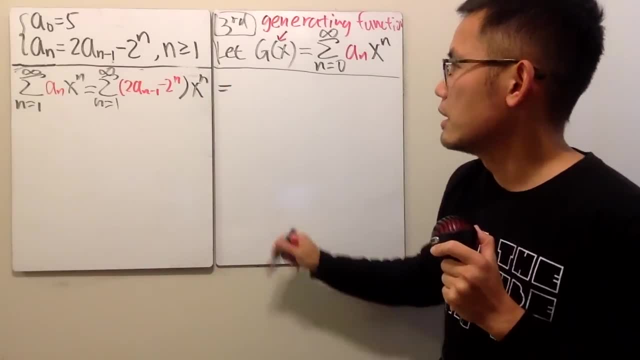 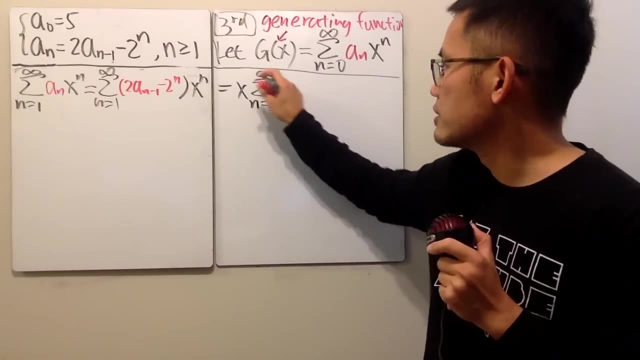 I want to fix the index here, so fix the power first. so I will have x times. the series n goes from one to infinity. this still stays the same. and then the rest right here, still stays the same. 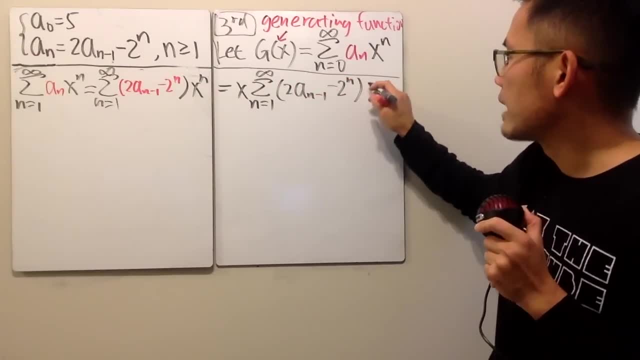 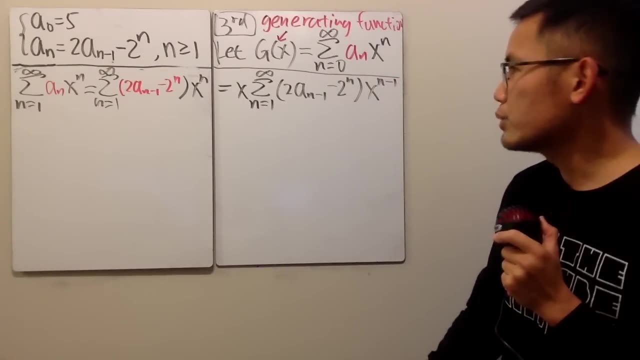 so we have two: an minus one minus two to the n times x, but this right here, is n minus one power. now, right then. what we are going to do next is that, right here, I am going to add one. 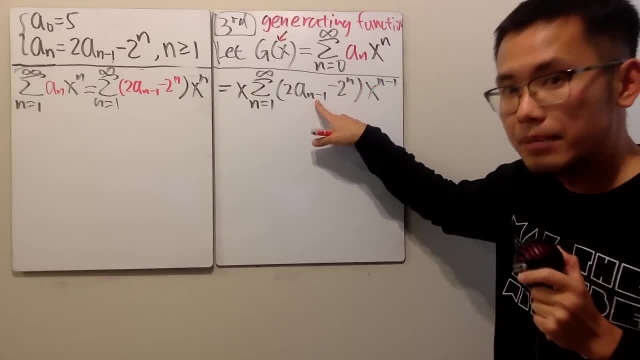 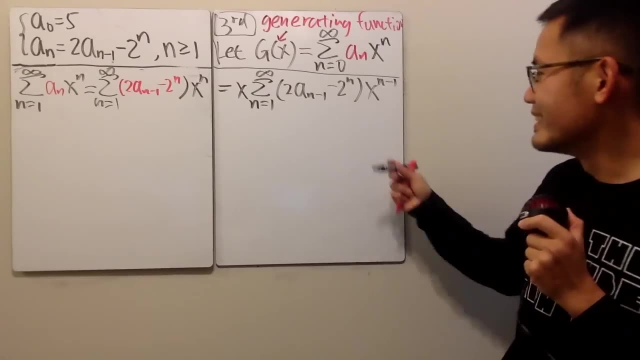 to all the index right here. in the meantime, all we have to do to keep this balance is just minus one here, minus one there. that's the idea. so, as you can see, this is x and then. 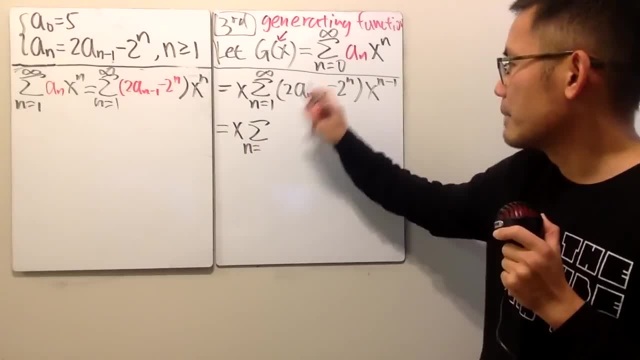 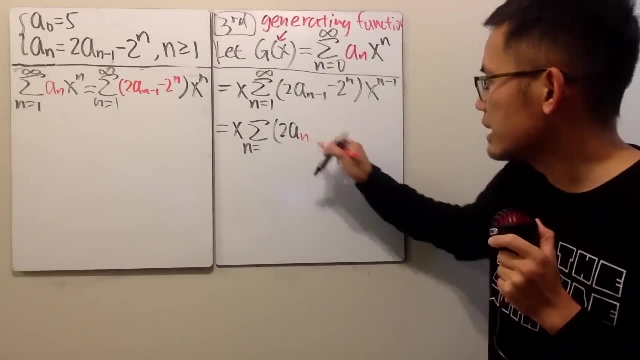 this is going to be n going from something to something, but again, let's do this in order. I will have two: a add one here, so it becomes just n, and then minus two- add one here. 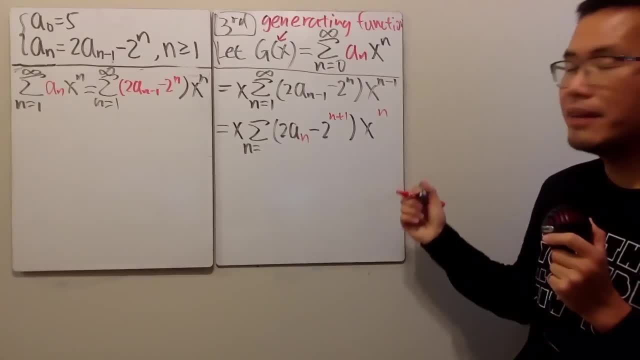 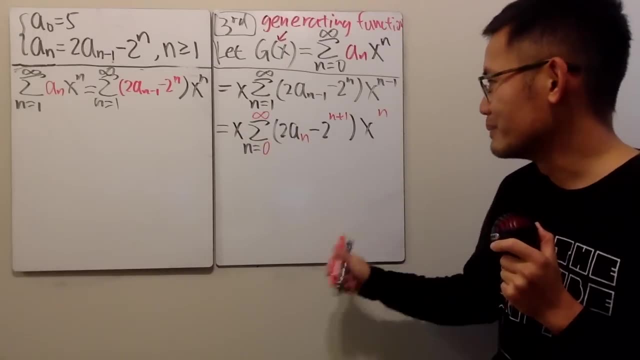 is n plus one times this is x to the nth power. now, right and again, here we have to: minus one. minus one, which is zero, and infinity minus one is still infinity. now you can see that. 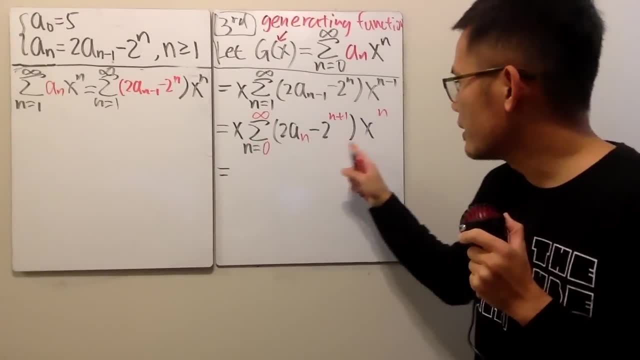 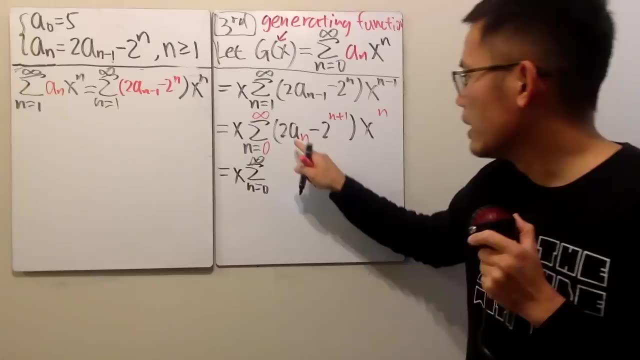 I can just multiply things out and all that stuff, and right here I will have x times the first part, which is the sum from zero to infinity, and I have two right here, right? so perhaps? 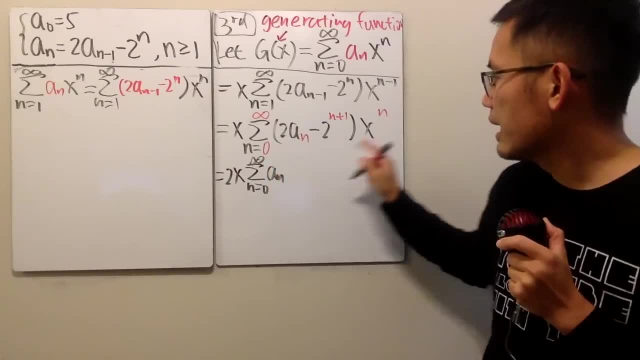 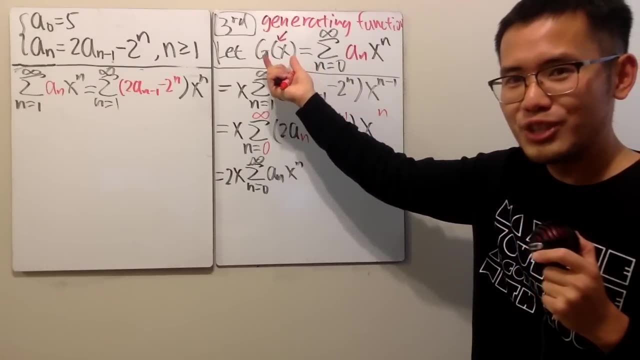 I will also put down the two in the front. and then here we have the a, n and then x to the nth power. what's this? yes, this is precisely our g? f, namely generating function. good, 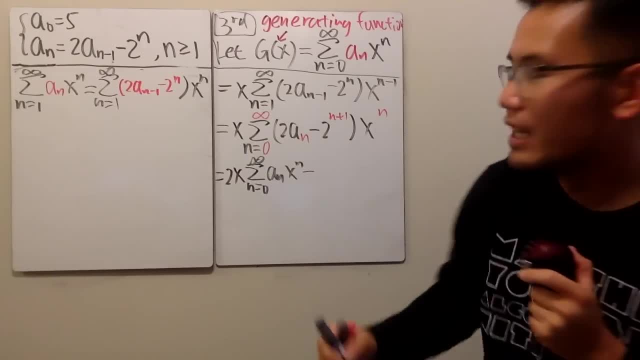 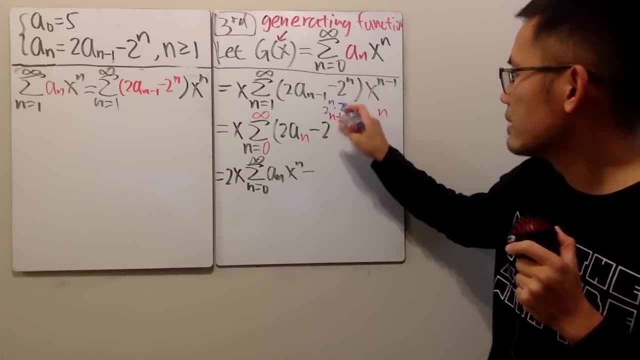 now minus well, be really careful with this. you see, here we have two to the n, plus one, well, of course, and we can just put the two in the front as well, so I'll put down the two. 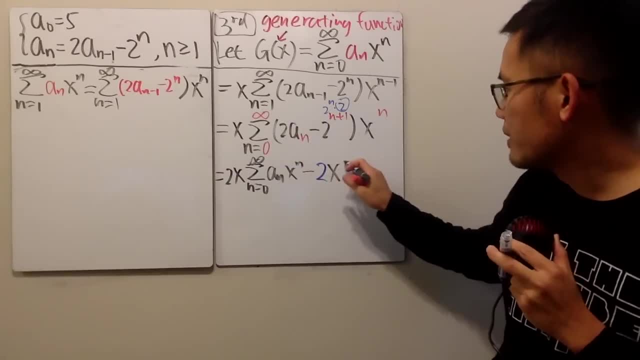 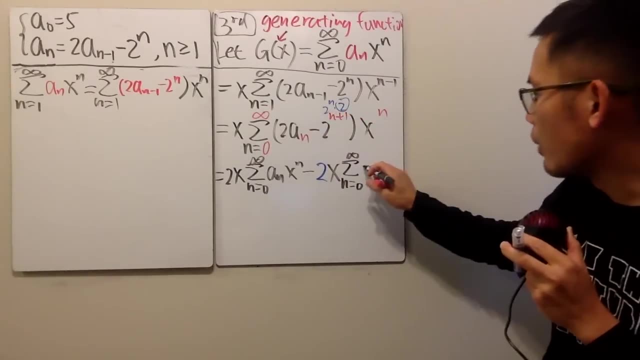 right here first, and then we have this x, and then we have the series as n goes from zero to infinity. then for the inside we will just have two to the nth power, times x to the nth power. 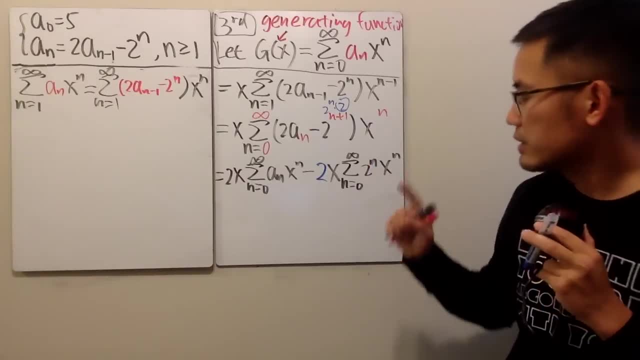 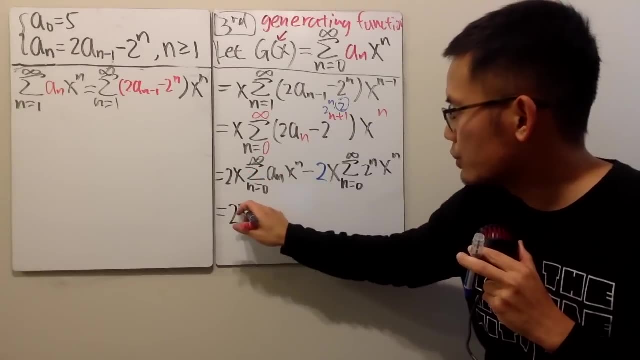 like this very good, and you'll see why I want to do. I want to do this in a sec, but anyway, this is what we have. and then, on the, this is two x and again. 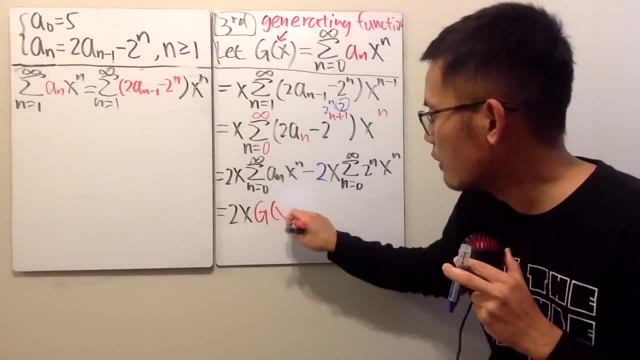 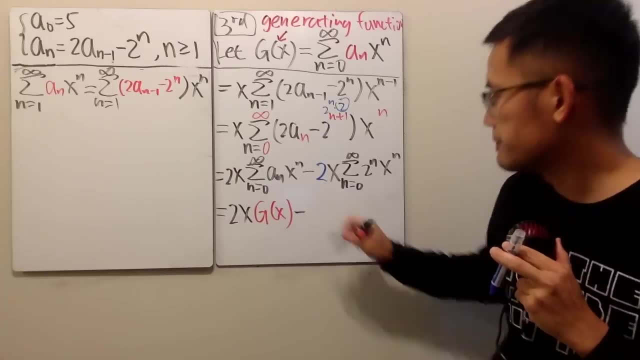 this is our generating function, which I will just write it down as g of x. right, this is from that. then, right here we have minus this. right here is still our two x, but what's this? 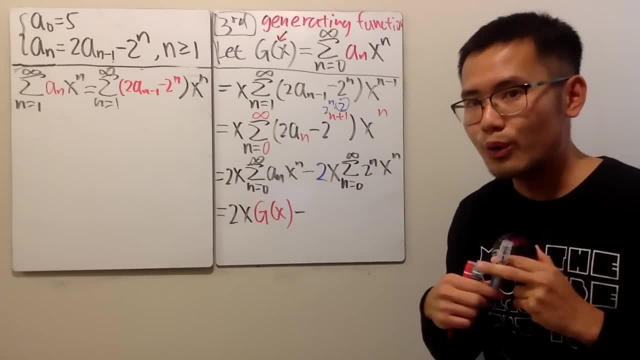 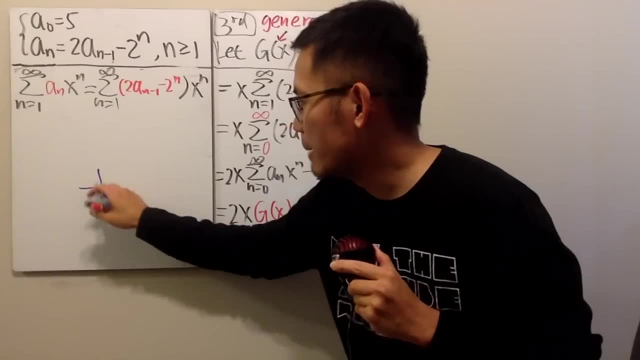 of course you can write this: two x in parentheses, raised to the nth power, and that should remind you of our best friend. let me remind you guys right here, when we have our best friend, namely one over one minus. 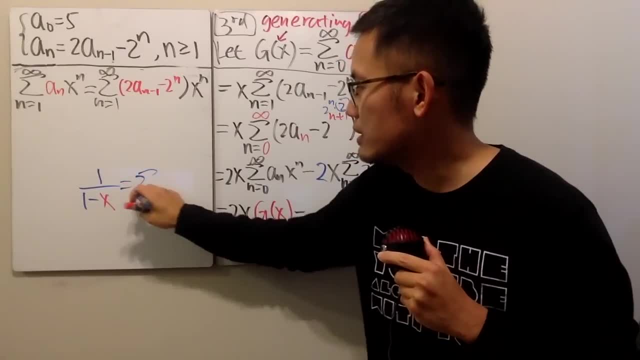 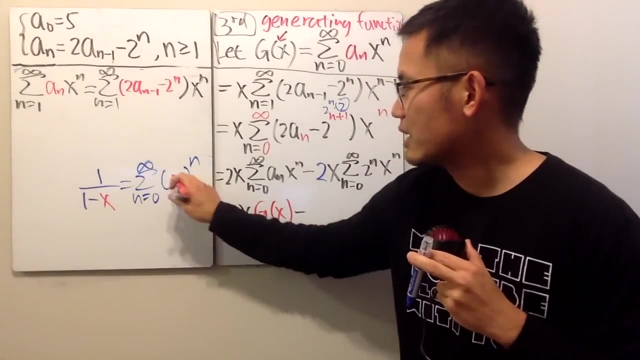 x. this right here is nicely equal to the series, as n goes from zero to infinity of something to the nth power right. all you have to do is put the x right here, that's all. 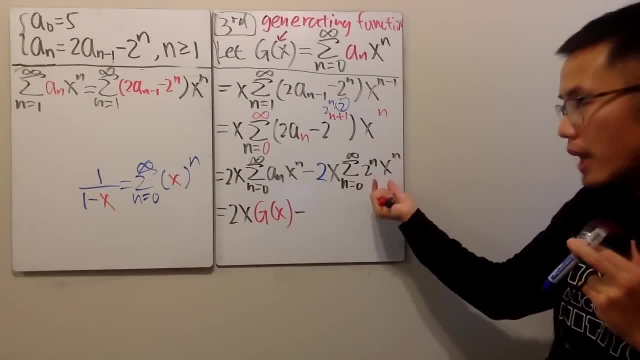 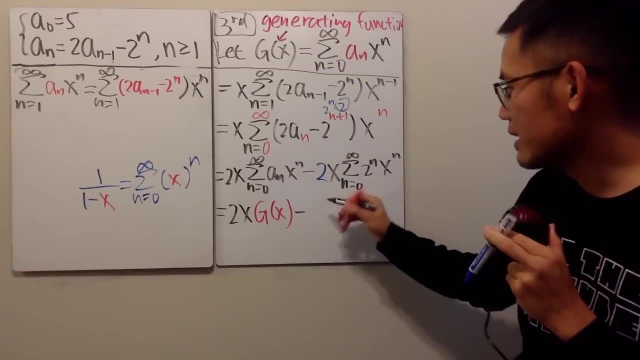 now we just have to go backwards, so the two x will be the input. we just have to put it here, and then we have another two x here. so all in all, we have to just have the two x on the top. 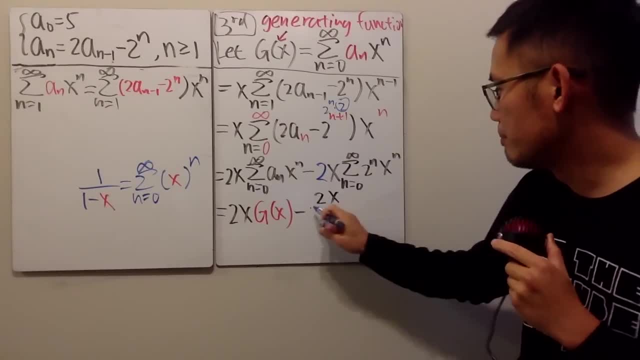 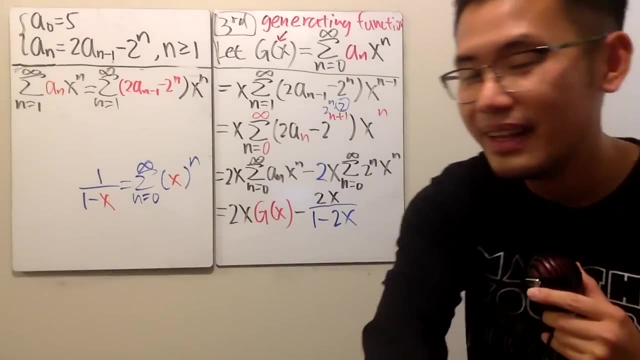 let me just write that down right here for you guys. and then over one minus, again two x, like that. very nice, right. so now this is all good, but we should also be. 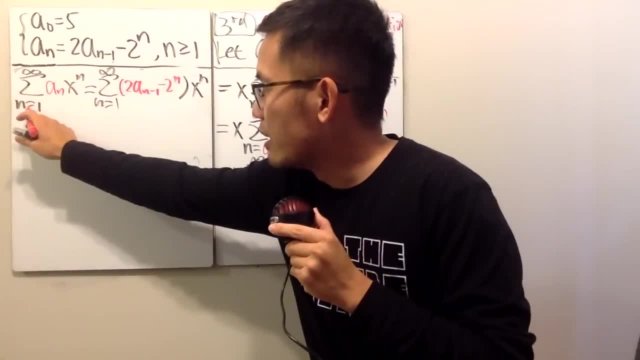 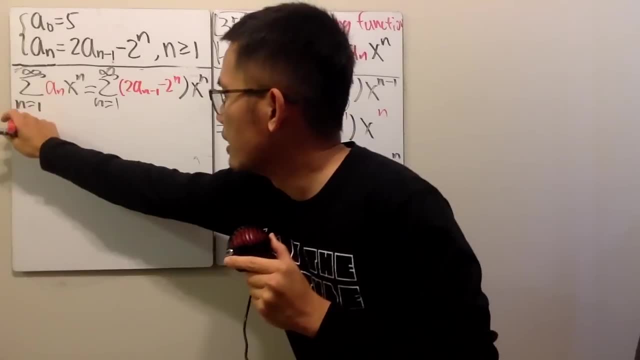 fixing this as well. have a look. this right here goes from one to infinity. I really want to go from zero to infinity. this is okay, let me just go ahead and do this. I'll just rewrite it. 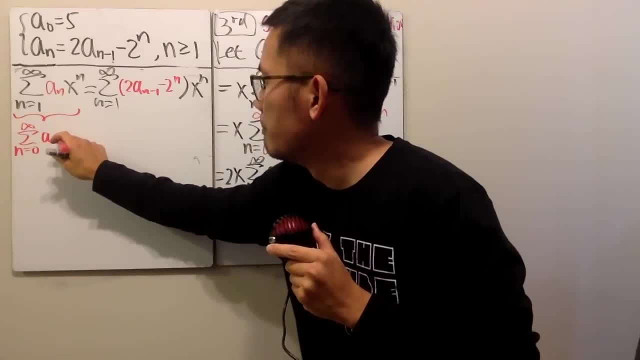 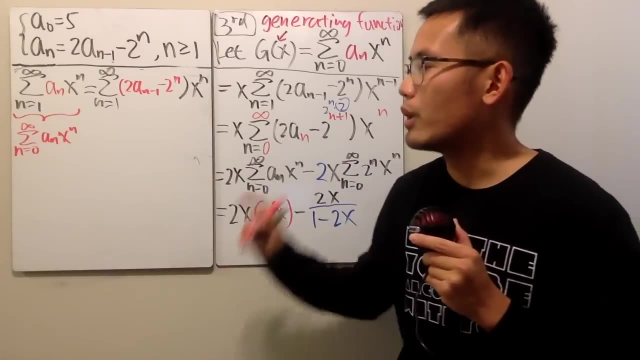 as n goes from zero to infinity, of a n times x to nth power. that's okay, but I cannot borrow one number and that number is precisely our: a zero right, I just add a zero here. 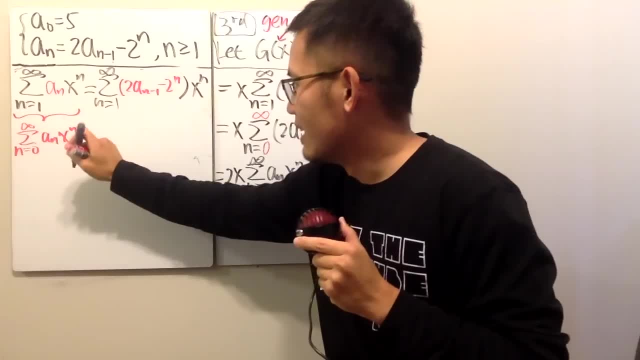 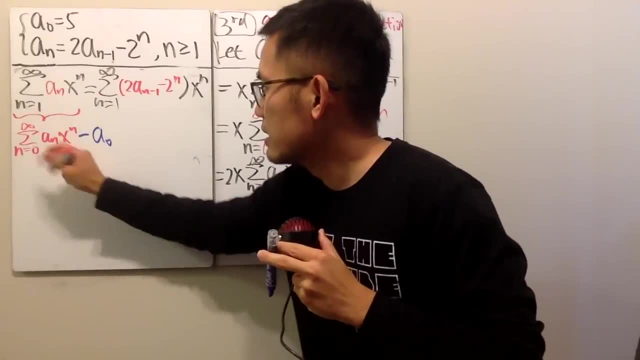 but of course, if you add the a zero, just go ahead and minus a zero so we can keep that to be balanced. and we do know what a zero is. this is the same as that, and you know. 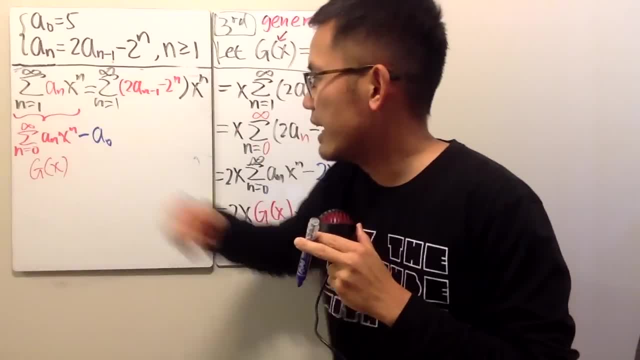 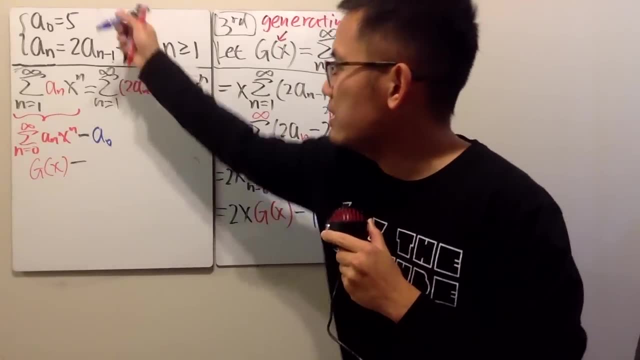 this is our generating function. so this right here is g of x, and then we can just go ahead and minus- the minus should be in black minus and the a zero is five. and now have a look. 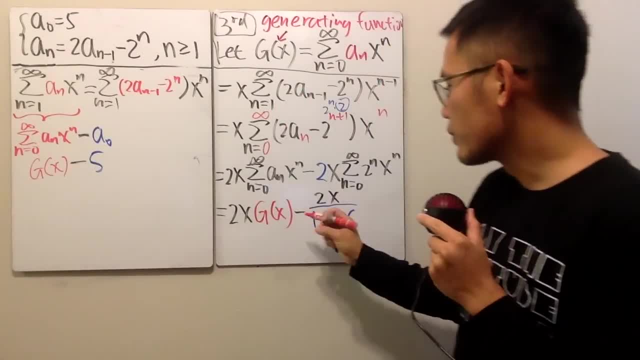 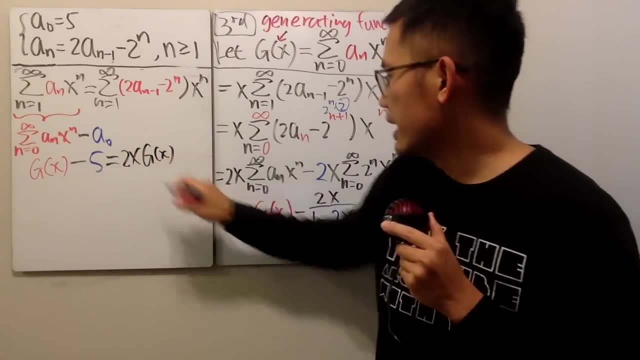 the left hand side is just g of x minus five, and then, of course, on the right hand side we have this, namely two x g of x, and then minus two x over one minus. 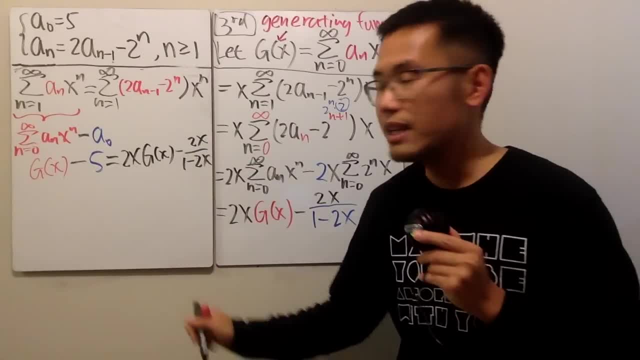 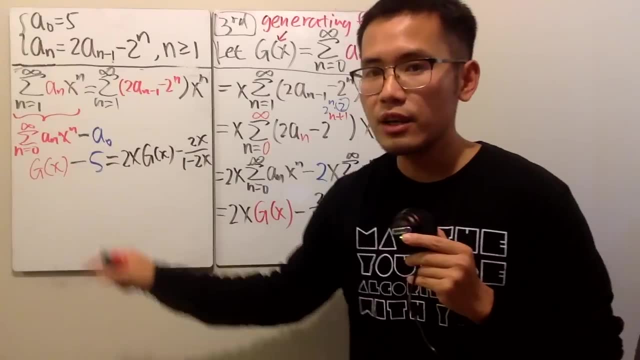 two x. I just have to bring this to the other side, and the reason I want to do that is because I want to solve for g of x is. so now let's go ahead and do that. 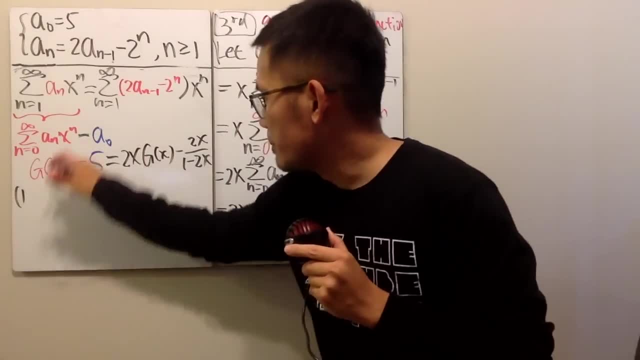 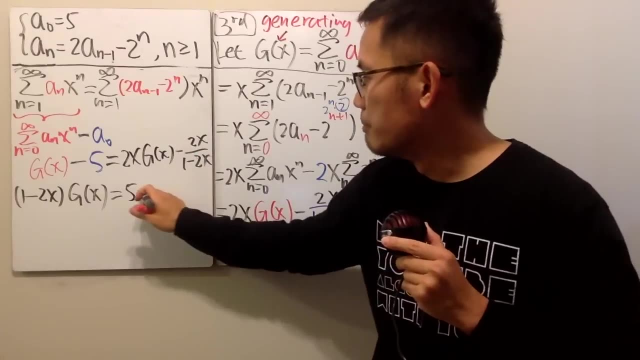 bring this to the other side and factor out g of x. let me just write it as one, and that becomes minus two x, and then we have the g of x right here, and then I'll have the five. 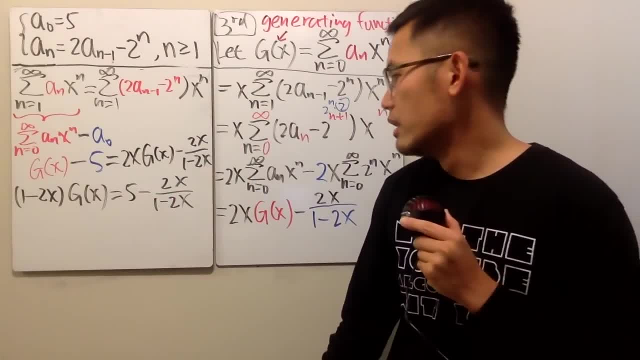 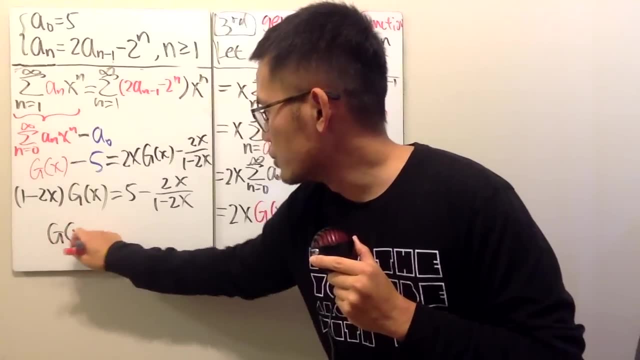 right here, minus two x over one minus two x, like that. right then, of course, we can combine the fractions. so combine the fractions. I need to have one minus two x as its denominator. 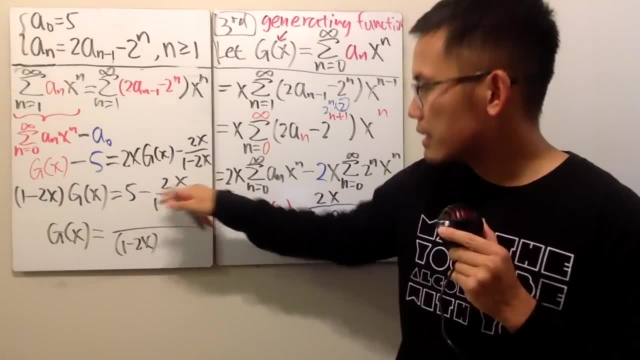 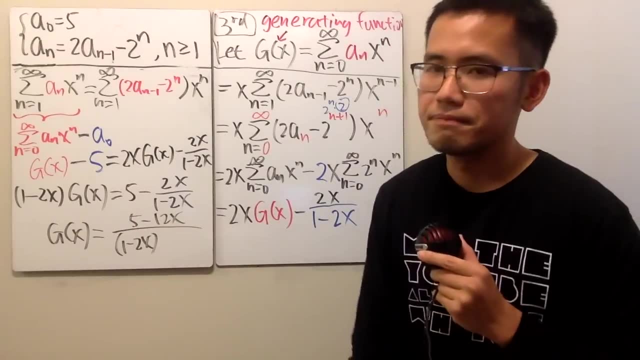 and, of course, this times that which is going to be five minus ten x and then minus another two x on the top. I have five minus twelve x, and then divide this to the other side. it's the same thing. 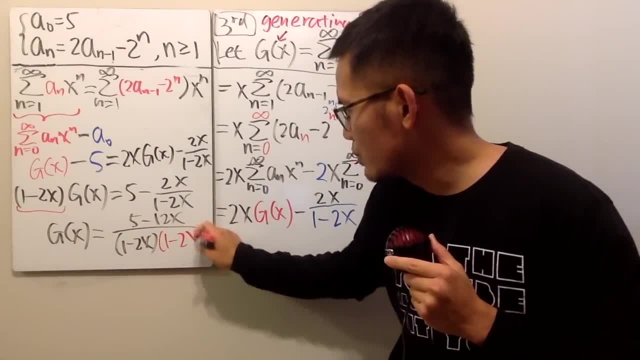 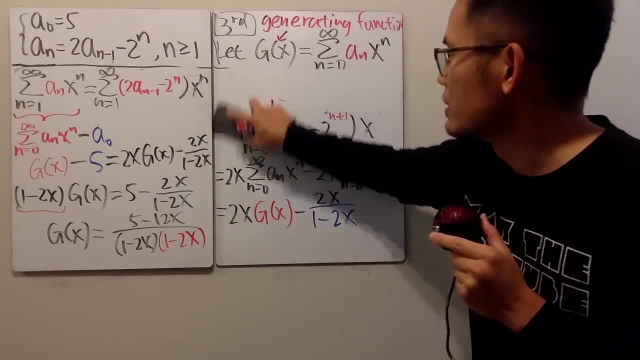 huh, this right here is one minus two x. things are going to get a little bit weird, you will see. keep this in mind. g of x is equal to this right, and I'm going to erase. 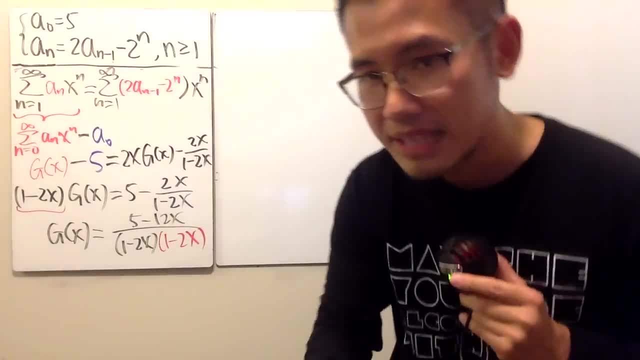 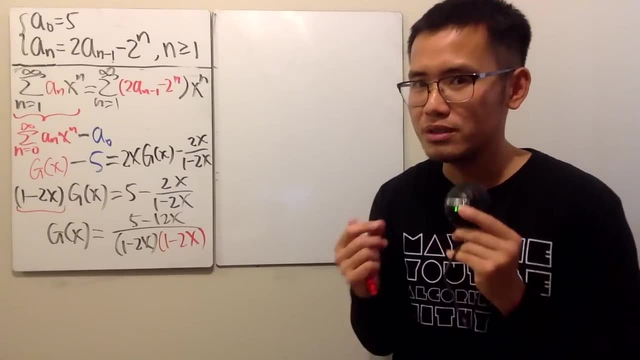 this part and the goal is that this. right here we have a rational function. if we can write this as a power series, we can just mix the, we can just mix and match the coefficient. that's the approach. 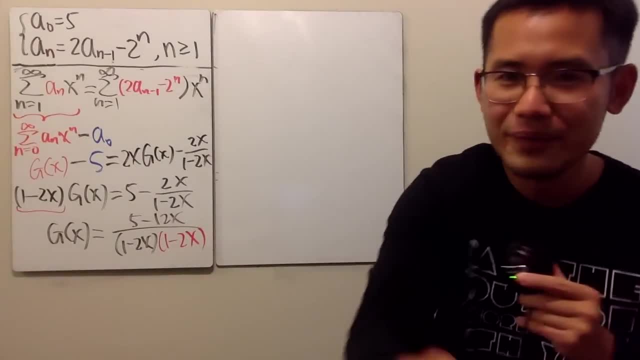 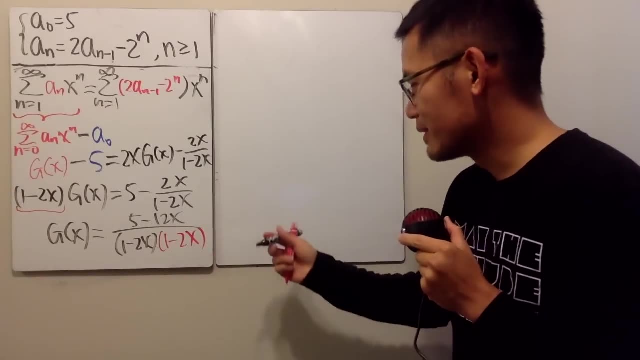 right. so here's the deal. oh man, I am going to break this down. it's not so bad. have a look. okay, so it's not so bad. have a look. g of x. 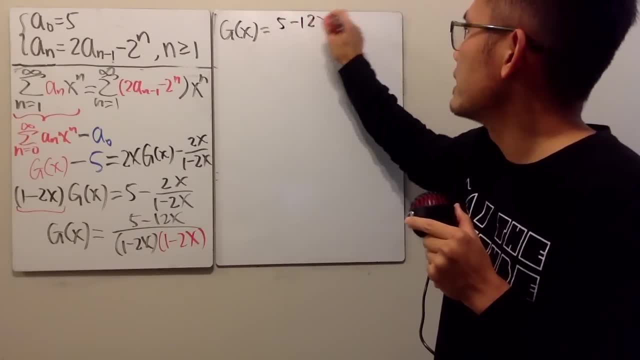 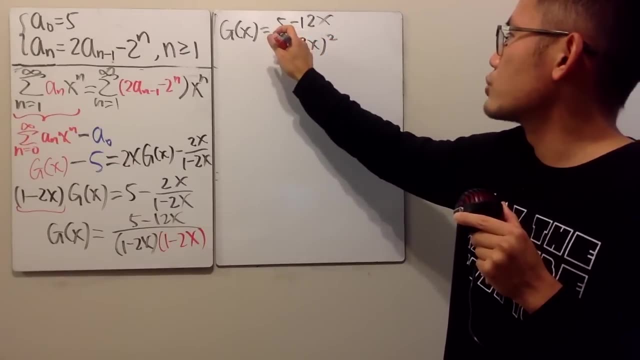 this right here is equal to: on the top, we have five minus 12 x over. of course, the bottom is the same as saying one minus two x and then square. you can try to do this. 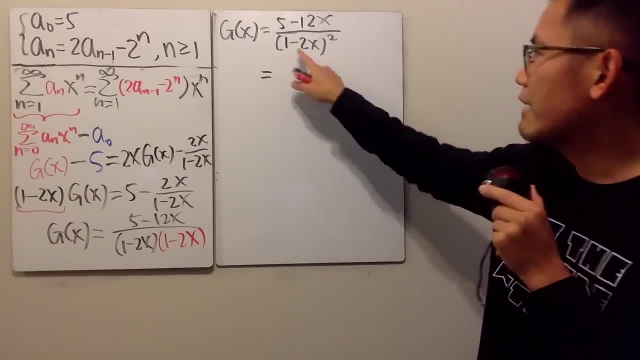 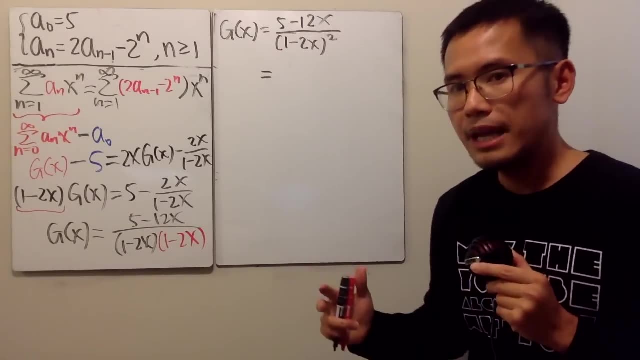 by partial fraction. or you can also just do the following: have a look on the bottom. here we have one time one minus two x, right, one minus two x on the top. wouldn't it be nice? 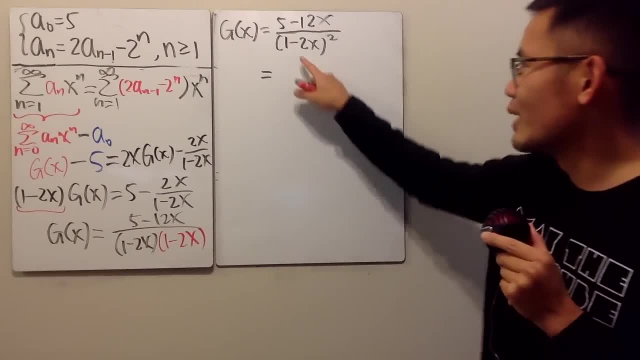 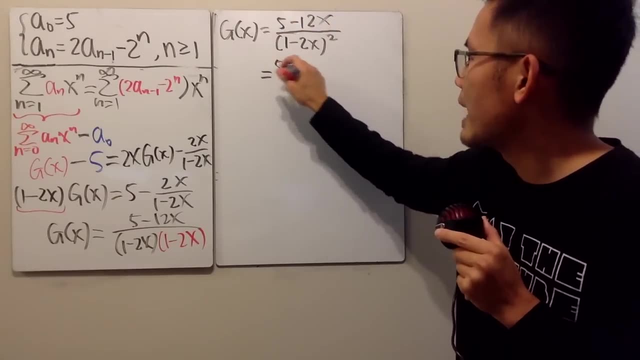 because we can factor out the five and then we can cancel out the one minus two x part. so for the top right here I'm going to write that as five minus 10 x, and then, of course, 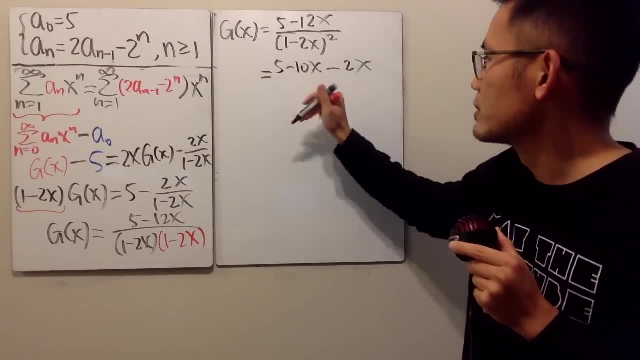 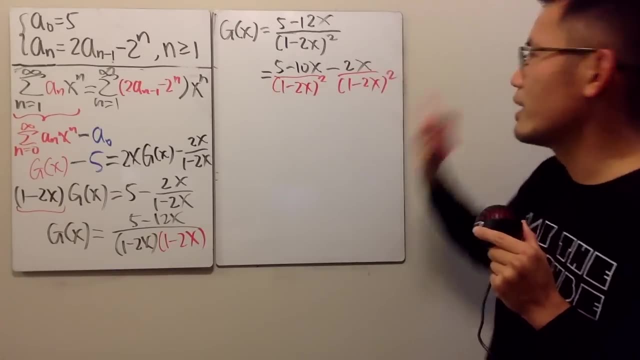 after that minus two x, and then you see, I will just go ahead and divide this by one minus two x square. likewise, one minus two x square. like that, factor out the five, divide out. 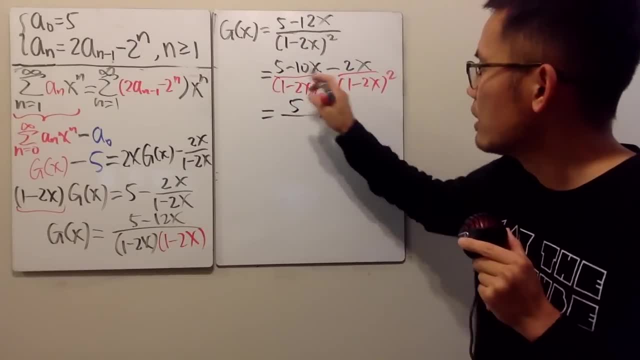 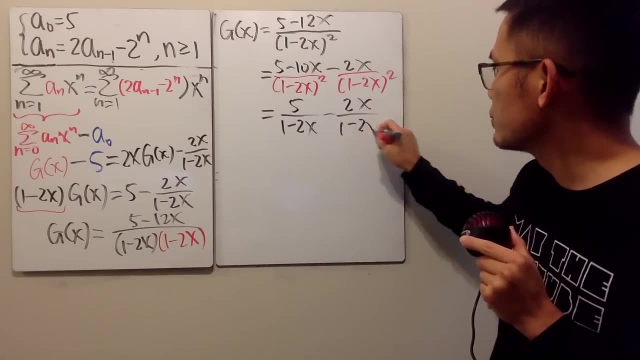 then you see, the first part is five over one minus two x. that's it for the second part. we have minus two x over one minus two x and we have to face this. 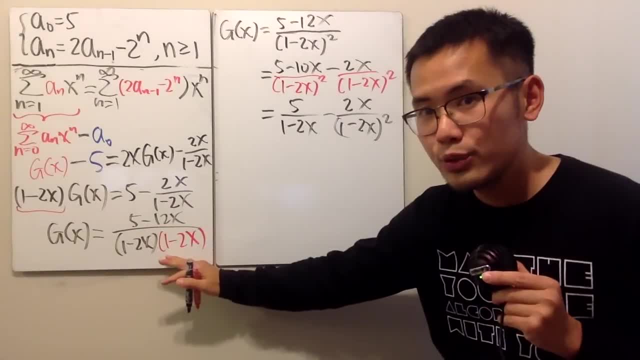 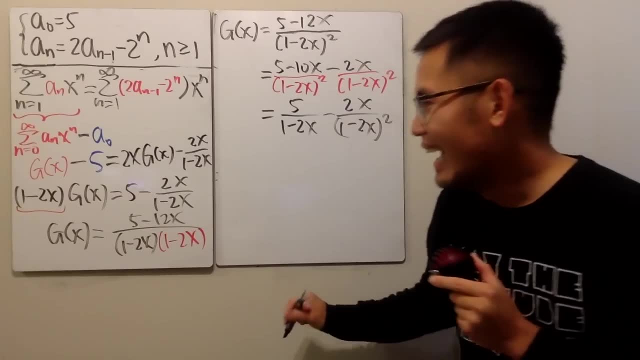 this right here, not so bad again. we are trying to go back to the. we are trying to go back to the infinite series form. so, yeah, anyway, this right here. use the best friend. we have the five. 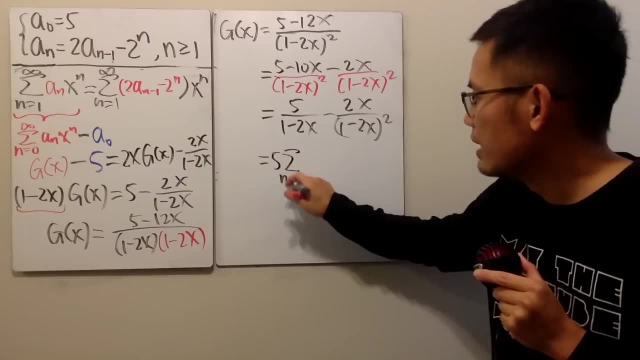 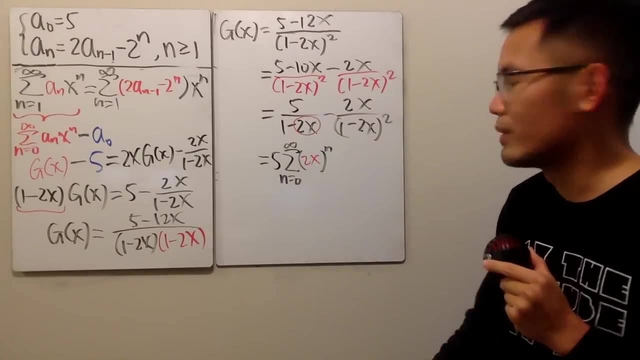 yeah, so put that on our side. and then n goes from zero to infinity. here is the input. I will just put down the two x here, and then to the nth power. that's it, best friend. 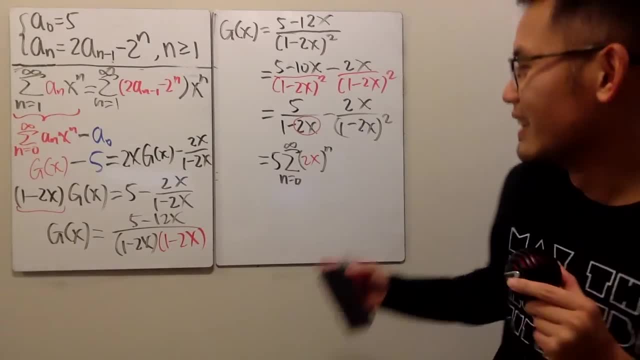 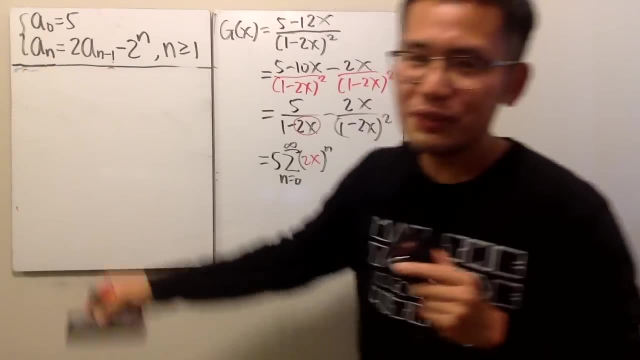 always is the best. trust me on that. now for this, though, hm, we will have to utilize other friends. you still have to use your best friend, namely it's derivative. so you'll see, because, on the bottom, 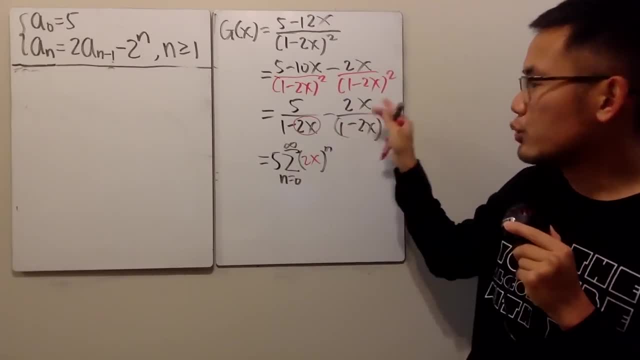 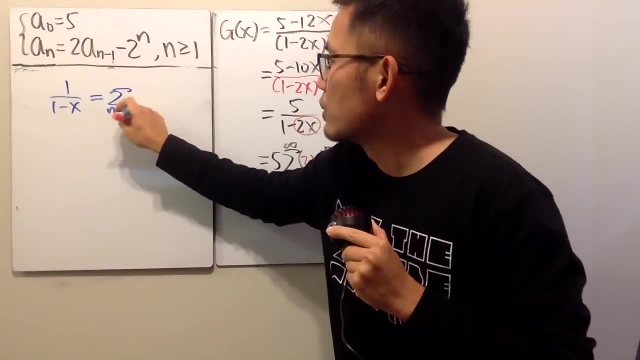 you have this and then you have this square again, the two x. just forget about that for now. have a look here. we know that. one over one minus x. this right here, it's the sum as n goes from zero. 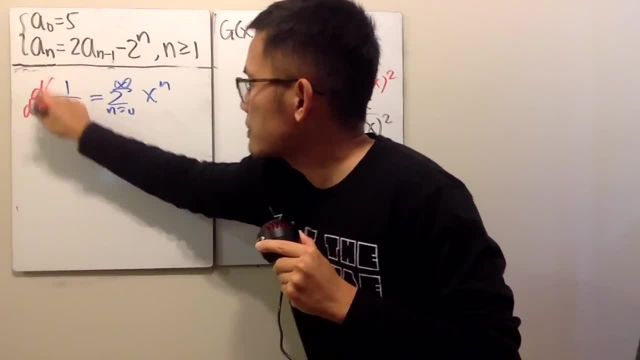 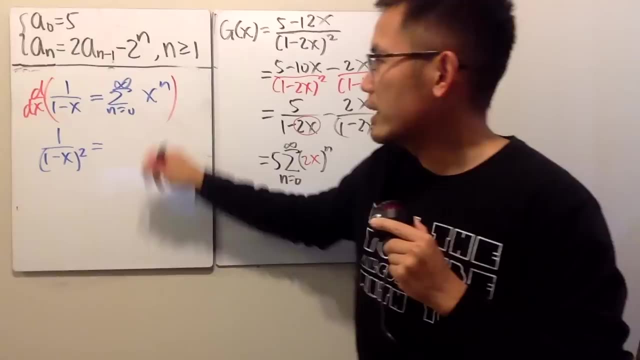 to infinity, x, to the nth power. and if you differentiate this on the left hand side, work out your derivative. trust me, you get one over one minus x. and then square the right hand side. you put the n to the front. 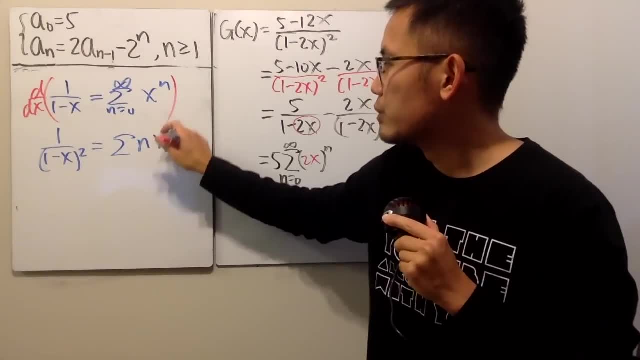 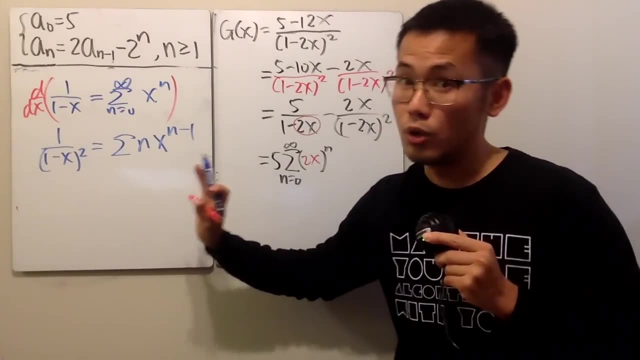 and then minus one. and here's the deal: you get minus one. but if you have n is start with zero. well, the first term would be zero, so it's not needed. you can just start with. 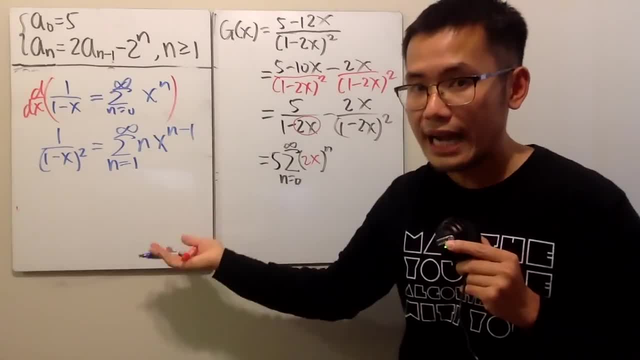 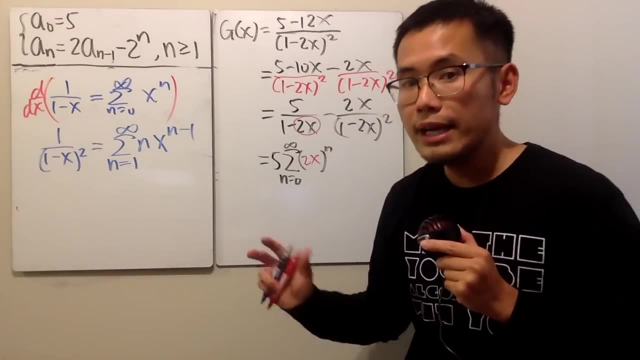 n is equal to one and then to infinity, so this is equal to that. and I did not forget about my chain rule. it actually is positive. I can go ahead and check out the differentiation, but again, we'd like to have: 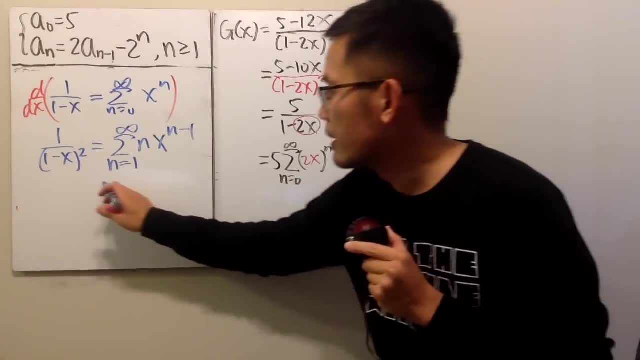 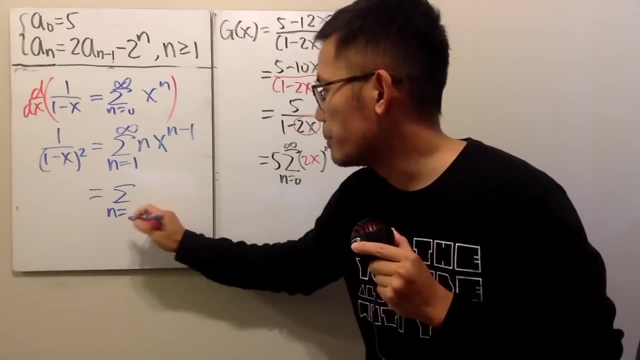 n start with zero. so we do the same trick as what we did earlier. this right here, I will add one. add one so I can subtract one. you see we will get. n will be going from zero. 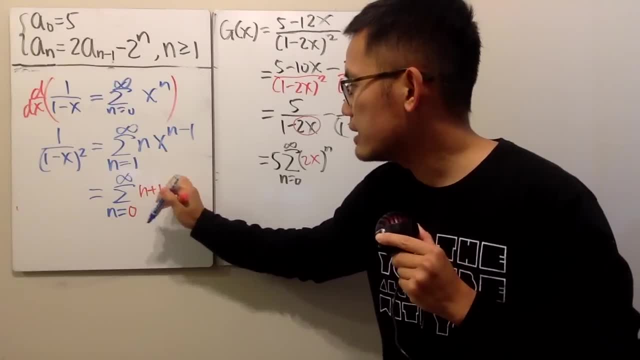 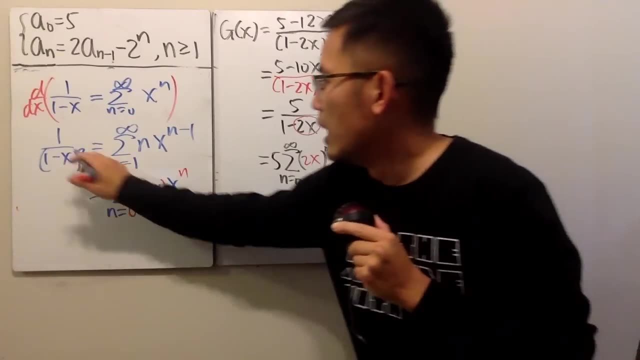 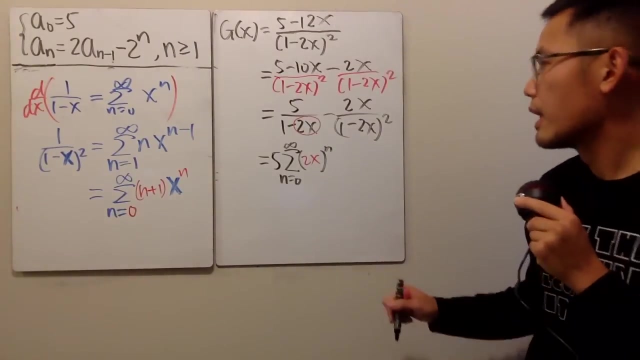 to infinity, and then n plus one, and then x to the nth power. that's what we want. now have a look. this right here is our input, right. so here's the deal, right here. 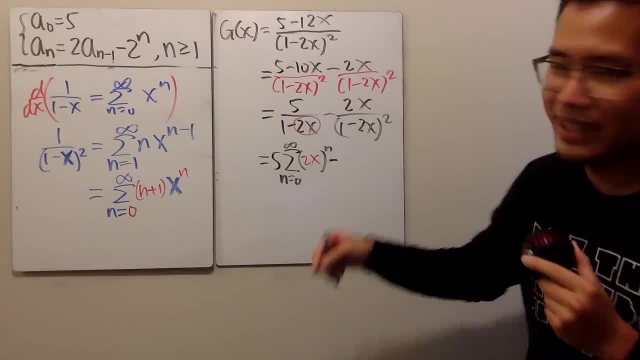 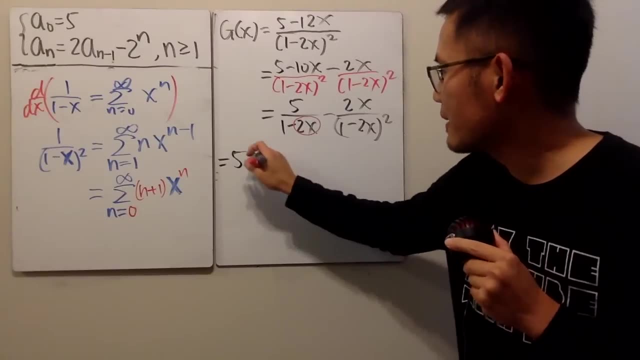 I have the minus two x. okay, I don't have enough space, alright, let me just write this down right here. I have the five and then sum as n goes from zero to infinity parentheses two x. 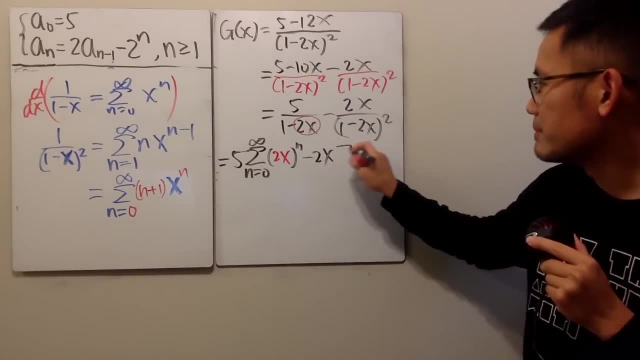 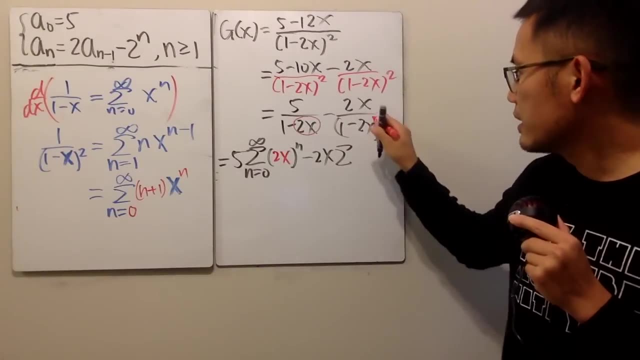 to the nth power. okay, minus two x times one over this, which I will just plug in. the two x right here is the input. plug in two x in here so I get the sum. 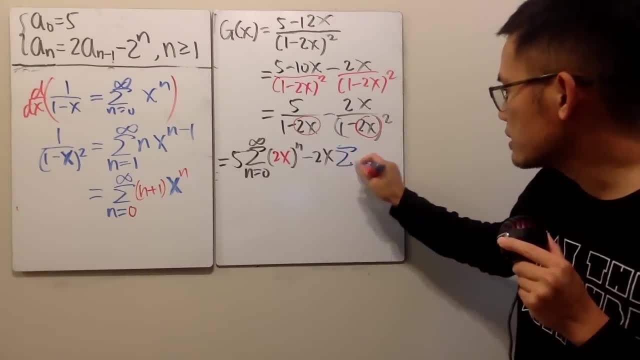 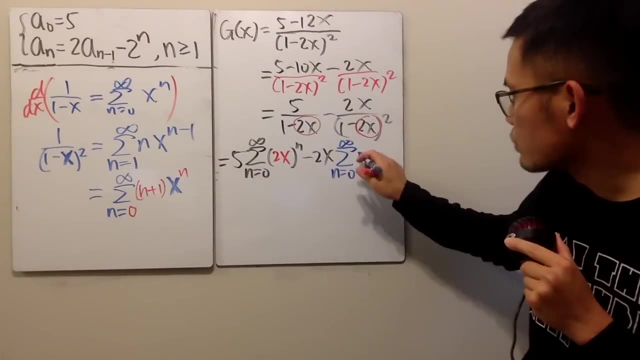 which I should put this down in blue, just to make it stand out for you guys. here is the sum which, ever way you want to call it, n, goes from zero to infinity, and then n plus one, and here we have. 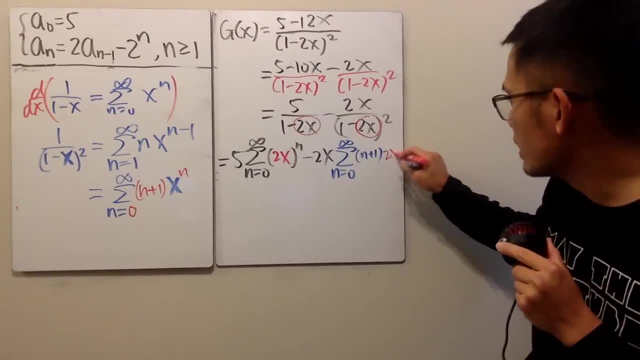 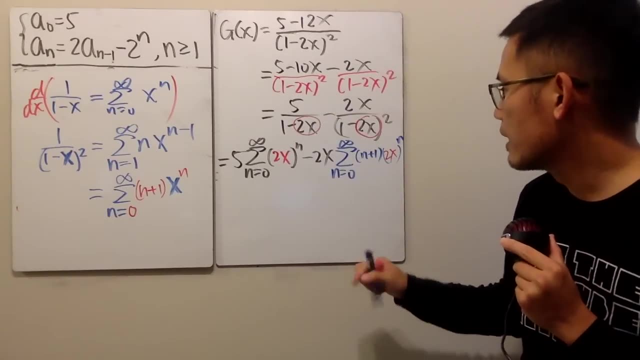 the two x, so be really careful. we still have the two x here. then you raise that to the nth power, like that. alright, so that's what we have now. we have the two x and this is also two x. 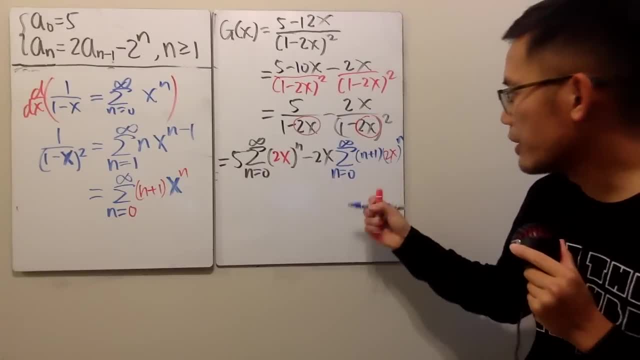 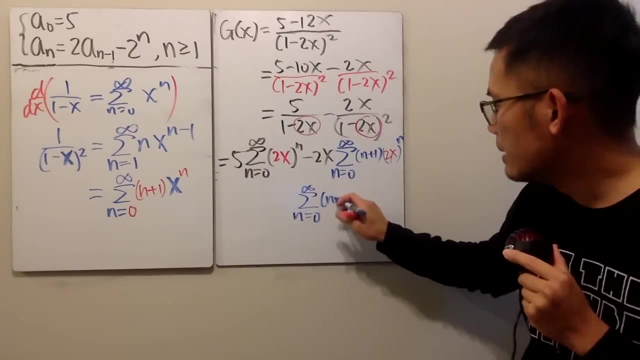 to the nth power. so of course we can fix the power here. so just focus on this right here. you see, n goes from zero to infinity, n plus one, and then this is two x to the. 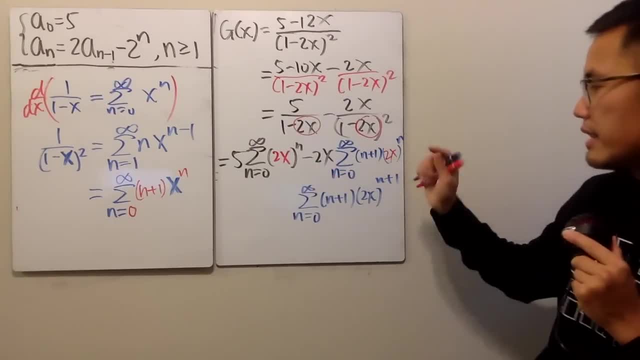 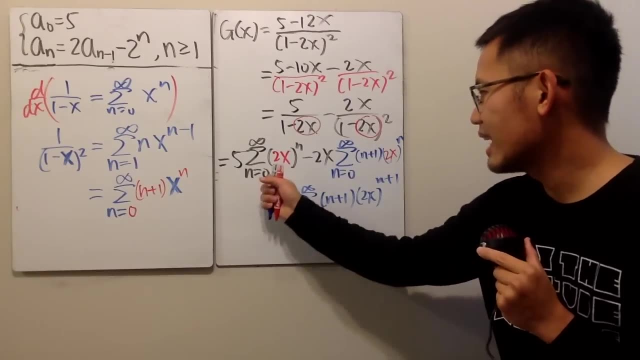 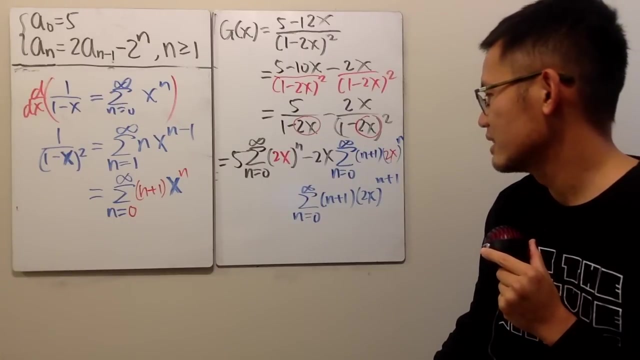 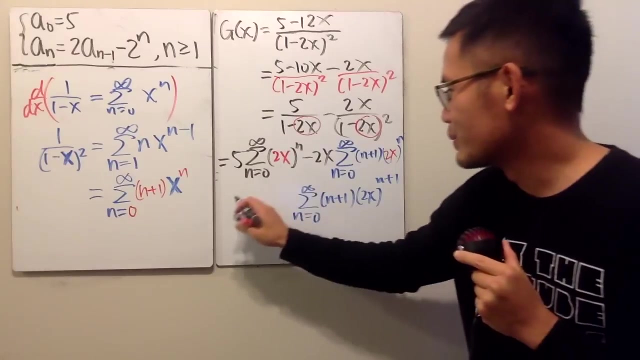 n plus one power, because I bring this inside and that's what we have. there's a problem, though? I cannot combine the infinite series. well, don't worry, fix the index, fix the n again. let me just write this down. 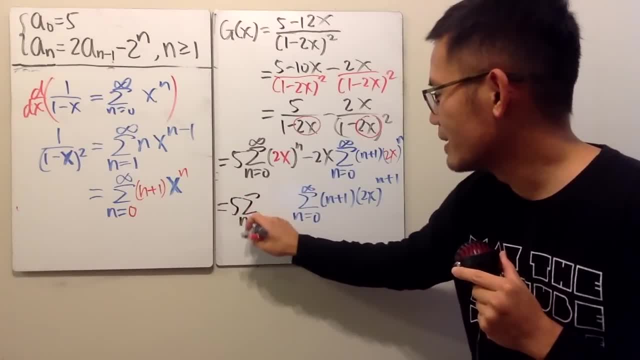 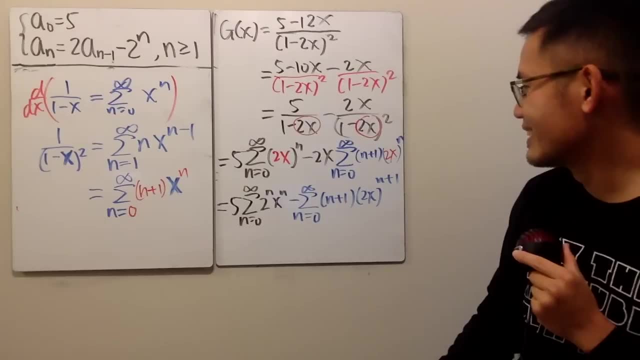 for you guys five, and then the sum n goes from zero to infinity. perhaps I'll just write it as two to the n, x to the n, and then this is minus, of course, right now. 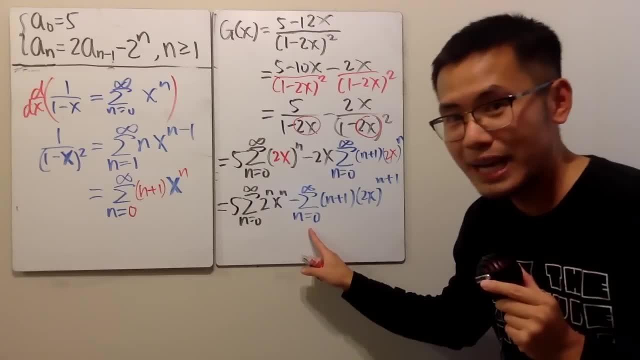 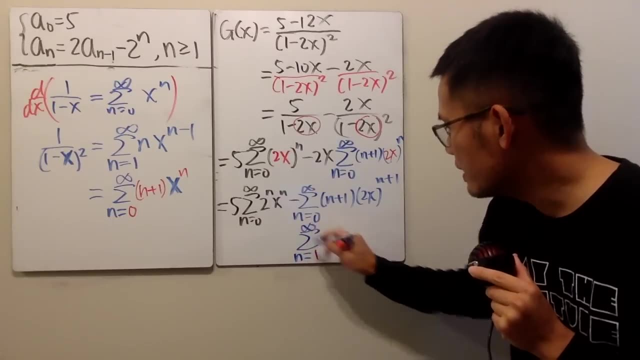 this is what we'll do. right here, I'm going to minus one, minus one, so in that case I just have to add one here. so focus on this. you get a sum, or the series n goes from. 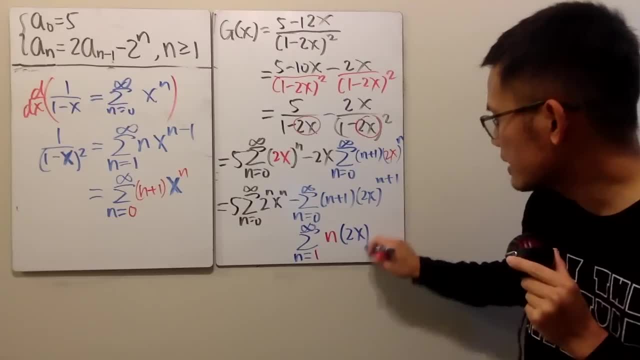 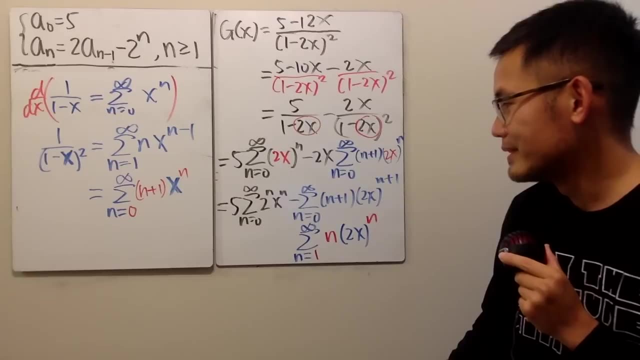 one and this becomes two x to the n's power, like this. so this right here is the form that we have, but again, the problem is that this and that they are not exactly, 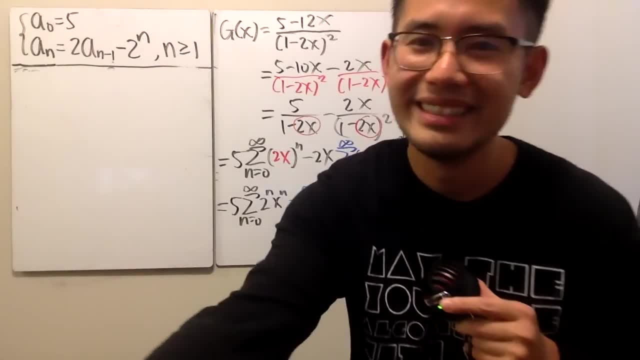 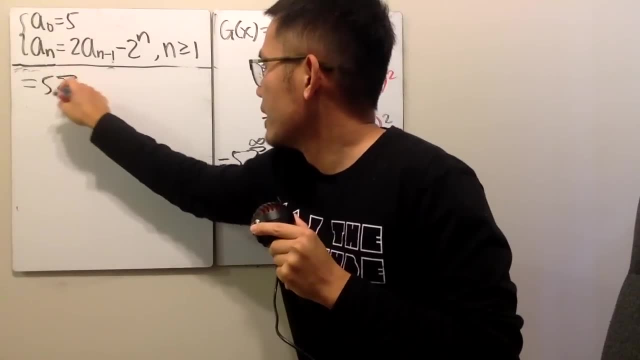 combinable at the moment, but I can make it happen for you guys, as long as we just do it carefully. anyway, this right here is equal to five times the sum. n goes from zero to infinity, two to the n. 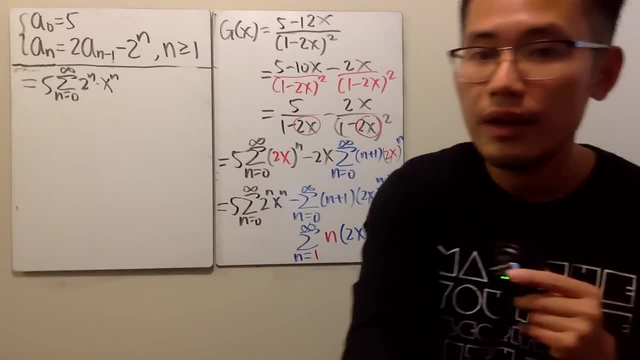 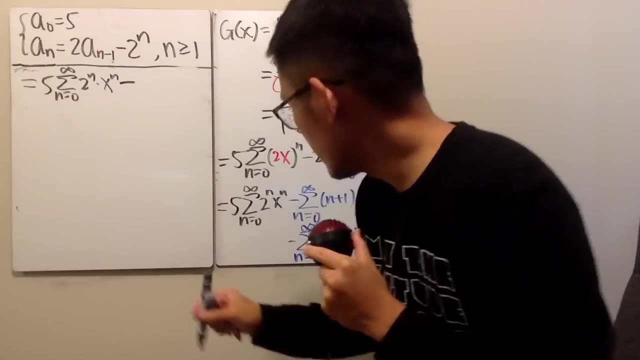 times x to the n. right now, right here, I will have to minus. right, this was a minus, so let me just put on the minus here. and then here we have, the sum n goes from: 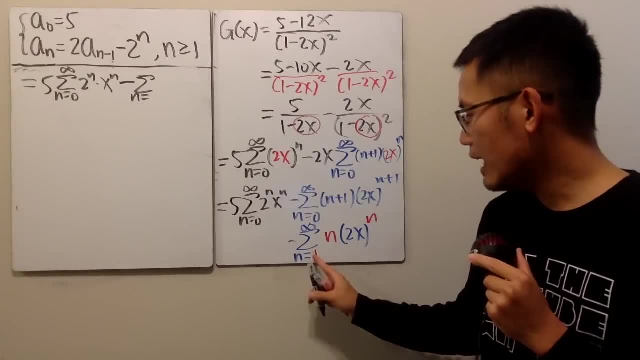 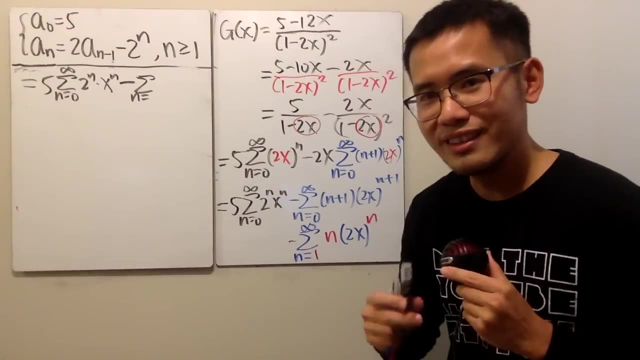 one to infinity. but if you have n goes from one. okay, that's good. if you want to combine, you need to have n is going from zero. can I legitimately change this to n start with zero? 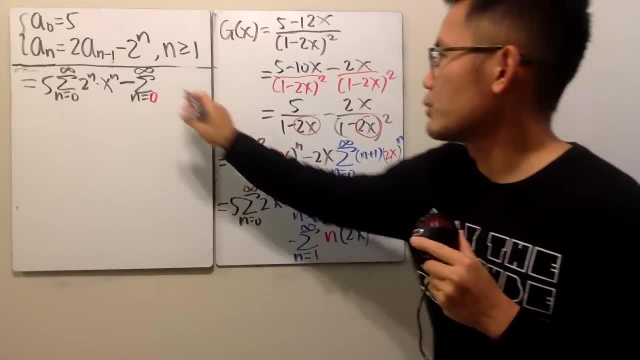 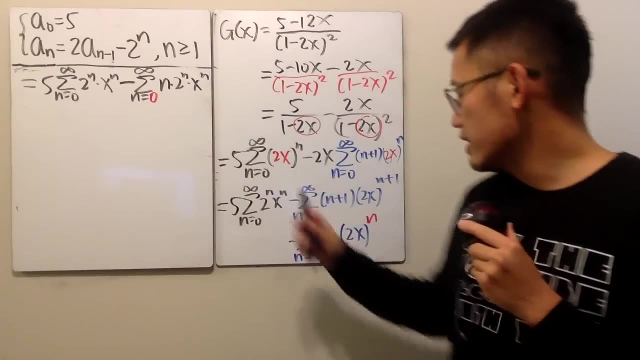 and then to infinity. and then I'll copy it on the rest: n times perhaps already. yes, two to the n times, x to the n. is this the same as that? yes, why? because 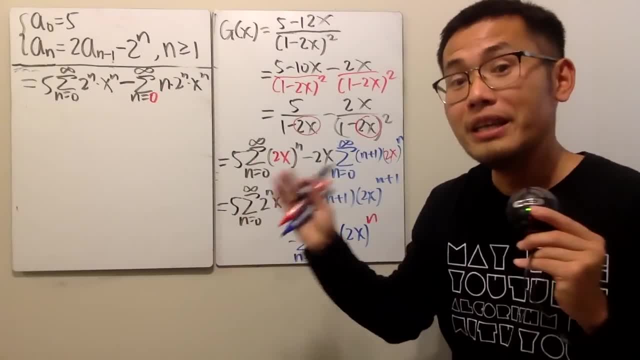 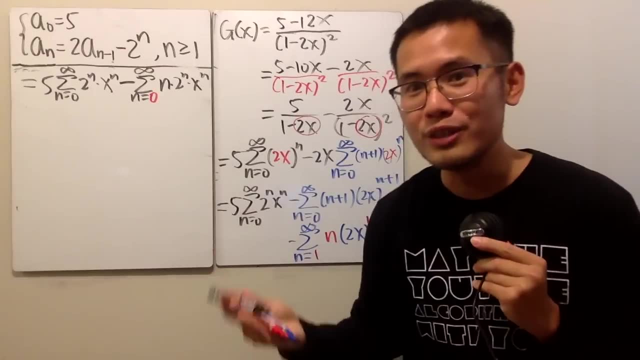 when you have n is equal to zero. you put it here: that's just zero. it does not matter. so this right here, you can just change that to zero. and now you see, the summations are both going from. 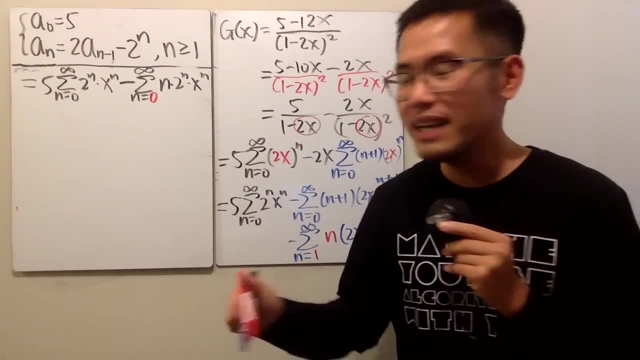 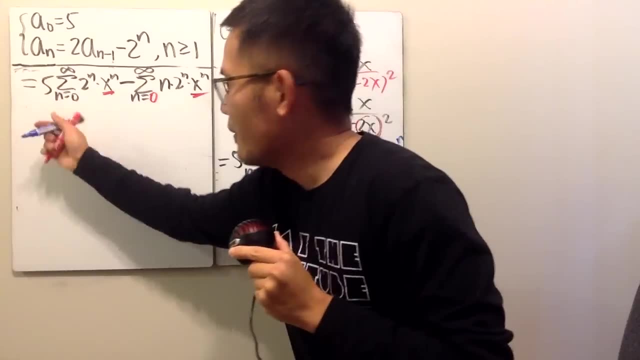 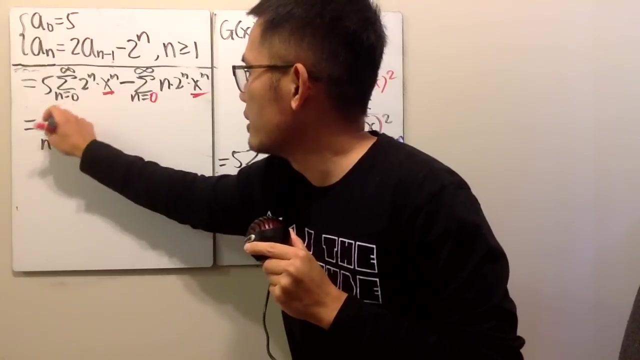 zero to infinity, which is very, very nice and better. yet both of them have x to the n's power. oh my goodness, oh my goodness, now, finally, finally, finally. I'm just going to write this down. 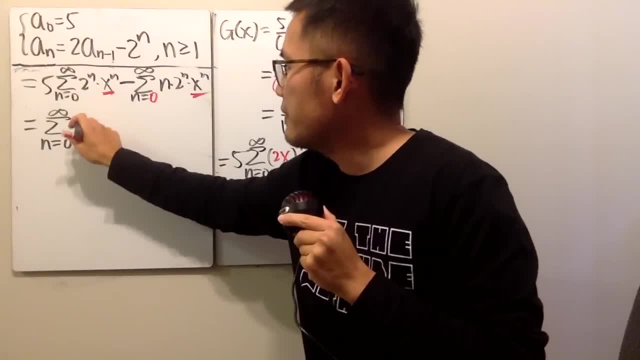 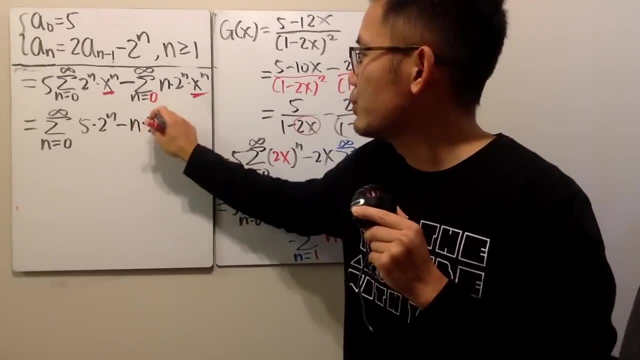 right here for you guys. here we have the sum. I will combine both of them together into just one. well, inside here we have five times two to the n. both of them have that x to the n's power.